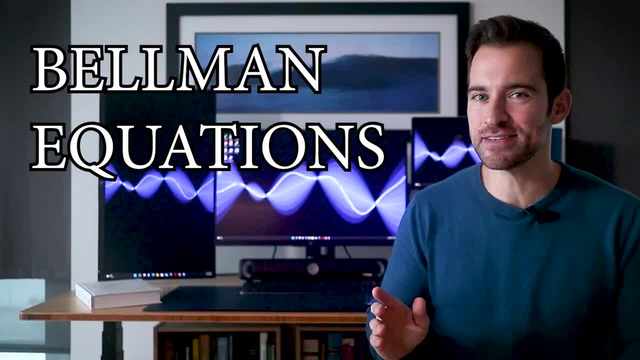 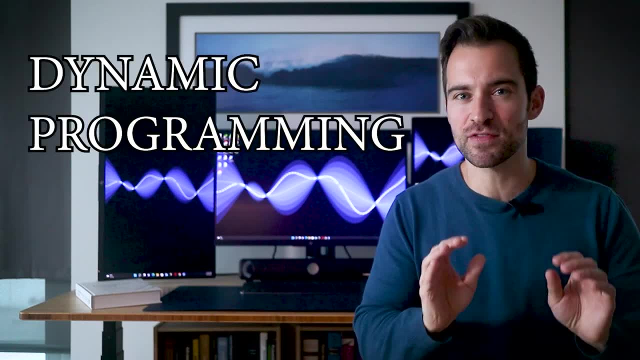 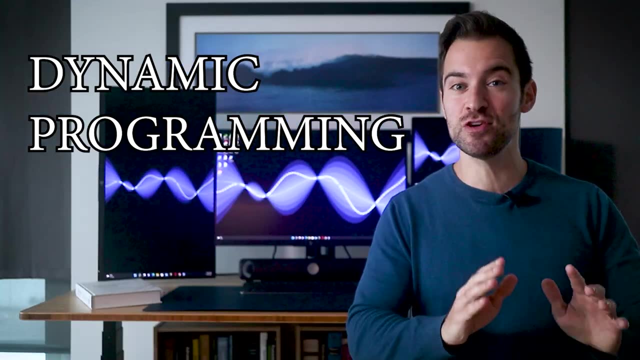 environment into improvements in the agent's behavior. Obviously that's important, And on our path to learning this, we'll also cover dynamic programming, whereby we assume perfect knowledge of the environment's dynamics and can therefore discover optimal policies, policies that are better than all other policies, Considering the huge space of potential policies for any given 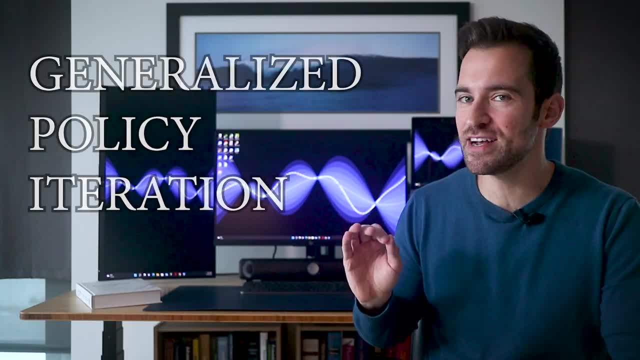 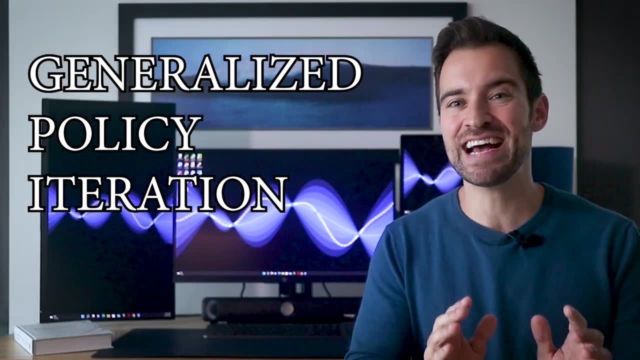 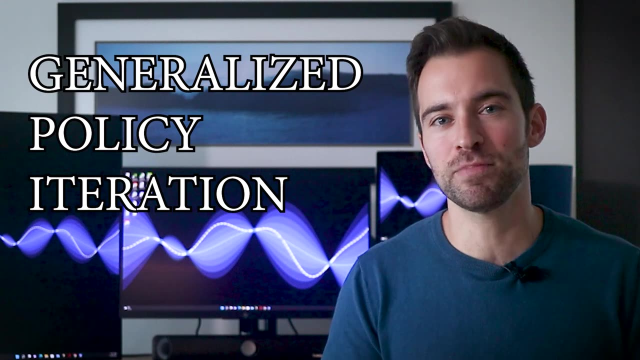 problem. this is quite powerful theory. We'll also learn about generalized policy iteration, which is a kind of solution template used by a huge number of RL methods. We'll see that it casts the component operations of RL algorithms as both competing and cooperating forces that together yield strong policies. For me personally, this angle on the subject 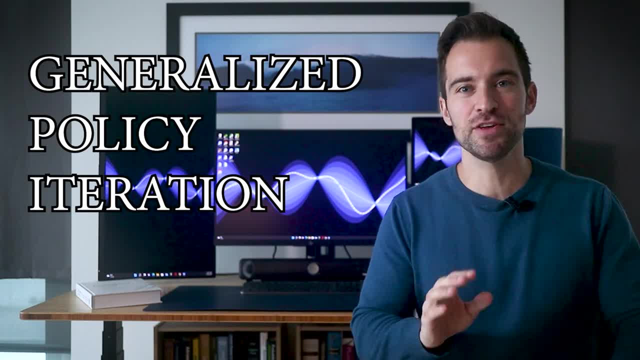 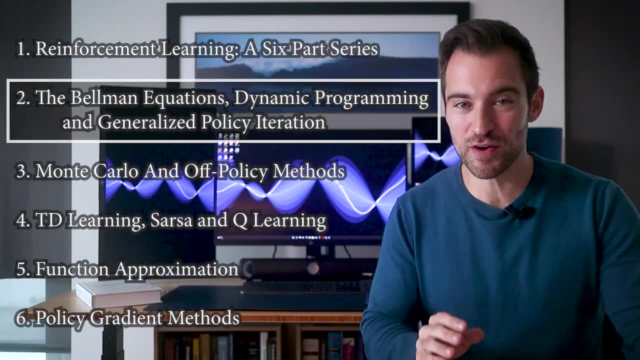 makes everything seem a bit simpler, And if I do my job, you'll soon feel the same way. If you'd like to understand reinforcement learning, these are must-know topics. In fact, this is part two of my six-part series on RL fundamentals. 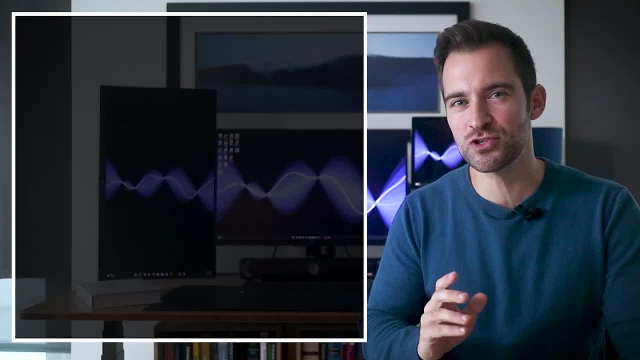 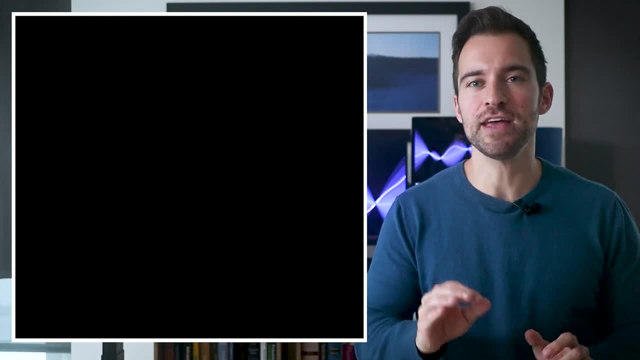 So enough with the selling, Let's get into it. We'll start with a short review, which you can skip with the time codes if you've seen the previous video. Okay, we cast quite generally our problem with a finite Markov decision process, or MDP. We 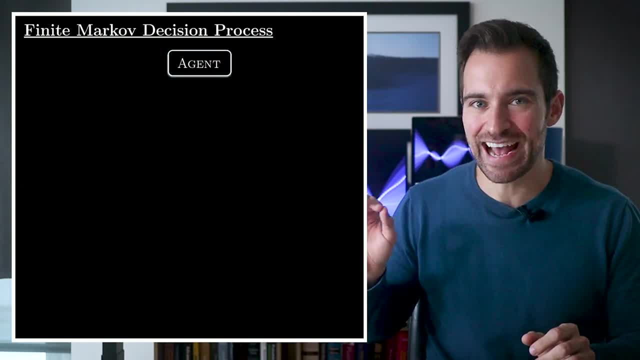 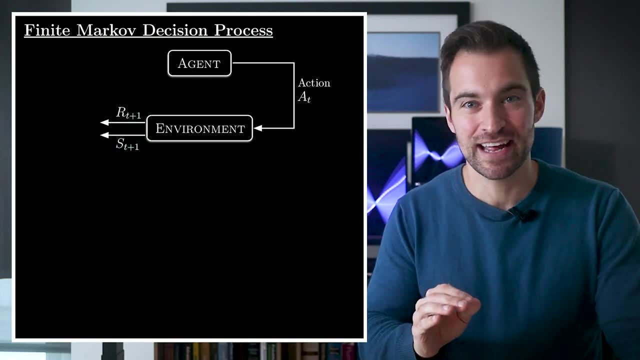 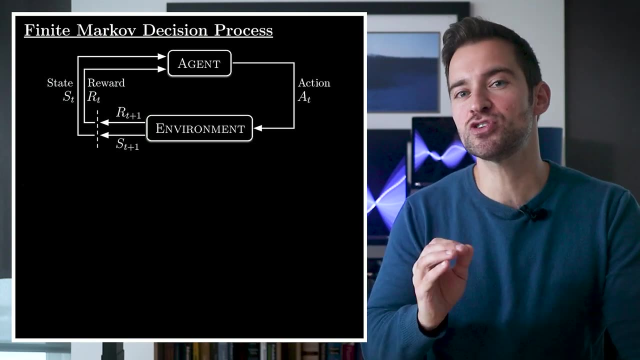 can think of it as a process whereby an agent takes actions that are passed to an environment, which then produces a reward and the next state. These are then passed back to the agent and the process repeats. In the episodic case, it repeats until some terminal state is reached. 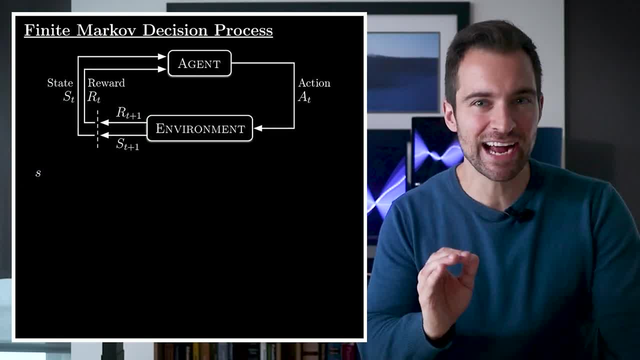 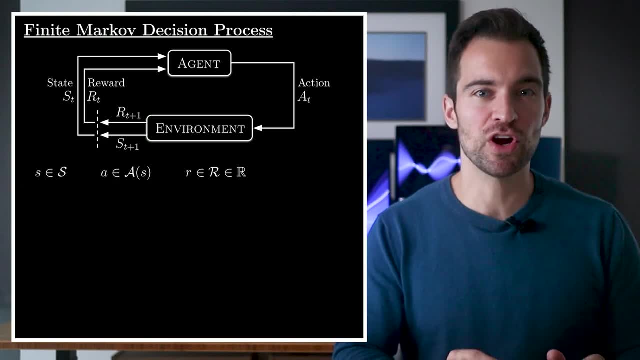 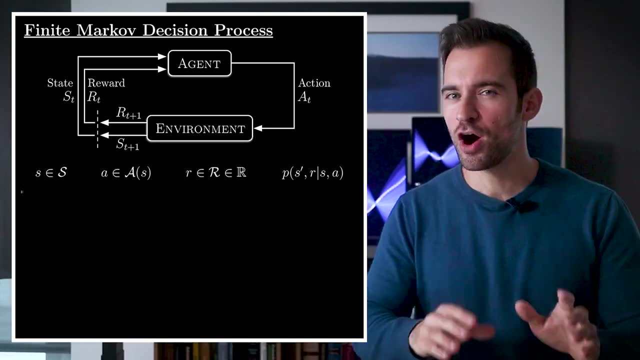 marking the end of an episode. The possible state, action and reward values are restricted to problem-specific finite sets. The dynamics of the environment are given with a probability function which provides the probability of the next state and reward, given the current state and action. 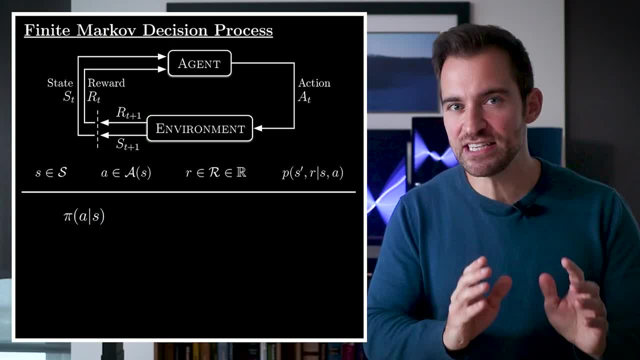 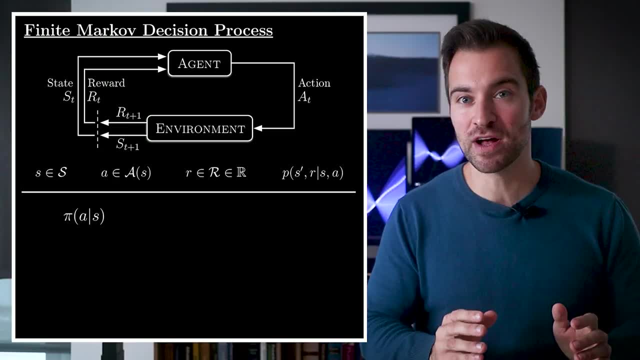 Our goal is to determine a policy which is a state-dependent distribution over actions. The agent selects actions by sampling from this distribution. If we run an agent's policy through the MDP, we'll get a trajectory of states, actions and rewards. 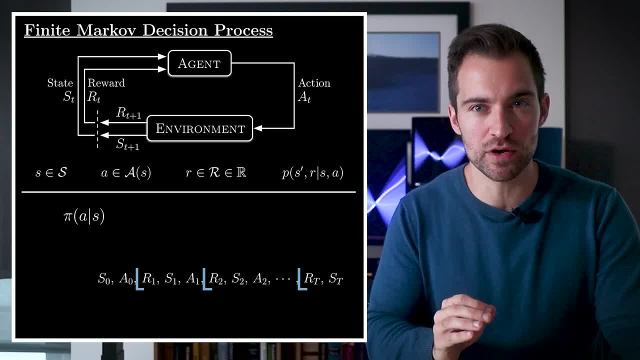 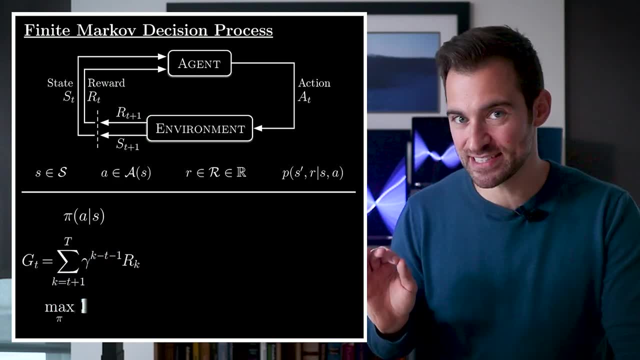 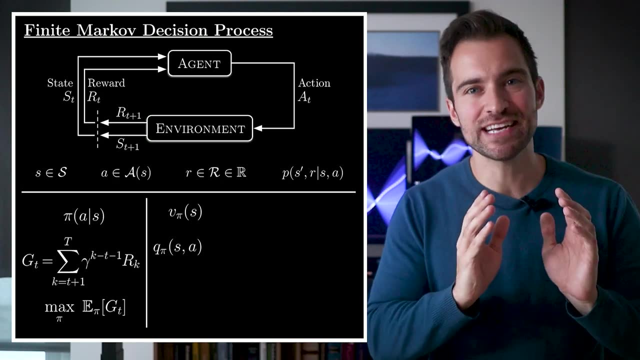 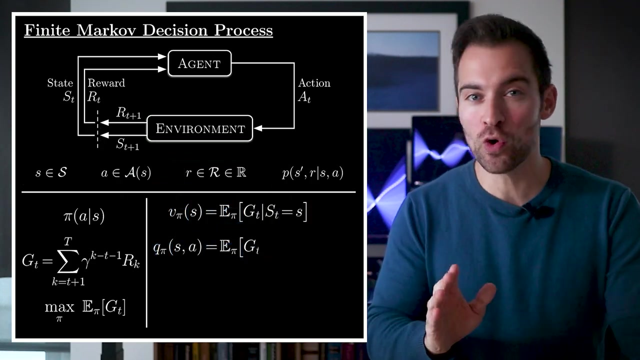 Our goal is to obtain a high discounted sum of future rewards, averaged over many trajectories. One such sum is written as GT, which means our goal is this: Now to make progress. we consider state-value functions and action-value functions which give us the expected value of GT, assuming the agent follows the policy pi and is at a given state or state-action pair. 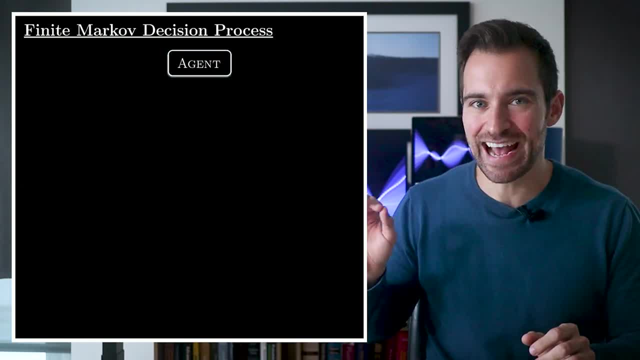 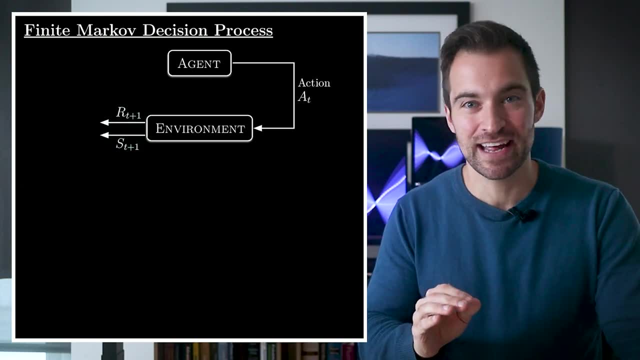 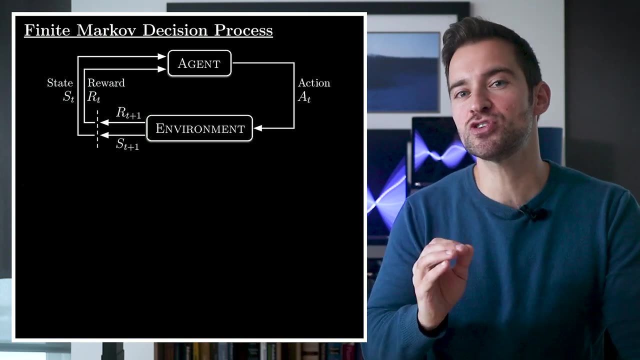 can think of it as a process whereby an agent takes actions that are passed to an environment, which then produces a reward and the next state. These are then passed back to the agent and the process repeats. In the episodic case, it repeats until some terminal state is reached. 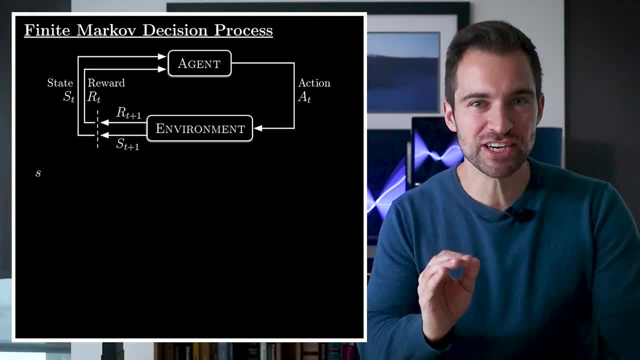 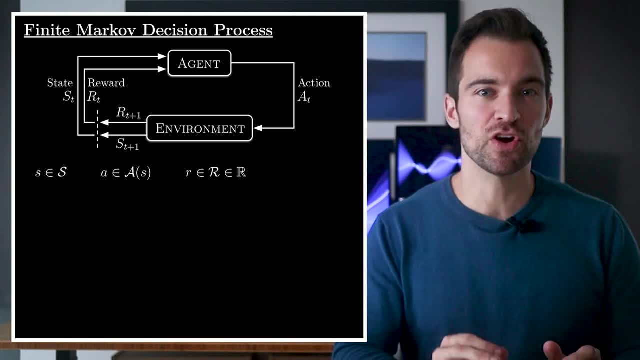 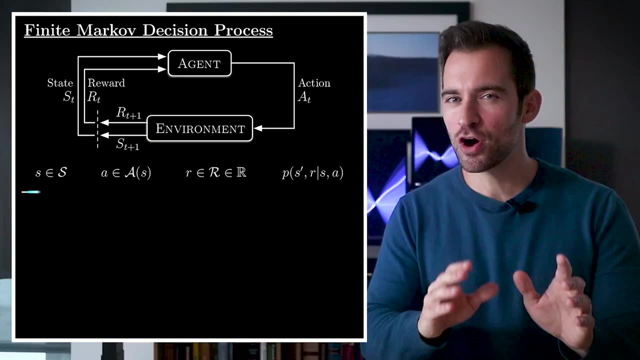 marking the end of an episode. The possible state, action and reward values are restricted to problem-specific finite sets. The dynamics of the environment are given with a probability function which provides the probability of the next state and reward given the current state and action. The probability of the next state and reward given the current state and action. Our goal: 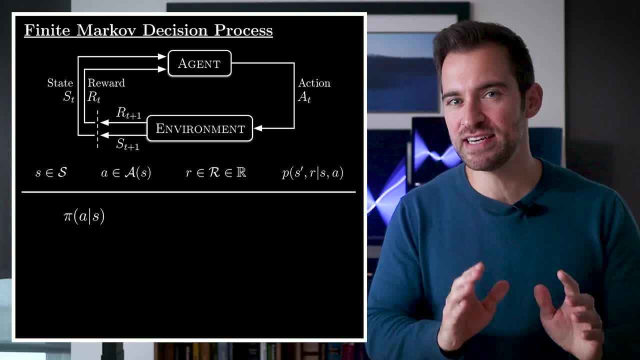 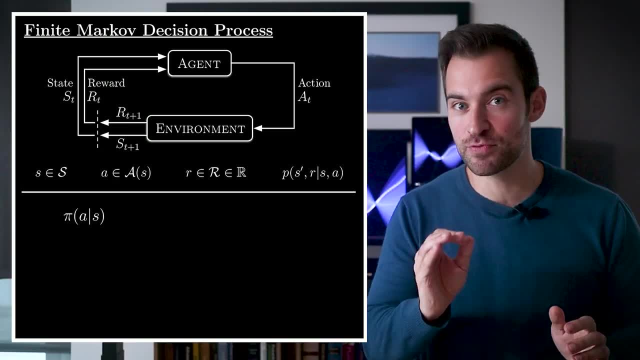 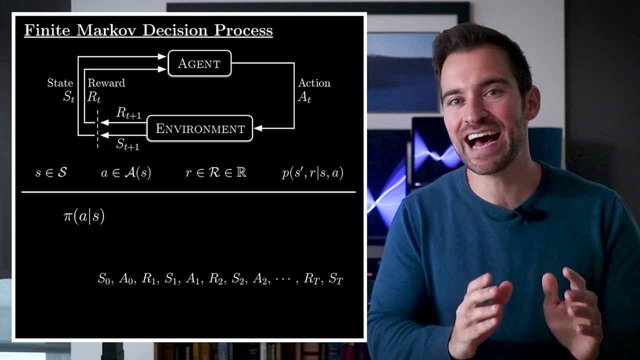 is to determine a policy, which is a state-dependent distribution over actions. The agent selects actions by sampling from this distribution. If we run an agent's policy through the MDP, we'll get a trajectory of states, actions and rewards. Our goal is to obtain a high 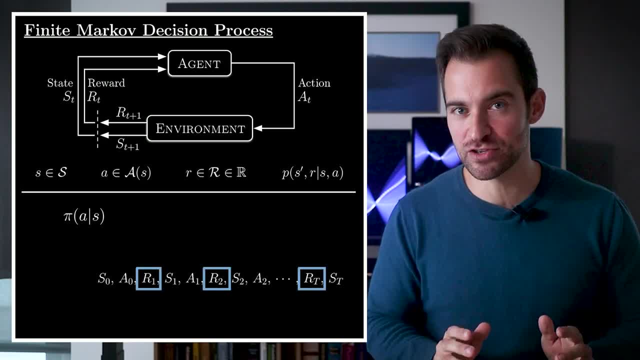 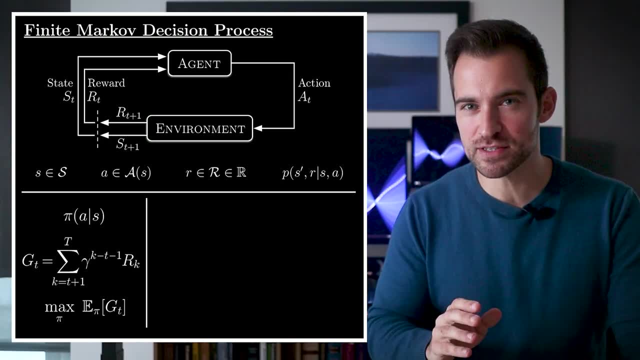 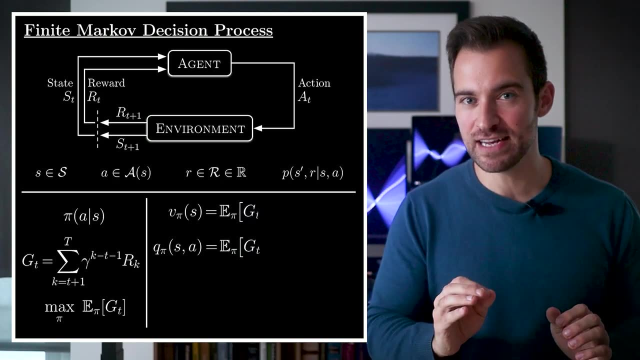 discounted sum of future rewards averaged over many trajectories. One such sum is written as GT, which means our goal is this: Now to make progress. we consider state value functions and action value functions which give us the expected value of GT, assuming the agent. 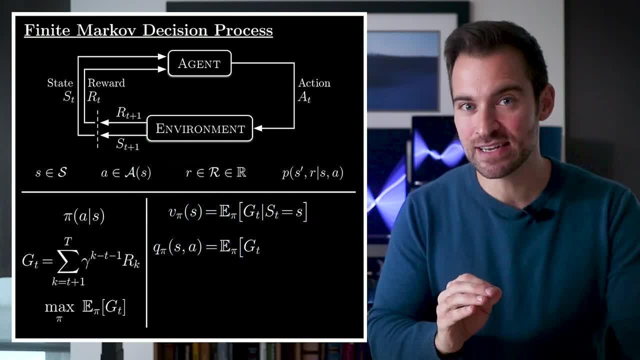 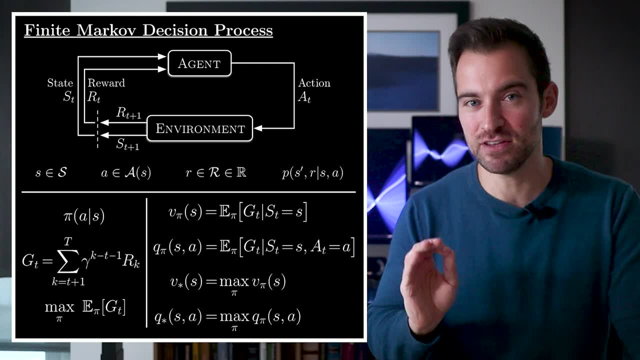 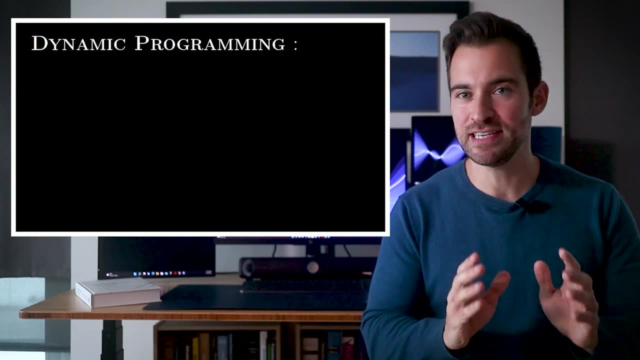 follows the policy pi and is at a given state or state-action pair. We learned previously: we can find the optimal policy if we can find the optimum of these functions. Okay, end of review. Now we can mention something new: dynamic programming. In our context, DP refers to 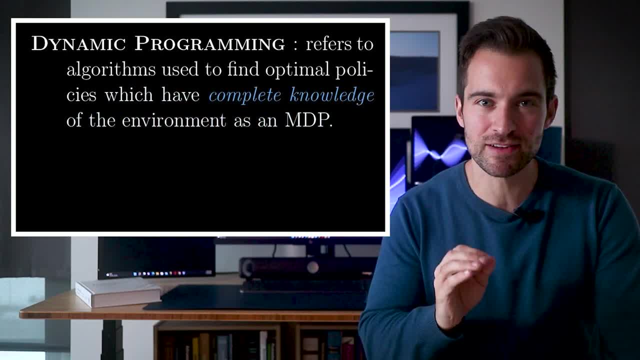 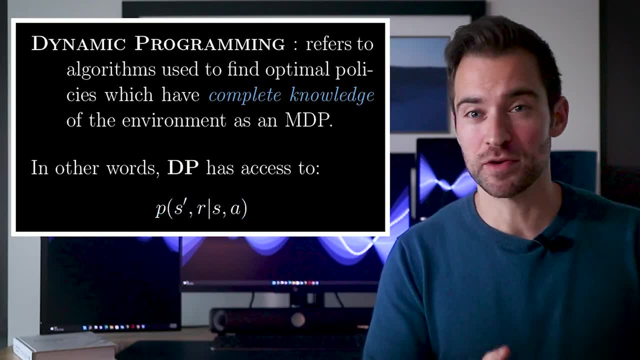 algorithms used to find optimal policies when we have complete knowledge of the environment, In other words, we have exact access to this, which is an unrealistic assumption in the real world. But for now, it gives us a lot of strength. Now to exploit this, we'll use an absolutely 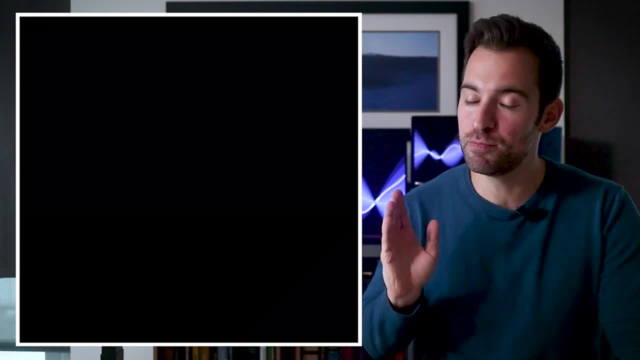 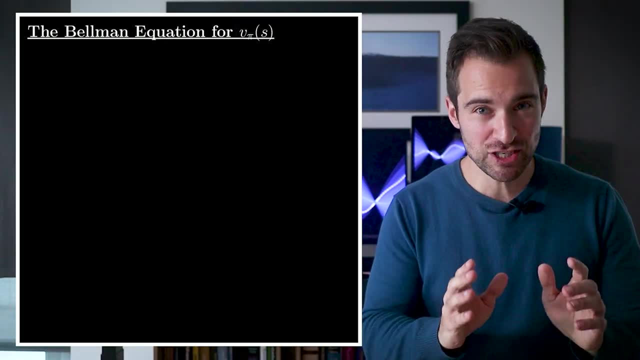 universal concept in the world of sequential decision making: the Bellman equation. There are actually a few of them. We'll start with the one for the value function. Now, before I show you this, I should warn you this panel is mostly algebra. It's not complicated. 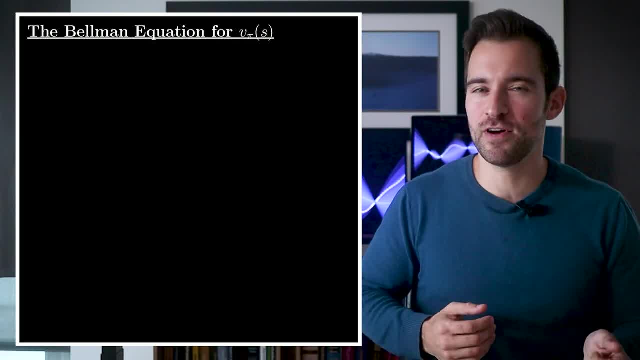 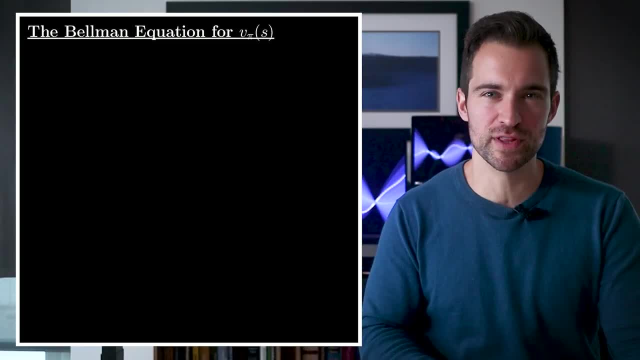 but it's a little boring. Now, as a YouTube educator, I'm supposed to make this fun, cool and exciting. Well, algebra is none of those, but you gotta know some of it if you wanna know RL. Okay, let's motivate this with an example. Let's say we have these states which we can label. 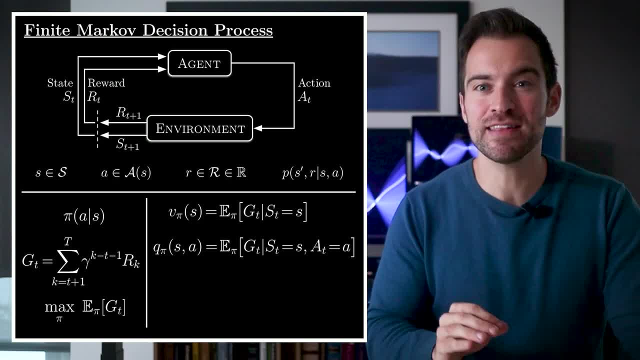 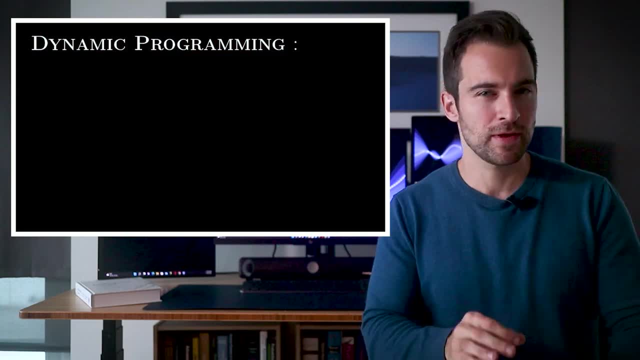 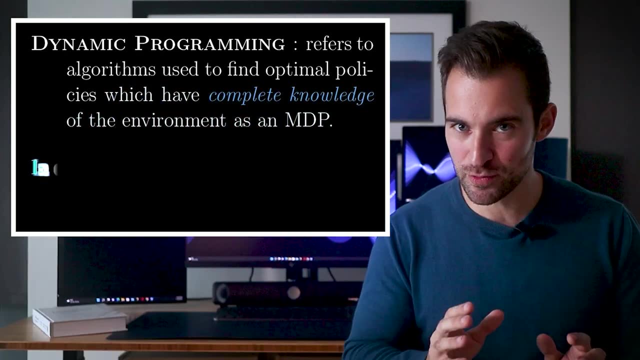 We learned previously, we can find the optimal policy if we can find the optimum of these functions. Okay, end of review. Now we can mention something new: dynamic programming. In our context, DP refers to algorithms used to find optimal policies When we have complete knowledge of the environment, in other words, we have exact access to this. 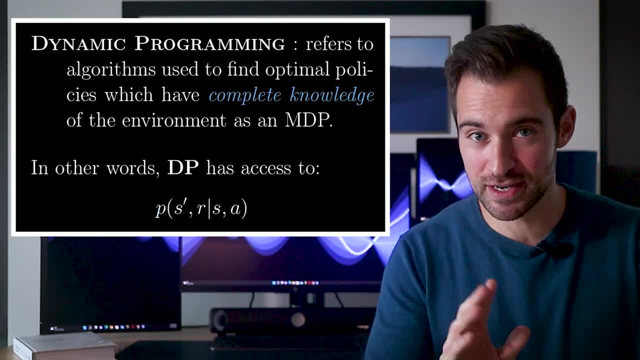 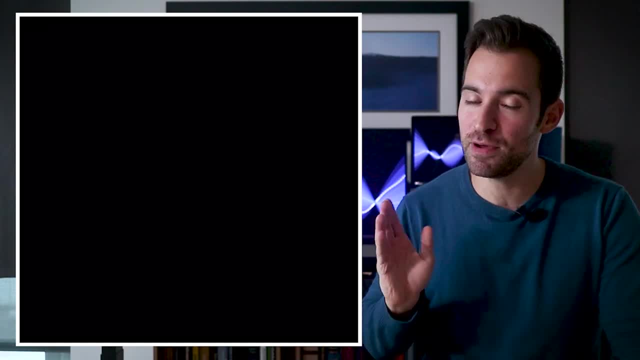 which is an unrealistic assumption in the real world. But for now it gives us a lot of strength. Now to exploit this, we'll use an absolutely universal concept in the world of sequential decision-making: the Bellman equation. There are actually a few of them. We'll start with the one for the value function. 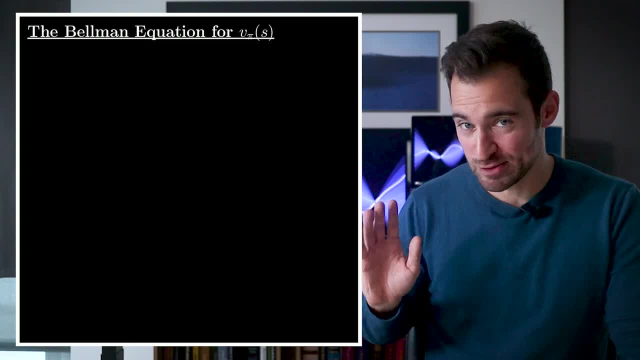 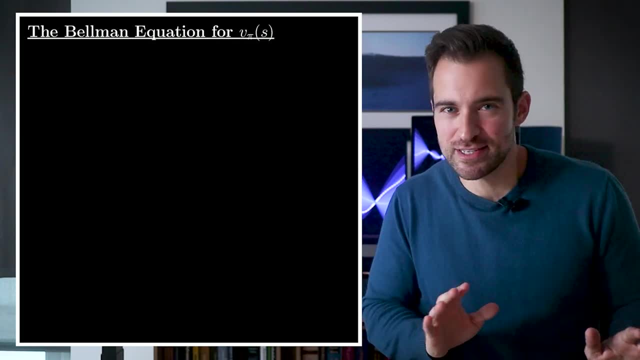 Now, before I show you this, I should warn you: this panel is mostly algebra. It's not complicated, but it's a little boring. Okay, As a YouTube educator, I'm supposed to make this fun, cool and exciting. Well, algebra is none of those, but you got to know some of it if you want to know RL. 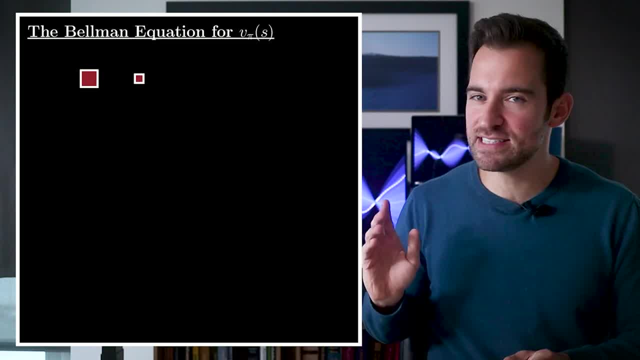 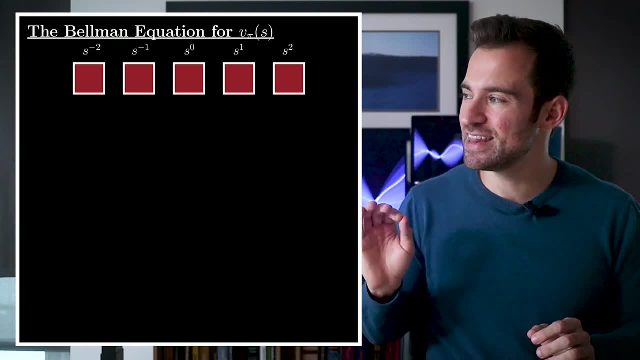 Okay, let's motivate this with an example. Let's say we have these states which we can label like this. Now, instead of describing the whole MDP, I'm going to focus on this state S0, and tell you from this state the agent can pick left or right. 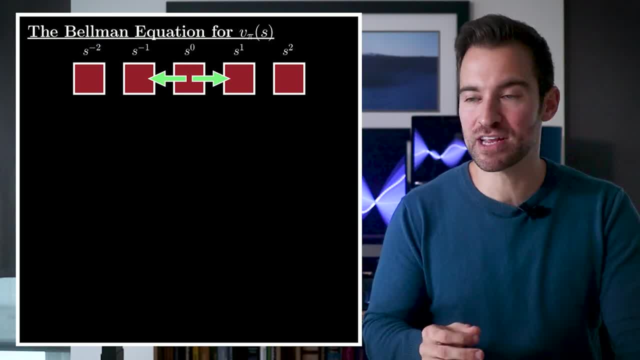 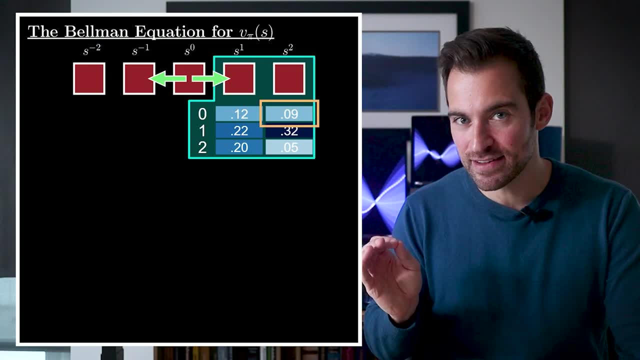 If the agent selects right, the reward and next state probabilities are given by this state. For example, if the agent selects right, this cell tells us there is a 9% chance the agent will end up at S2 with the reward of 0.. 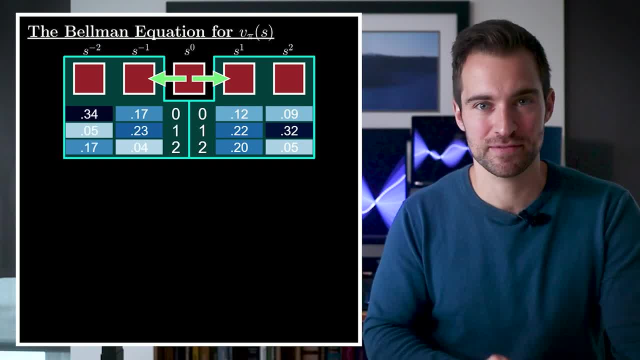 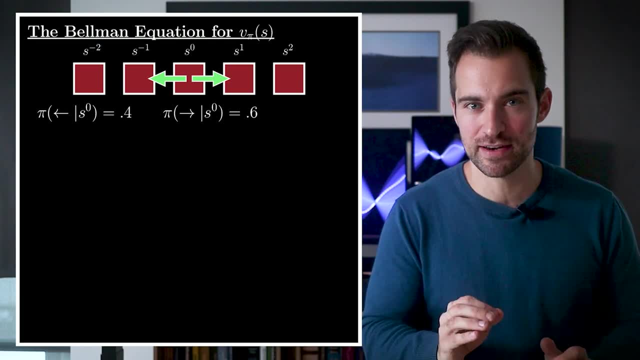 As you'd expect, something similar is true for selecting left. Next, the policy from this state is a 40% chance of choosing left and a 60% chance of choosing right, And the discount factor is 0.95.. Now here's the question. 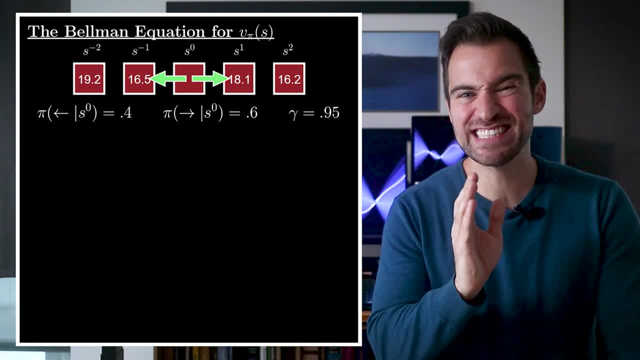 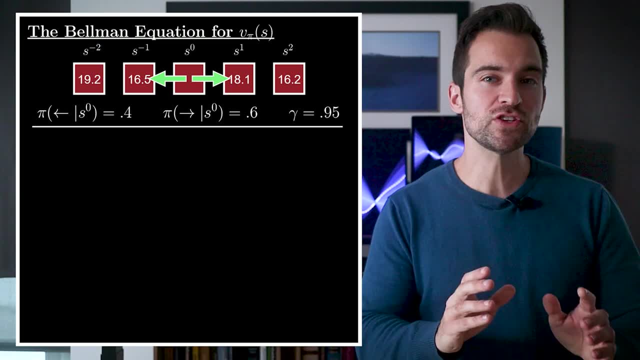 Can you determine the values of the possible next states? Can you determine the state value of S0?? Yes, and it's the Bellman equation that does this. To discover it ourselves, we start with the definition of what we're trying to calculate. 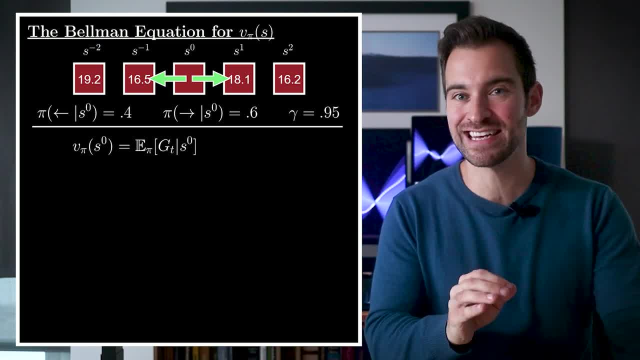 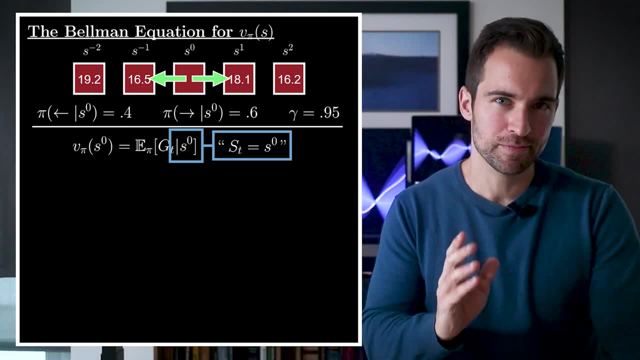 Remember it's the expected return, conditional on the center state S0.. Regarding notation, I'll be using this shorthand to omit the random variable. when it's obvious, Okay, back to it. We break this down by action, meaning it'll be a sum of two terms. 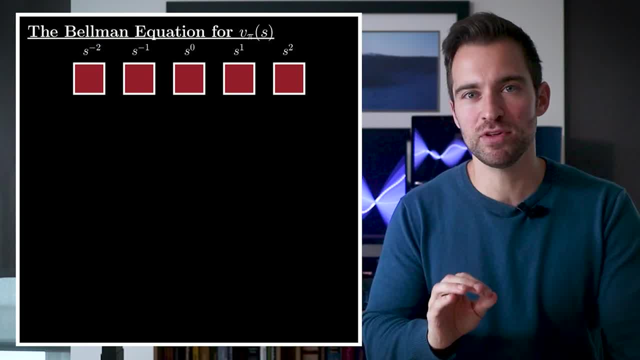 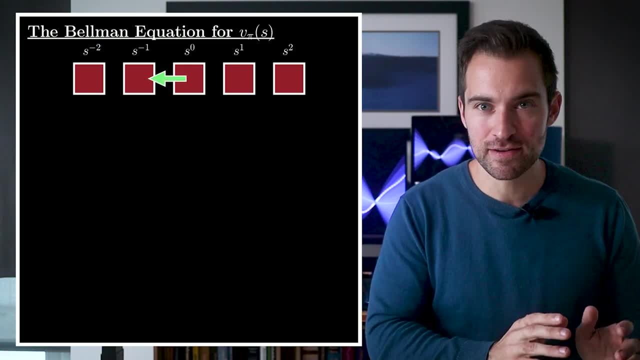 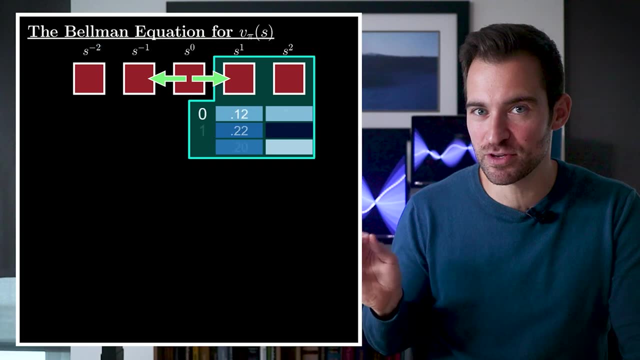 like this. Now, instead of describing the whole MDP, I'm going to focus on this state S0, and tell you from this state the agent can pick left or right. If the agent selects right, the reward and next state probabilities are given by this distribution. For example, 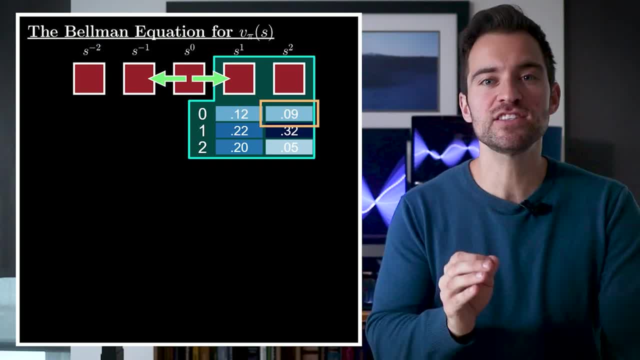 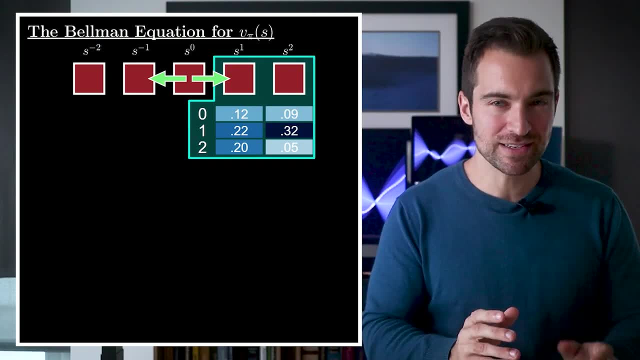 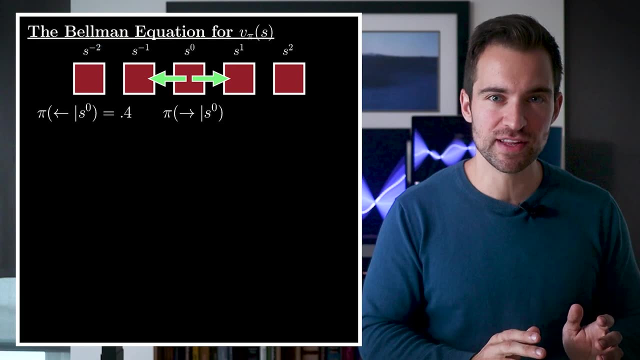 if the agent selects right, this cell tells us there is a 9% chance the agent will end up at S2 with a reward of 0.. As you'd expect, something similar is true for selecting left. Next, the policy from this state is a 40% chance of choosing left and a 60% chance of choosing right. 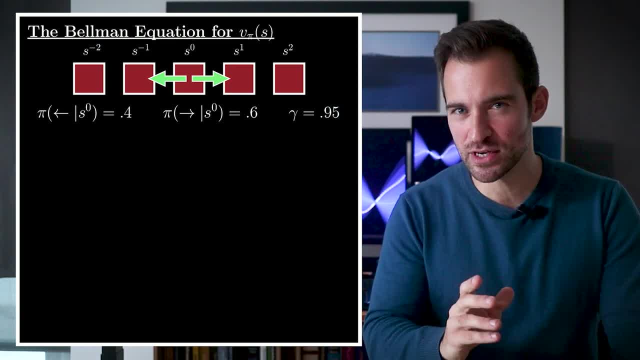 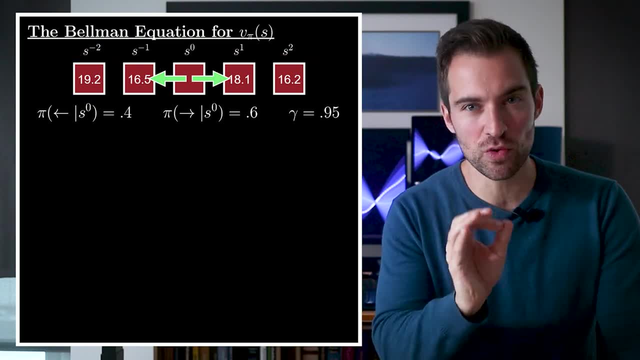 And the discount factor is .95.. Now here's the question: If I also tell you the state values of the possible next states, can you determine which one is correct? Well, if you do that, you can determine the state value of S0.. Yes, and it's the Bellman equation that does this. 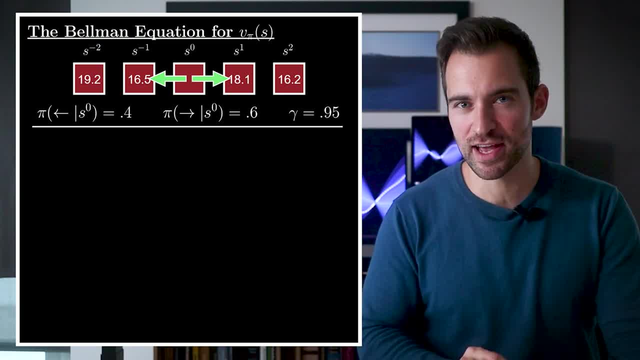 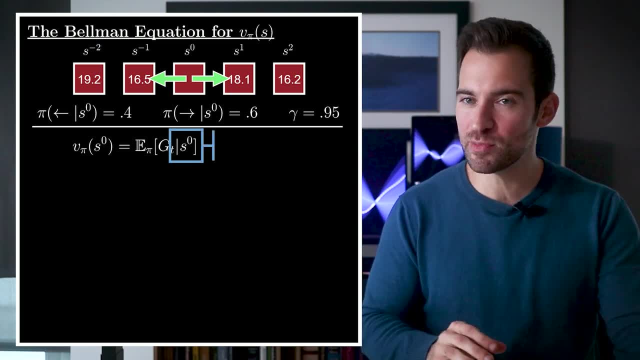 To discover it ourselves. we start with the definition of what we're trying to calculate. Remember, it's the expected return conditional on the center state S0.. Regarding notation, I'll be using this shorthand to omit the random variable when it's obvious. Okay, back to it. 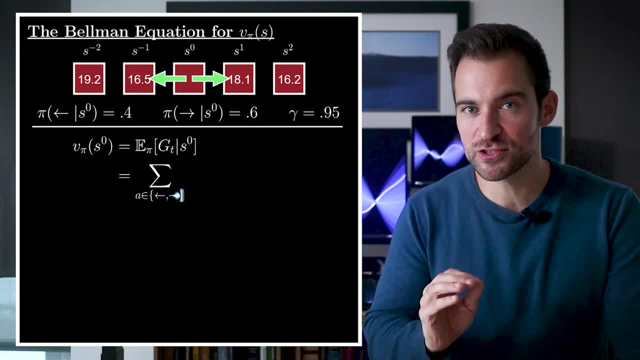 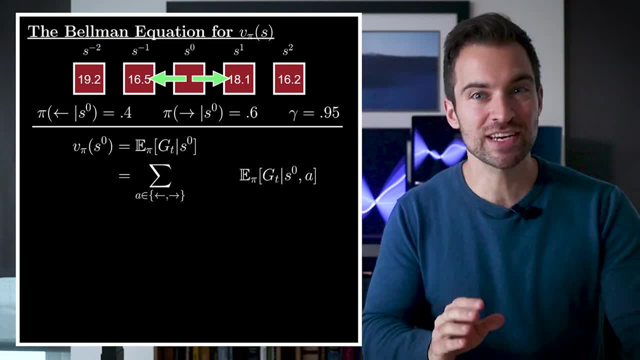 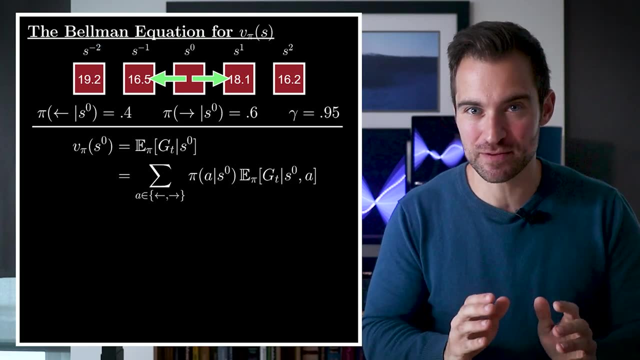 We break this down by action, meaning it'll be a sum of two terms, one for the left action and one for the right action. Each term will be the expected return, conditional on the current state and the action, weighted by the probability of taking each action. If you know your probability, 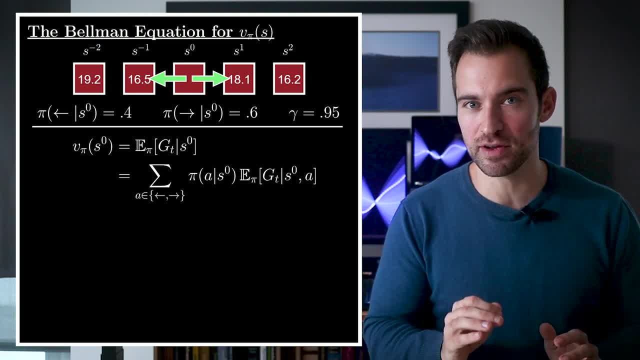 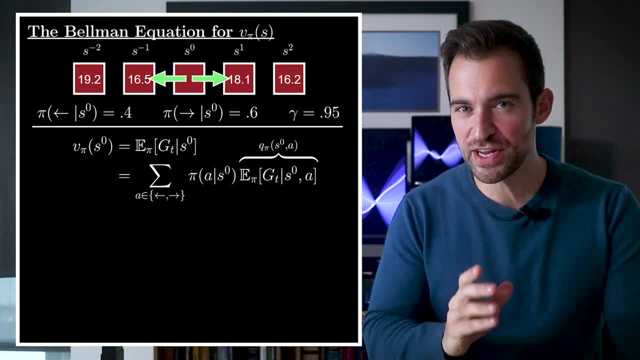 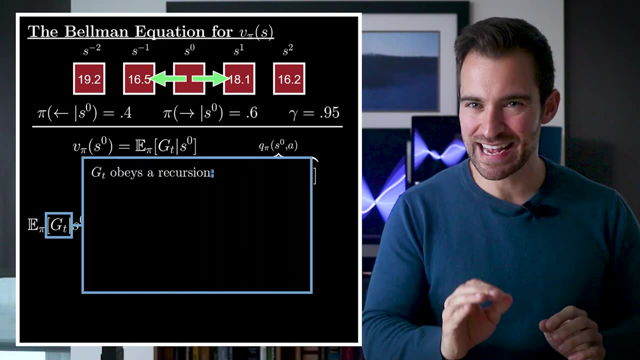 theory, you'll notice this is just an application of the law of total probability. Also, if you're observant, you'll recognize that this term is in fact an action value. Okay, from here let's pick out the go-right expectation and recognize something about GT: It obeys. 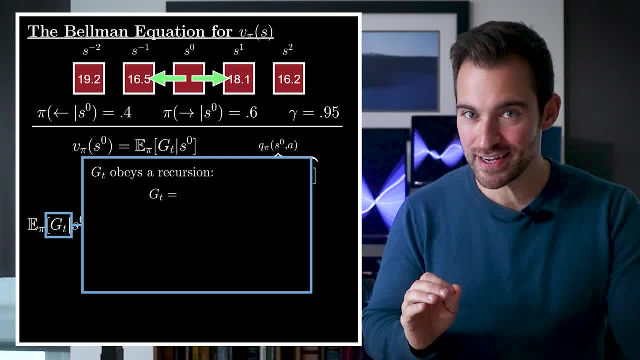 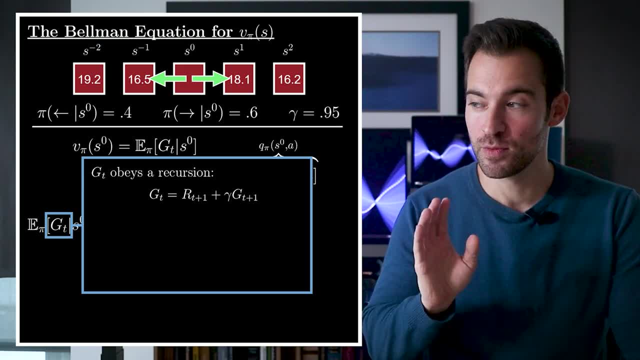 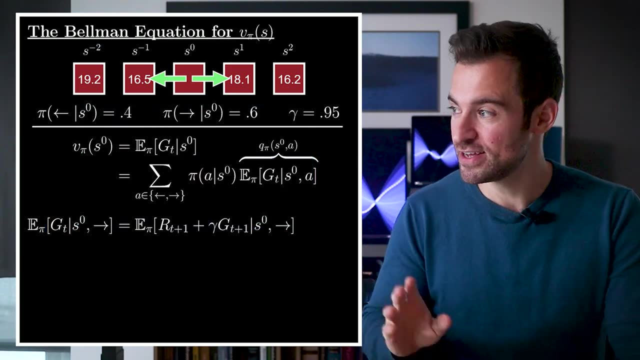 a simple recursive relationship: GT is equal to the reward plus the once-discounted return one step later. With a little algebra that's not too hard to see. And so we can write this And then something sneaky, This: What I've done here is I've replaced GT plus one with what you. 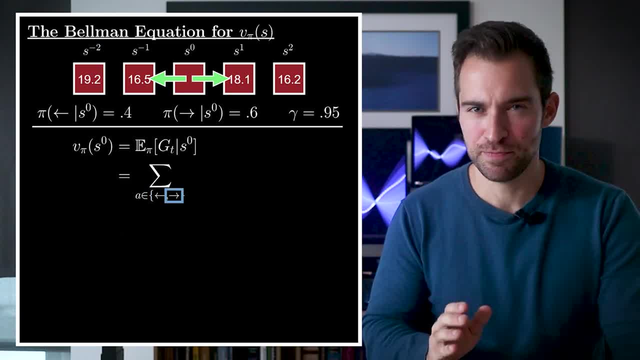 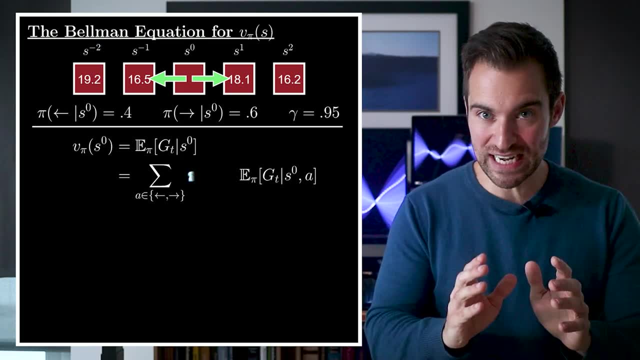 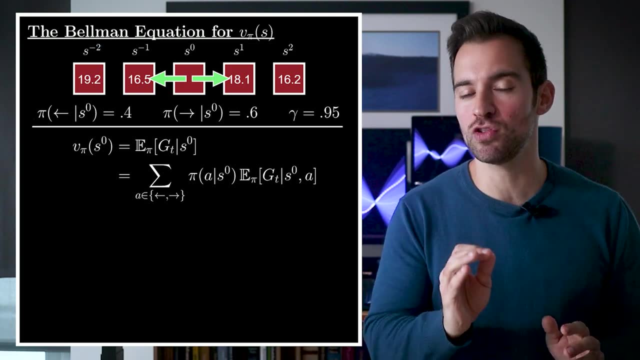 One for the left action and one for the right action. Each term will be the expected return, conditional on the current state and the action, weighted by the probability of taking each action. If you know your probability theory, you'll notice this is just an application of the law of total probability. 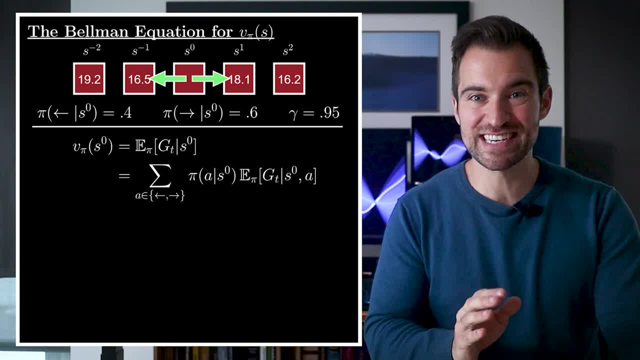 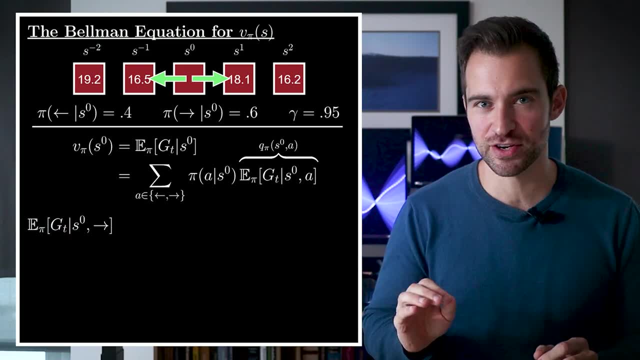 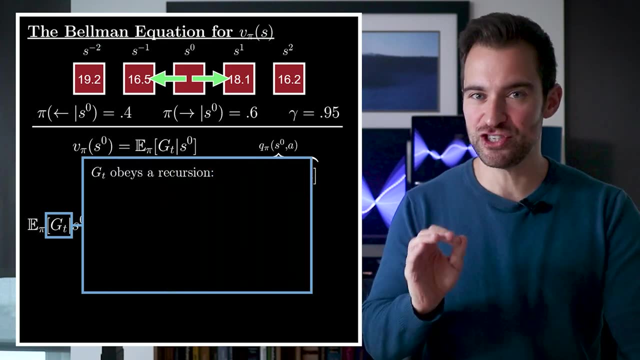 Also, if you're observant, you'll recognize that this term is in fact an action value. Okay, from here, let's pick out the go-right expectation and recognize something else. Let's look at something about gt. It obeys a simple recursive relationship. 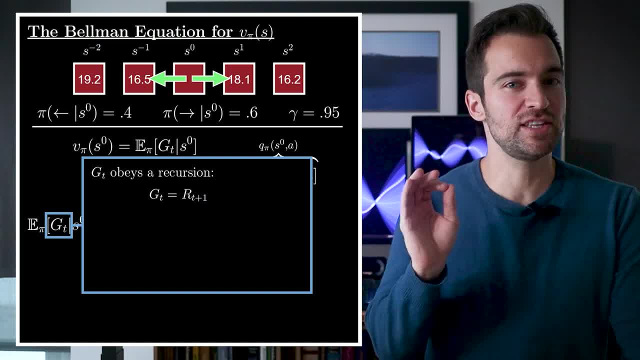 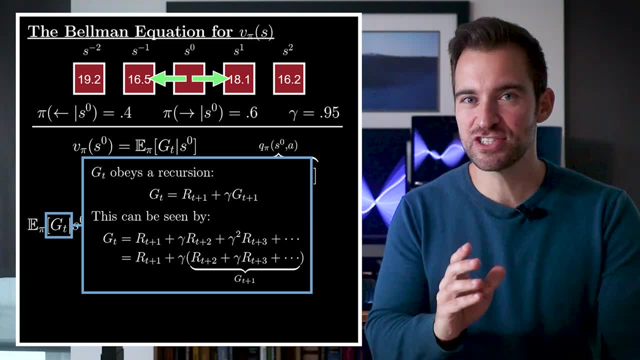 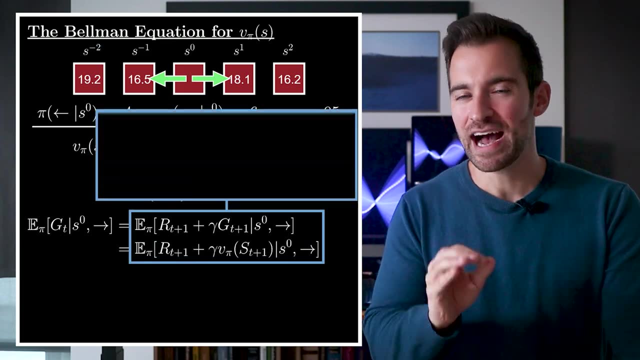 gt is equal to the reward plus the once-discounted return one step later. With a little algebra, that's not too hard to see. And so we can write this And then something sneaky, This: What I've done here is I've replaced gt plus one with what you get when plugging the randomly determined 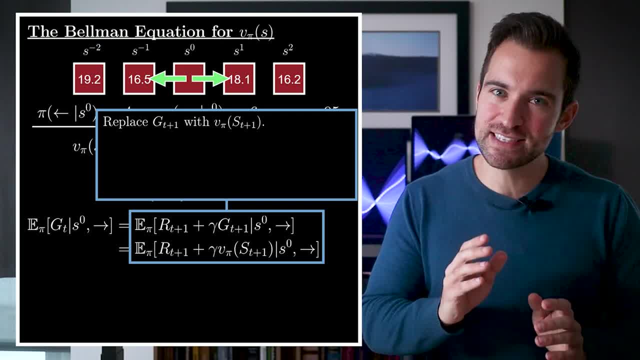 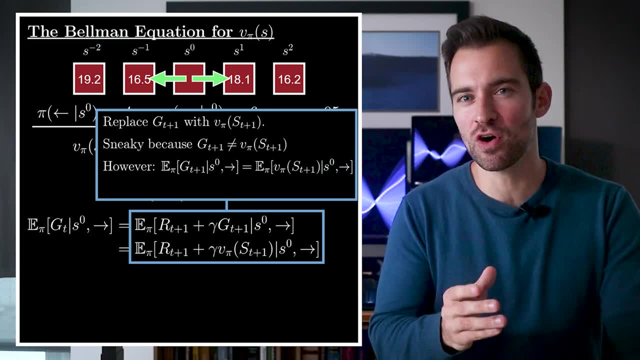 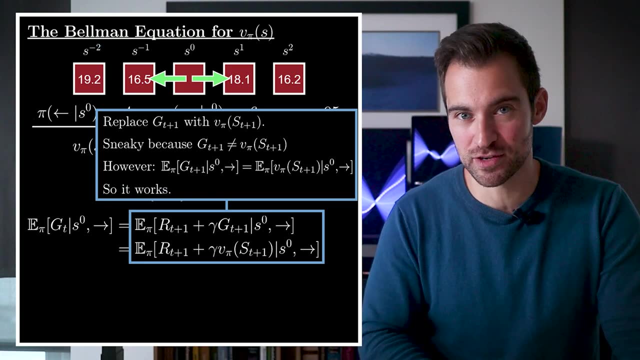 next state into the value function. This is sneaky because they're not equal, However, in expectation they are. This isn't too hard to see if you recall the definition of the state value function and apply the law of total probability. But, more importantly, because it's true, this substitution works. 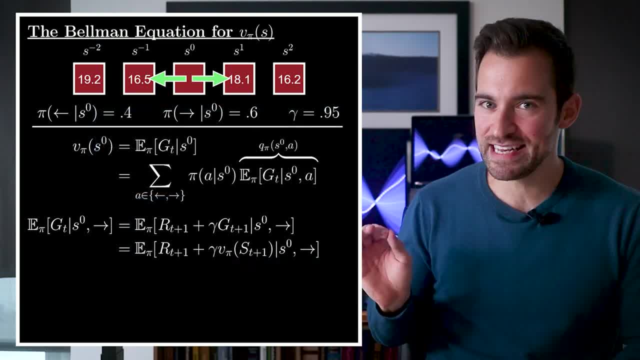 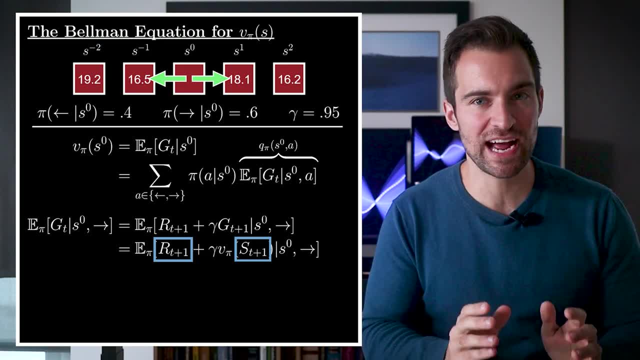 Now, from here it gets easier. We just remember that these are random variables and we're calculating an expectation. By definition, it's just a probability-weighted average of values, And we can find that information in the go-right distribution. 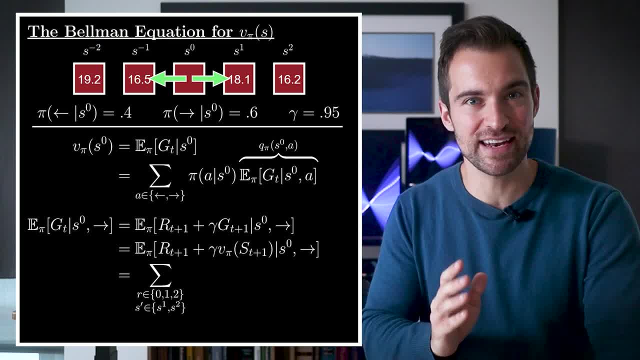 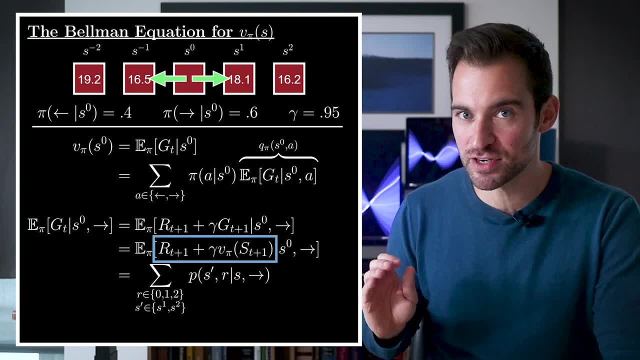 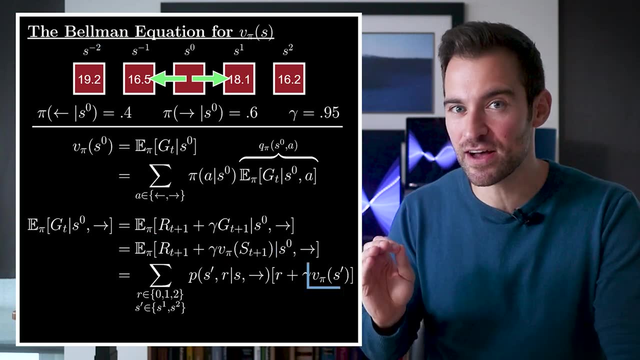 Specifically, this will equal a sum over all pairs of reward and next state. Each term will be weighted by their probability. The terms themselves are just this expression with the values substituted in, which is this: And remember, at the start we were given these values, so we have everything we need to calculate the right action expectation. 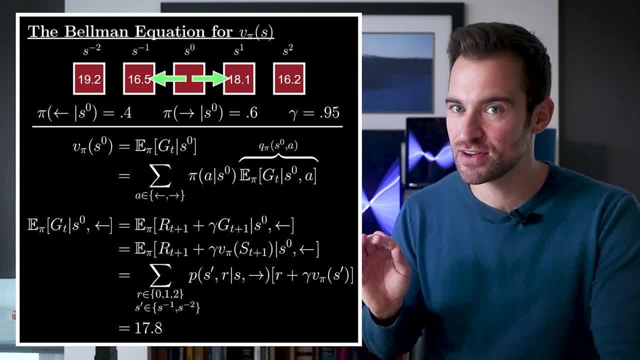 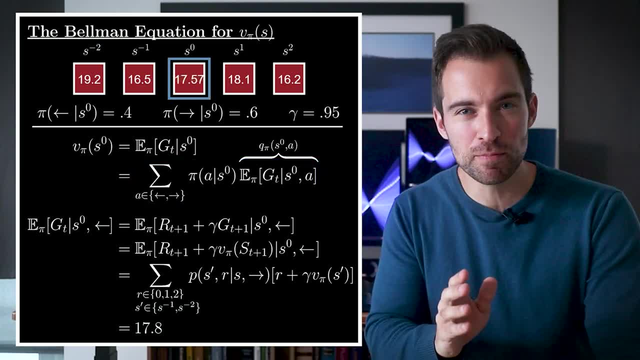 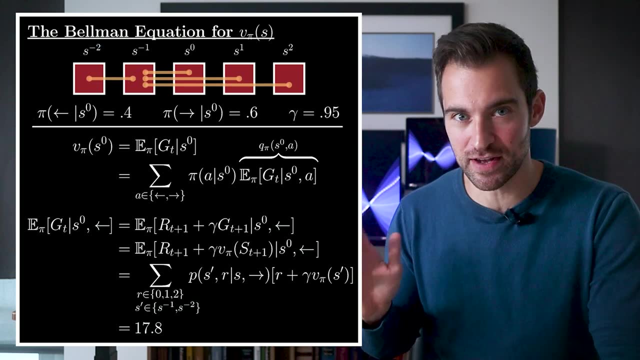 And we can do the exact same thing for the left action. That would give us all numbers for this, which means we have everything to calculate our answer. And this is what the Bellman equation does for us: It connects state values. In fact, it connects all state values. 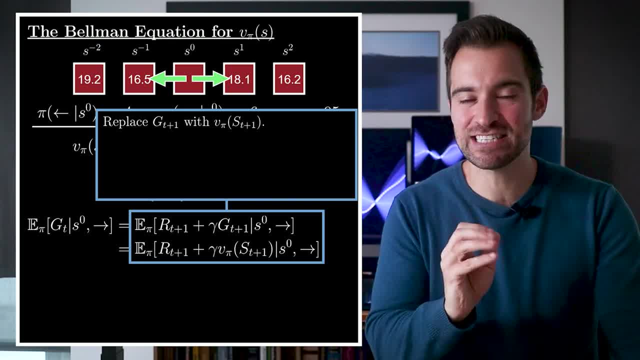 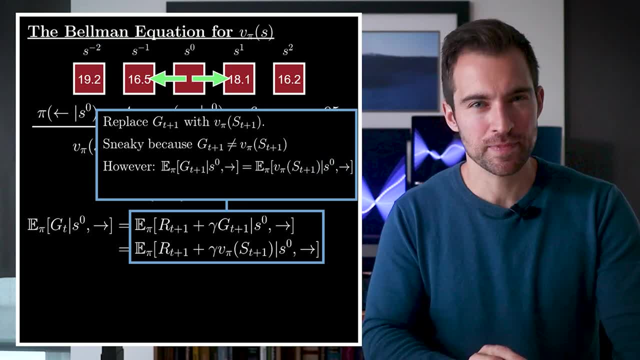 get when plugging the randomly determined next state into the value function. This is sneaky because they're not equal, However, in expectation they are. This isn't too hard to see if you recall the definition of the state value function and apply the law of total probability. 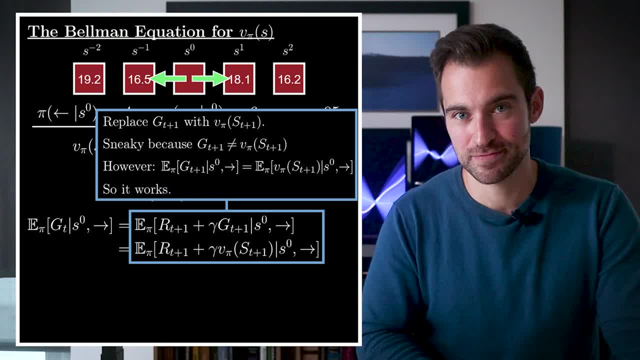 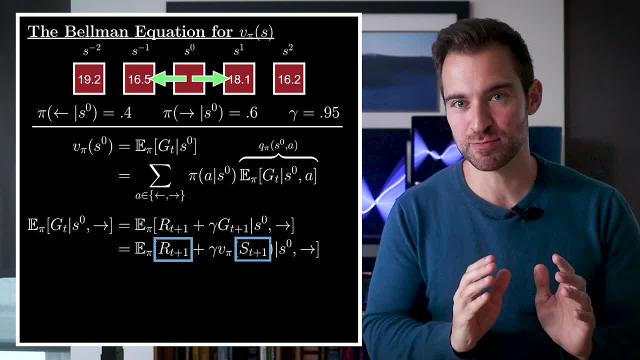 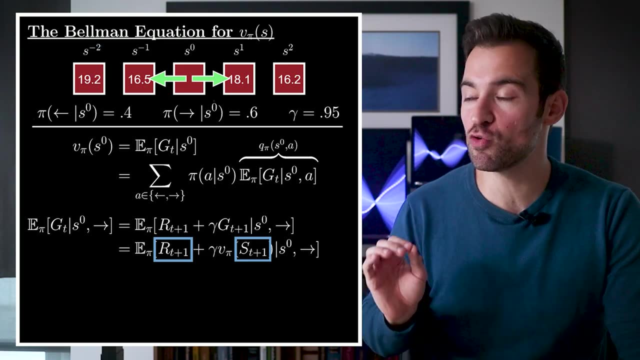 but more importantly, because it's true, this substitution works. Now, from here it gets easier. We just remember that these are random variables and we're calculating an expectation. By definition, it's just a probability-weighted average of values, and we can find that information in the 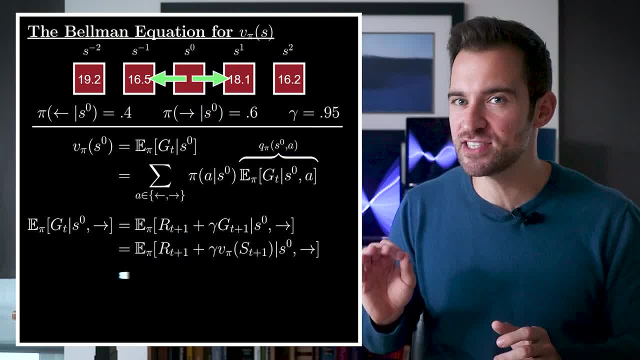 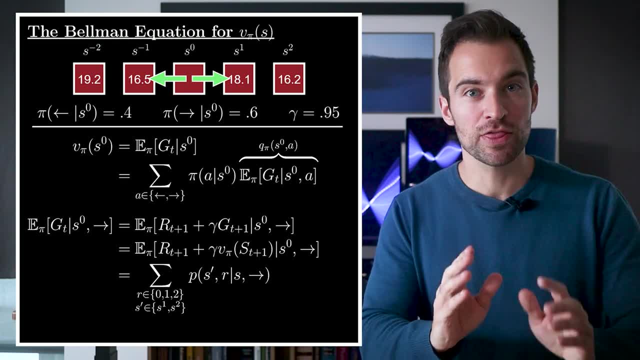 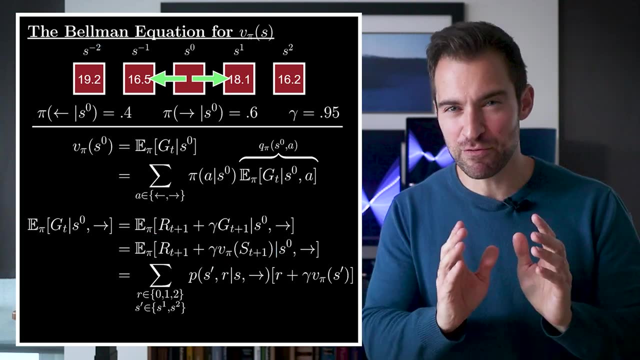 go-right distribution. Specifically, this will equal a sum over all pairs of reward and next state. Each term will be weighted by their probability. The terms themselves are just this expression with the values substituted in which is this: And remember, at the start we were given these values. 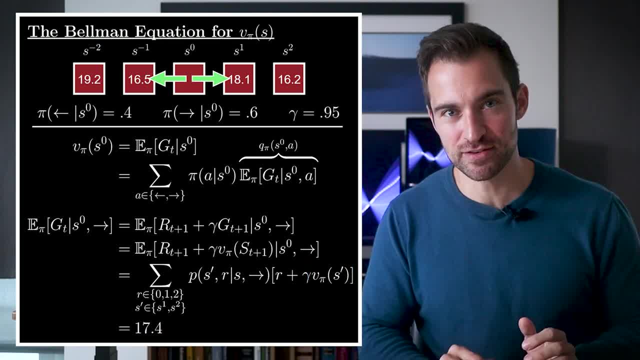 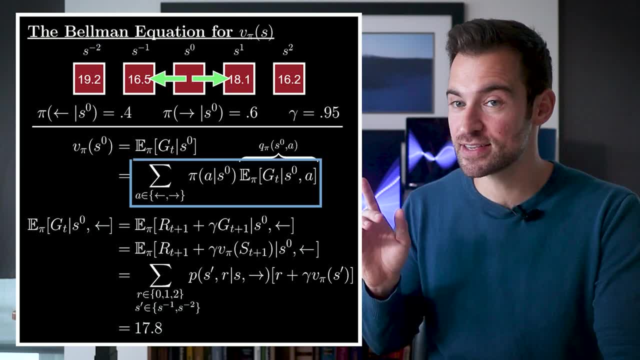 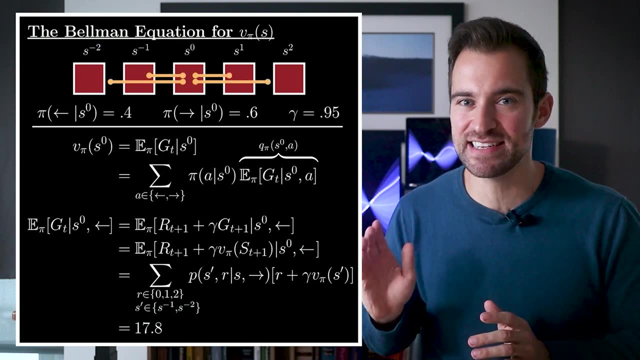 so we have everything we need to calculate the right action expectation, And we can do the exact same thing for the left action. That would give us all numbers for this, which means we have everything to calculate our answer, And this is what the Bellman equation does for us. It connects. 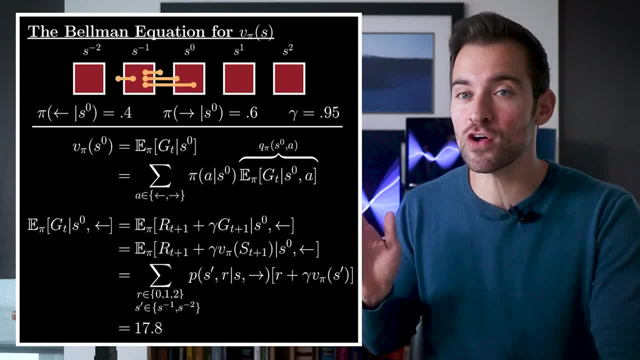 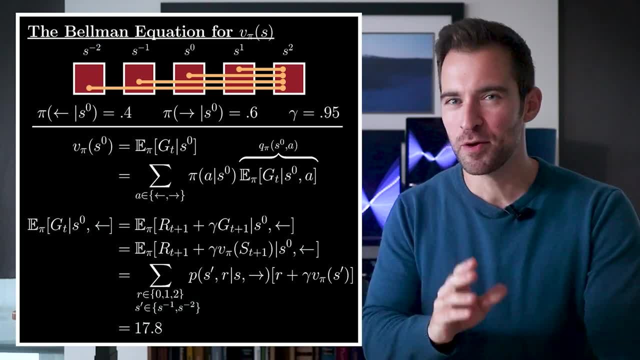 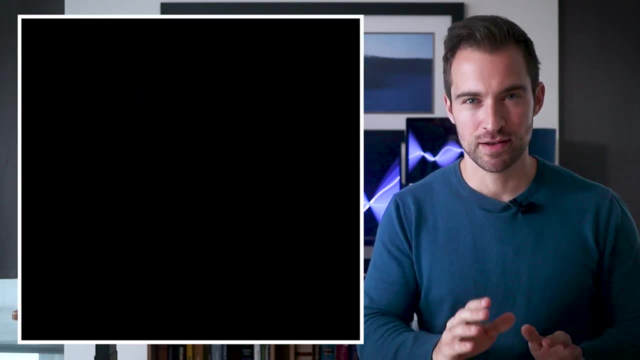 state values. In fact, it connects all state values. This means, if we can solve for some state values, we can solve for others. That's huge, But it's not the whole story. These are connections for any policy. Let's now talk about optimal policies, In particular the Bellman optimality. 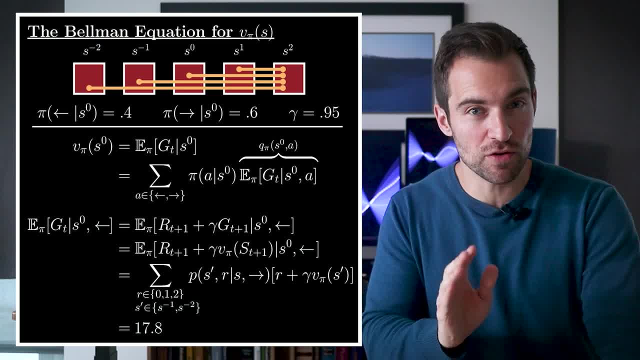 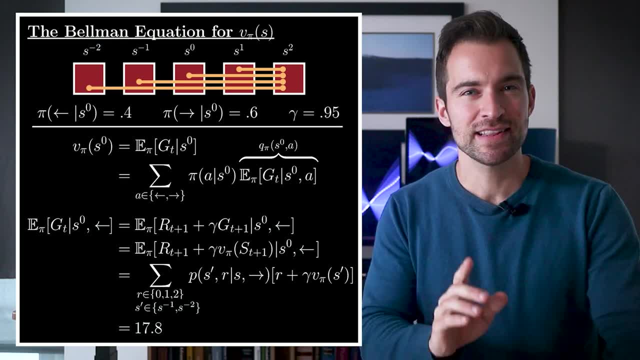 This means if we can solve for some state values, we can solve for others. That's huge, But it's not the whole story. These are connections for any policy. Let's now talk about optimal policies, In particular the Bellman optimality equation. 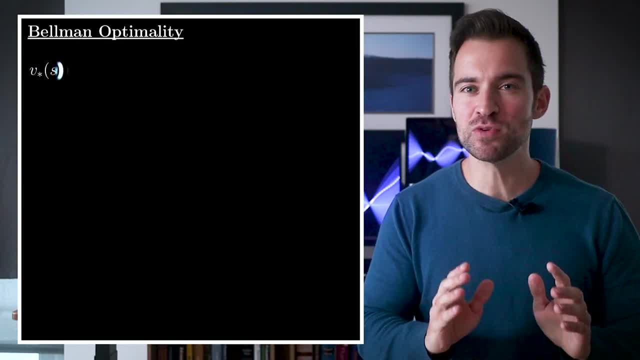 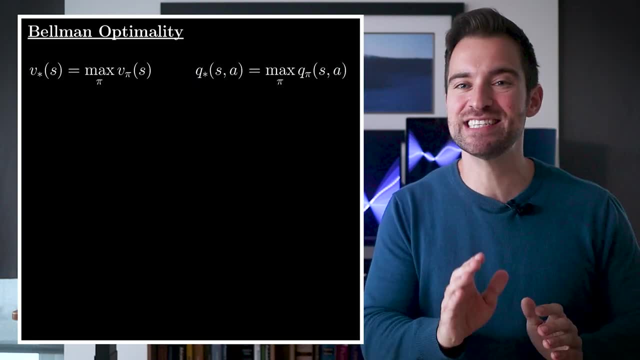 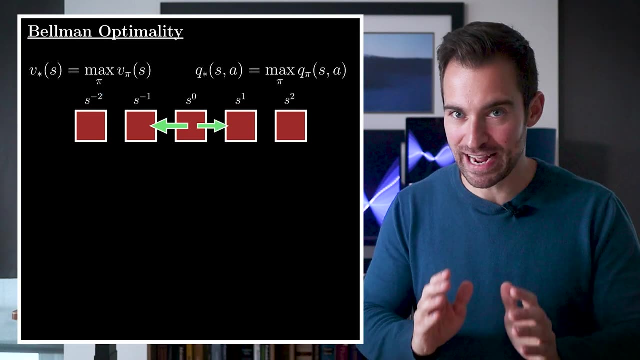 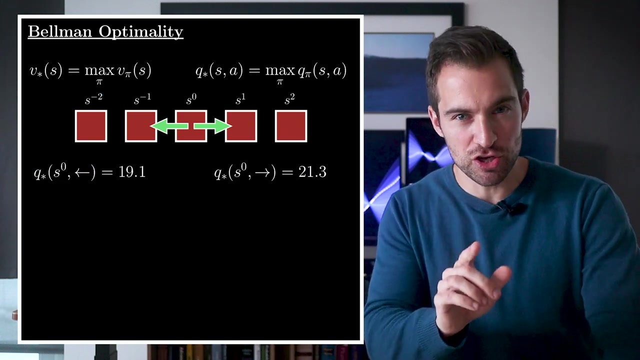 If you recall, the optimal state value function gives the highest possible values across all policies. The optimal action value function is the same for state action pairs. Now let's revisit those five states and focus again on the left and right actions. Okay, if I gave you the optimal action value for going left and going right, could you tell me the optimal state value of the center state? 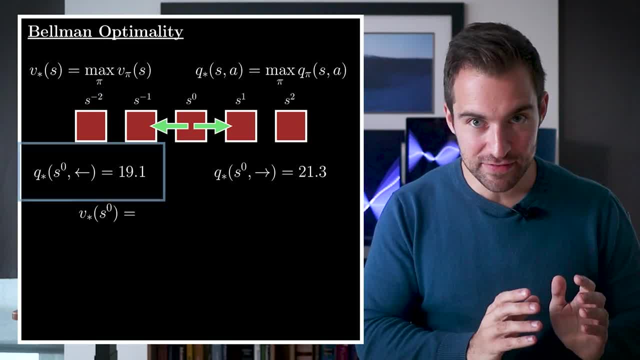 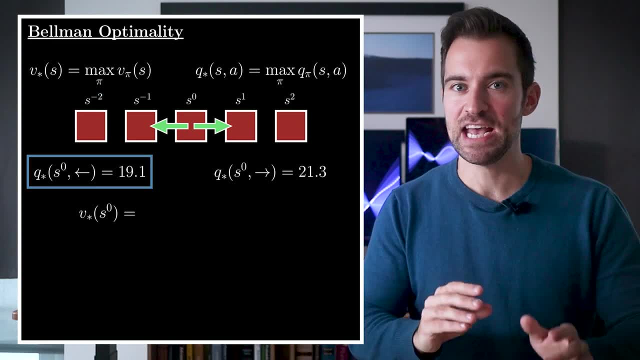 Just imagine you're the agent. If you select left and continue to follow whatever the optimal policy is, you'll get on average a return of 19.1.. If you select right, you'll get, on average a return of 21.3.. 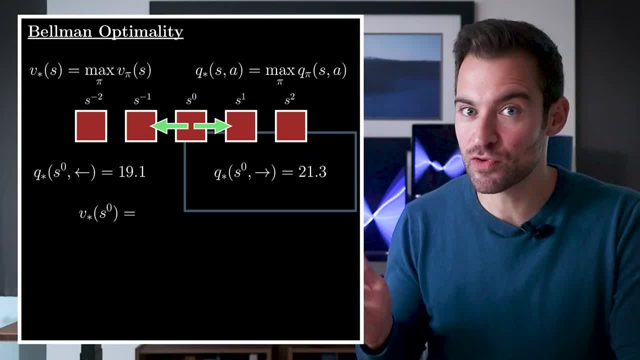 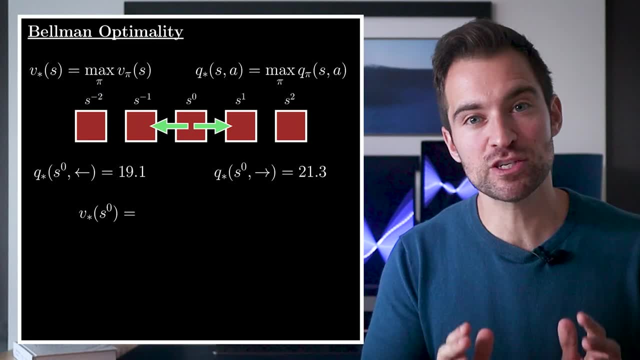 So what would you do? Clearly, select right. There's more reward there And in fact it's obvious that's what the optimal policy must do. Otherwise you're leaving expected return on the table. That means the value of the center state must be 21.3.. 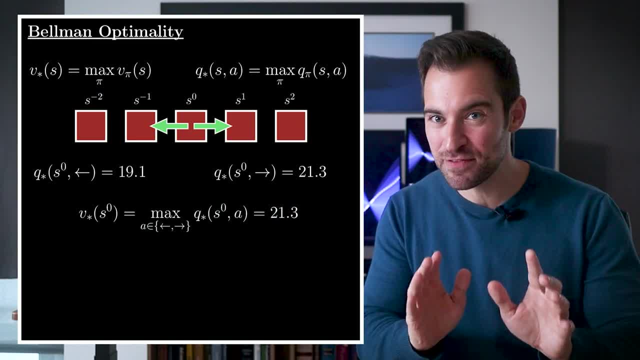 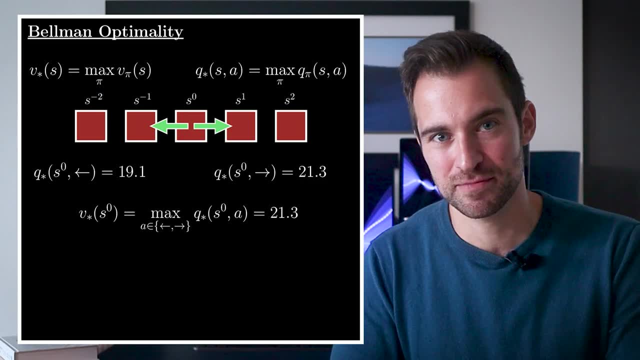 It's the max action value And that's the fundamental condition of Bellman optimality. The agent must always select the highest action value, Otherwise it's not behaving optimally. Now there is one complication that arises from multiple actions achieving the same highest value. 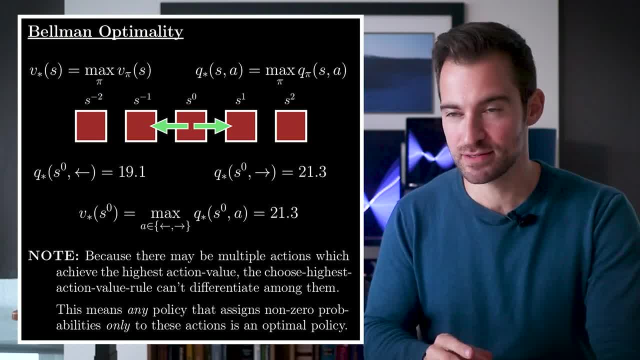 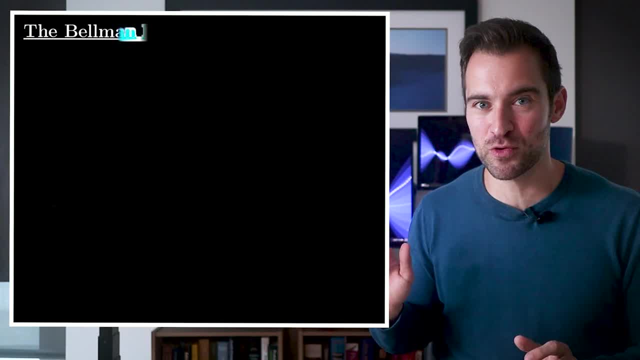 It just means that there are multiple optimal policies. Read this for more details. Okay, at this point it'll help if we take a step back and talk generally about the Bellman equations. What we've seen is that for any policy and for all states and for all actions in each state, 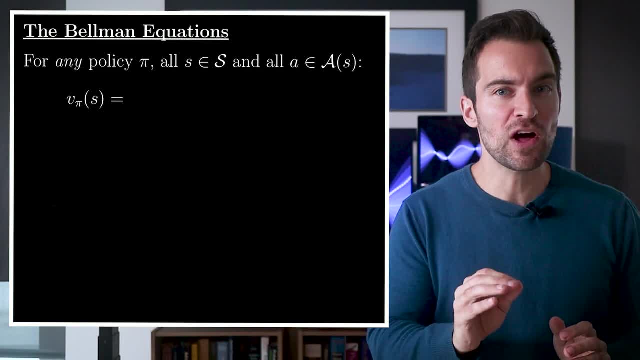 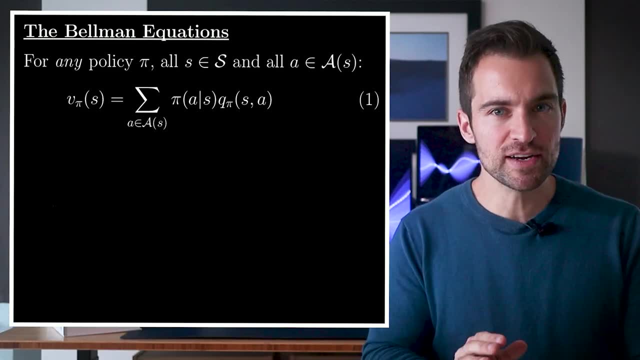 we have the following: The value of a state when following the policy pi is equal to the policy weighted average of the action values, which is something we saw earlier. To be clear, if we had 100 states, this would provide 100 equations. 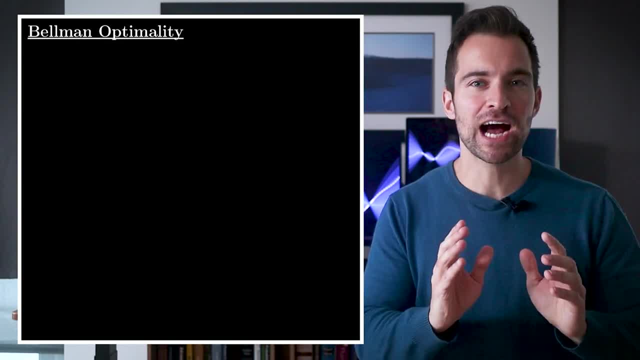 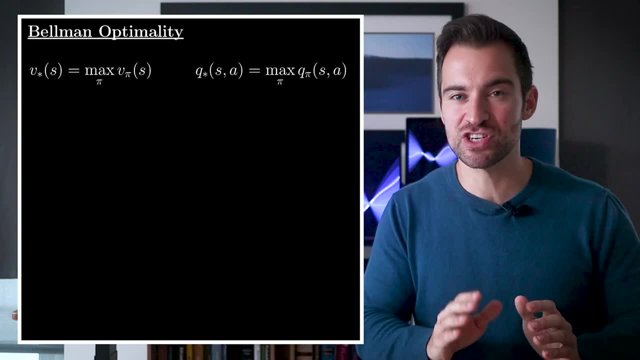 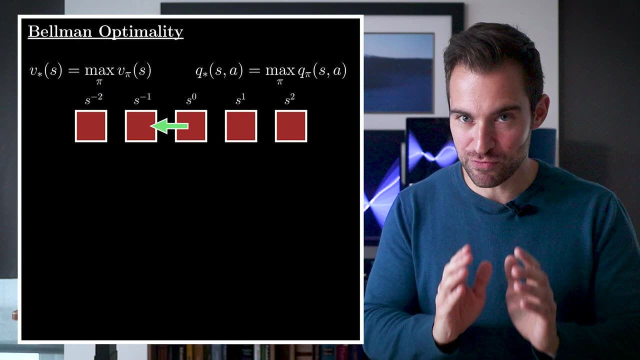 equation for state value functions. If you recall, optimal state value function gives the highest possible values across all policies. The optimal action value function is the same for state action pairs. Now let's revisit those five states and focus again on the left and right actions. Okay, if I gave you the optimal action value for going. 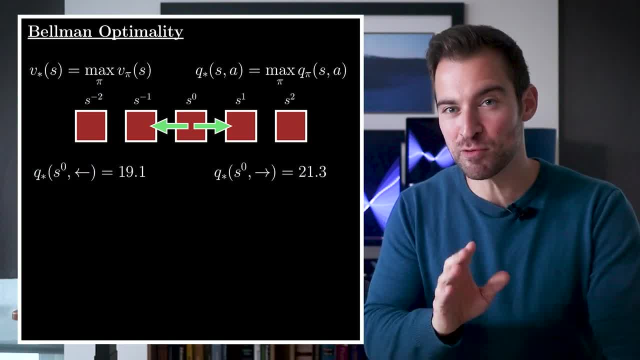 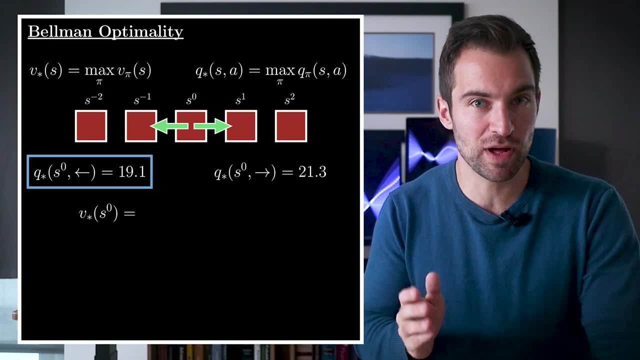 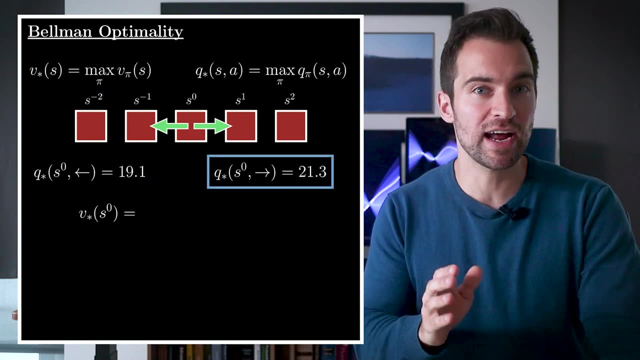 left and going right. could you tell me the optimal state value of the center state? Just imagine you're the agent. If you select left and continue to follow whatever the optimal policy is, you'll get on average a return of 19.1.. If you select right, you'll get on average a return of. 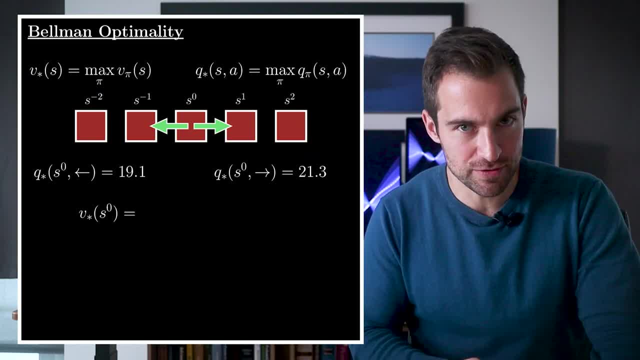 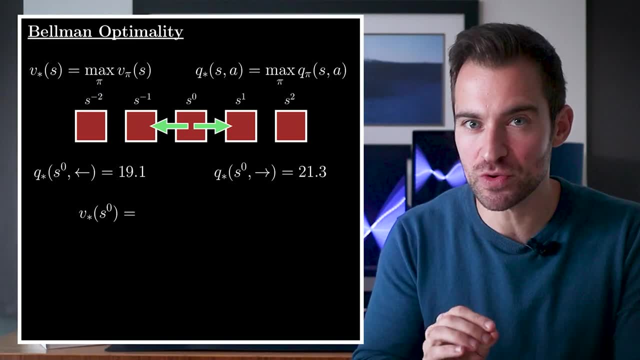 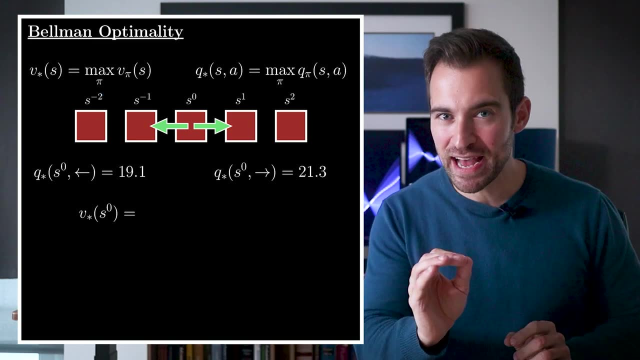 21.3.. So what would you do? Clearly, select right. There's more reward there And in fact it's obvious that's what the optimal policy MUST do. Otherwise you're leaving expected return on the table. That means the value of the center state MUST be 21.3.. It's the max action. 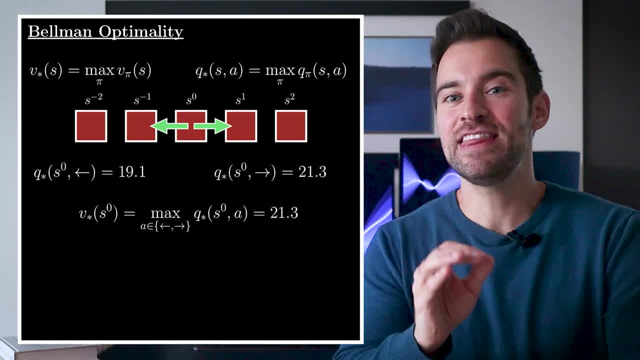 value, And that's the fundamental condition of Bellman optimality. That is the agent value of a two-component set of five states. So what would you do? You simply use a value of 0.03.. And you're must always select the highest action value. 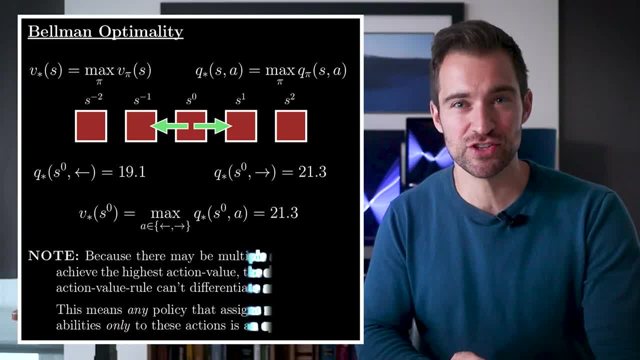 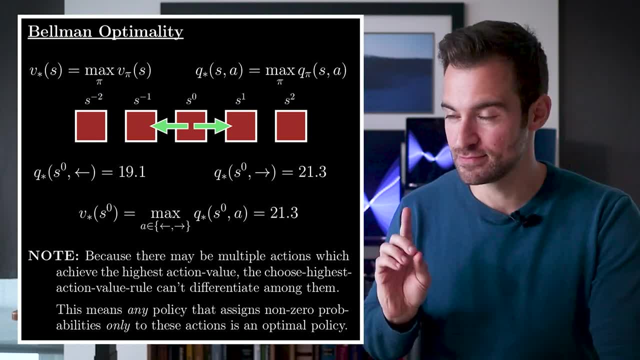 Otherwise it's not behaving optimally. Now there is one complication that arises from multiple actions achieving the same highest value. It just means that there are multiple optimal policies. Read this for more details. Okay, at this point it'll help if we take a step back. 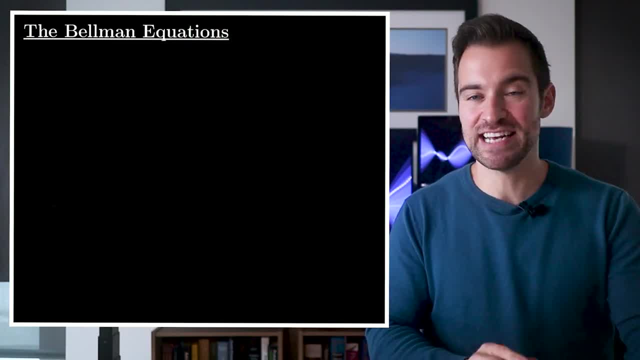 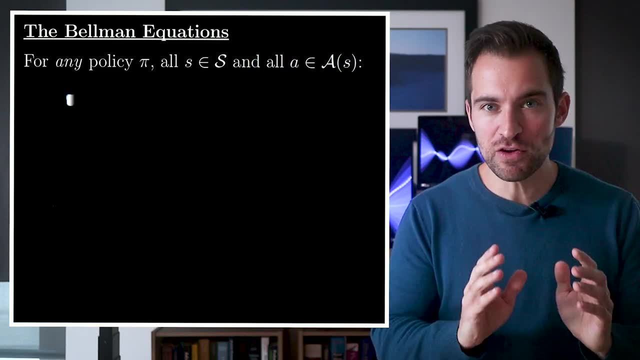 and talk generally about the Bellman equations. What we've seen is that for any policy and for all states and for all actions in each state, we have the following: The value of a state when following the policy, pi, is equal to the policy weighted average. 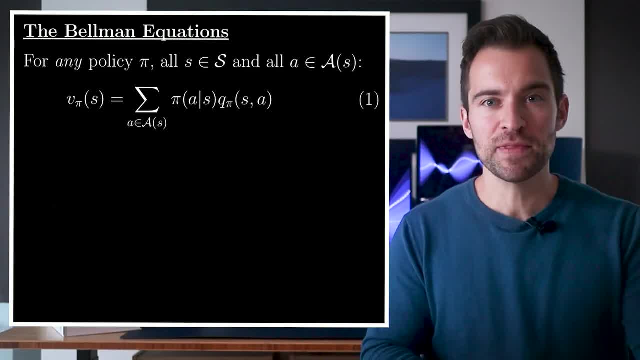 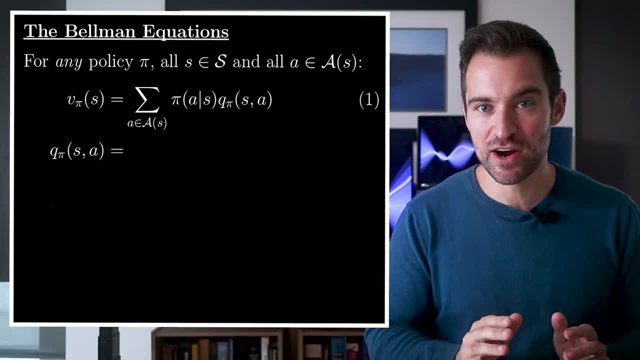 of the action values, which is something we saw earlier. To be clear, if we had 100 states, this would provide 100 equations. Second, the action value of a state action pair is the probability weighted average of the reward you'll get in the next step. 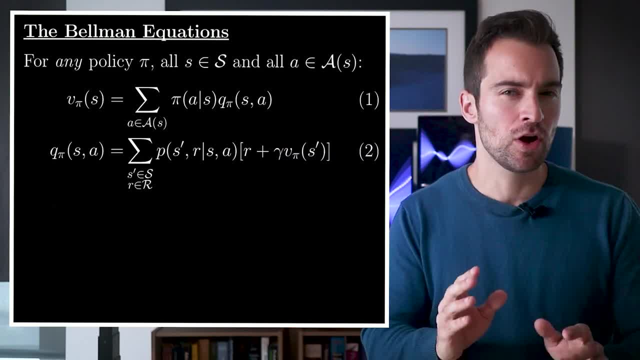 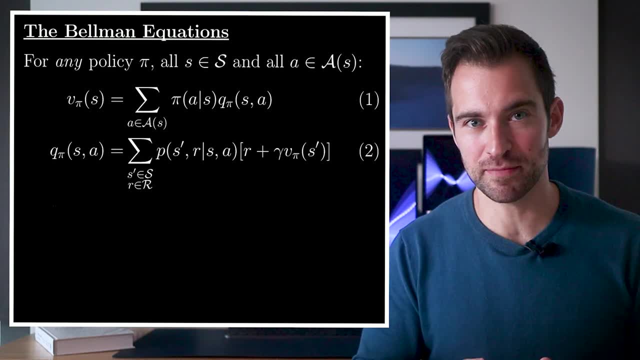 and the once discounted value of the next state. Hopefully, given what we've covered already, these equations make sense to you. Now, these aren't the Bellman equations, But they can be used to build them. To frame this, I'll use a grid with the state. 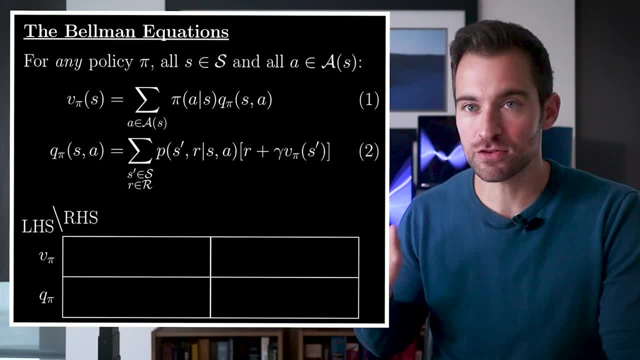 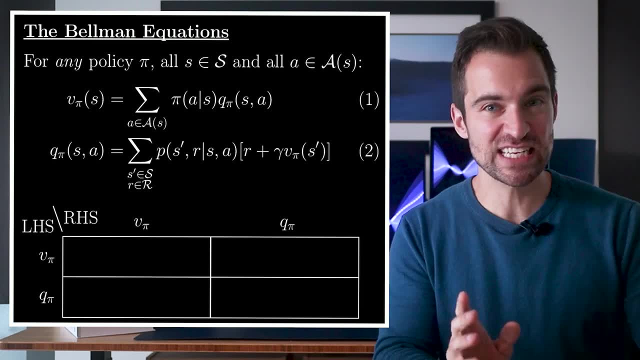 and action value along the rows and along the columns. Each of these cells will refer to an equation where what appears on the left-hand side of the equation is given by the row label and what appears within the right-hand side is given by the column label. 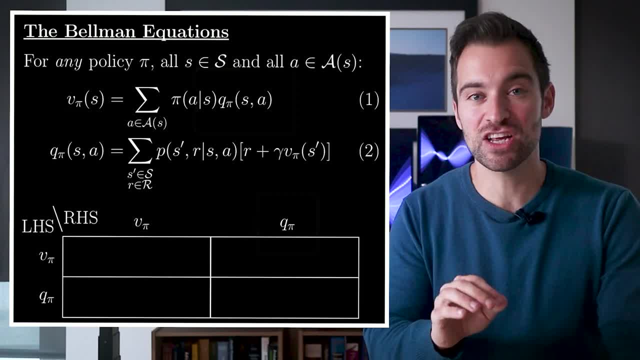 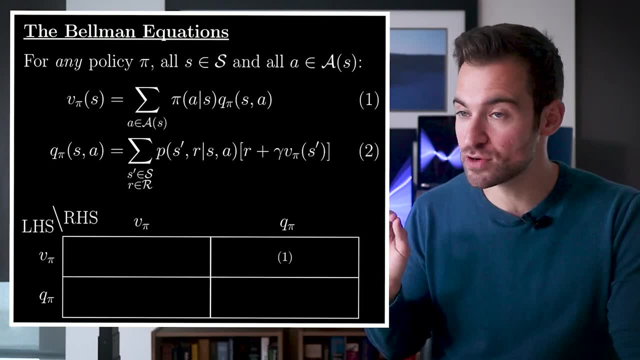 For example, an equation with v on the left-hand side and q in the right-hand side is given by equation one. Naturally, equation two goes here. All I'm doing is organizing things a bit, But here's the nice part. The grid suggests something more. 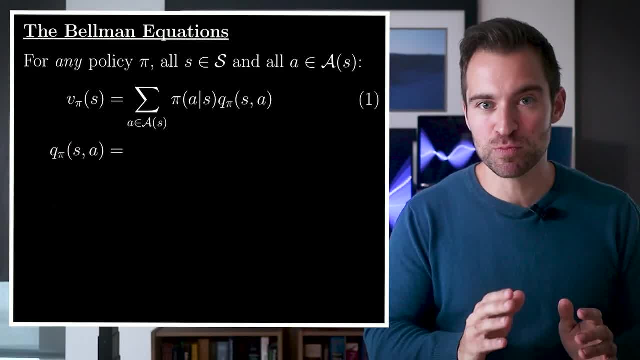 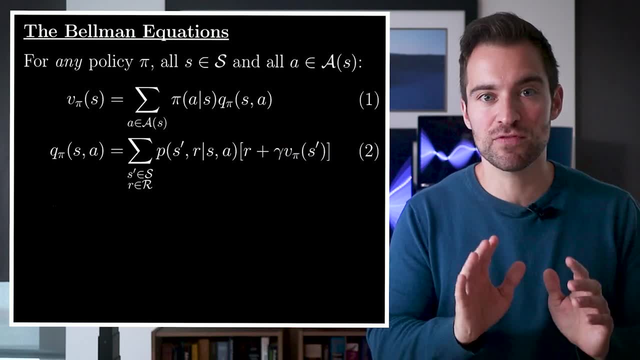 Second, the action value of a state-action pair is the probability weighted average of the reward you'll get in the next step and the once-discounted value of the next state. Hopefully, given what we've covered already, these equations make sense to you. 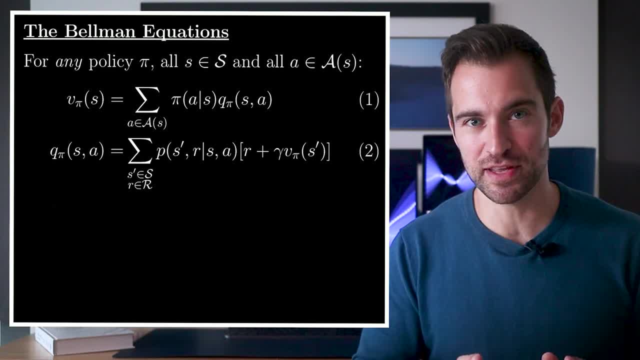 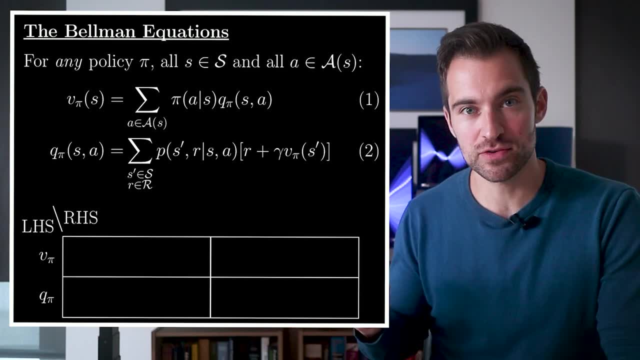 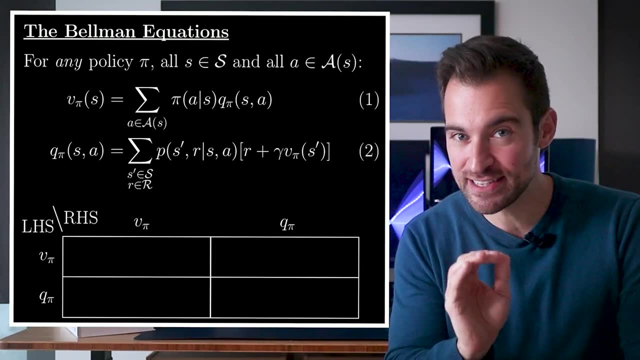 Now, these aren't the Bellman equations, but they can be used to build them. To frame this, I'll use a grid with the state and action value along the rows and along the columns. Each of these cells will refer to an equation where what appears on the left-hand side of the equation 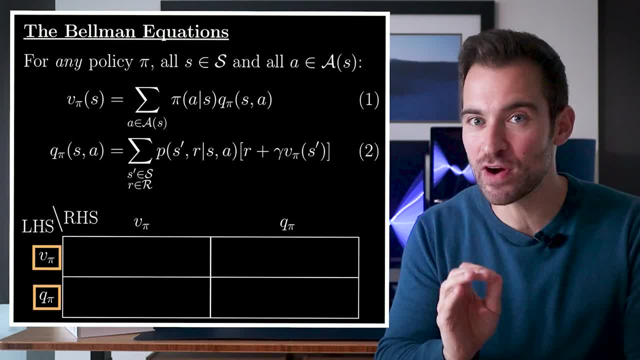 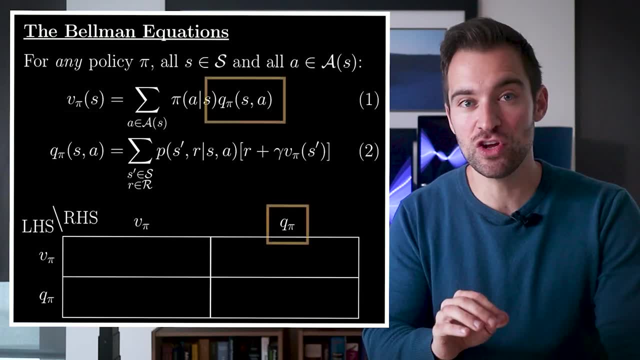 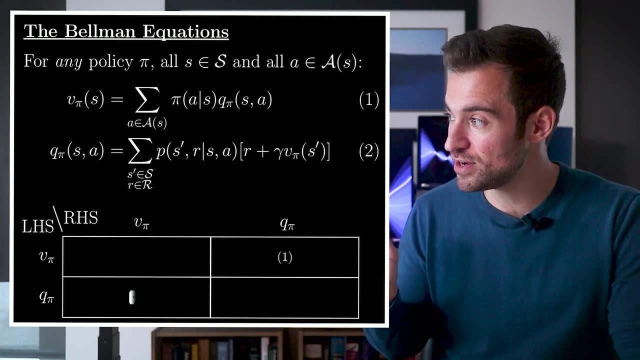 is given by the row label and what appears within the right-hand side is given by the column label. For example, an equation with V on the left-hand side and Q in the right-hand side is given by equation 1.. And naturally equation 2 goes here. 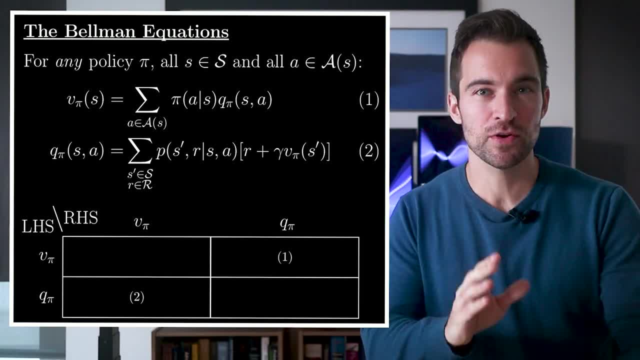 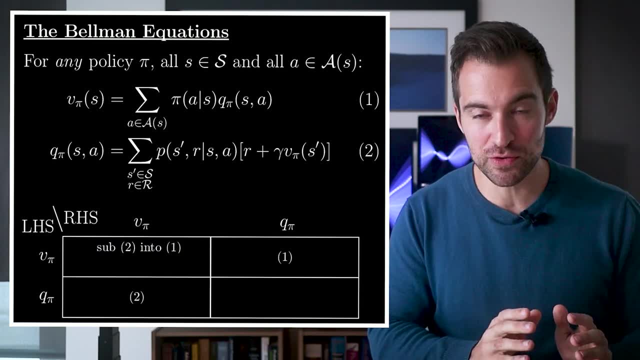 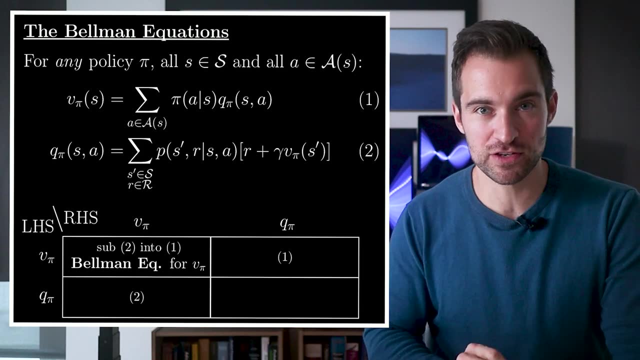 All I'm doing is organizing things a bit. But here's the nice part: The grid suggests something more. If we substitute 2 into 1, we can relate any state value to all state values one step away, And this gives us the Bellman equation for the state-value function. 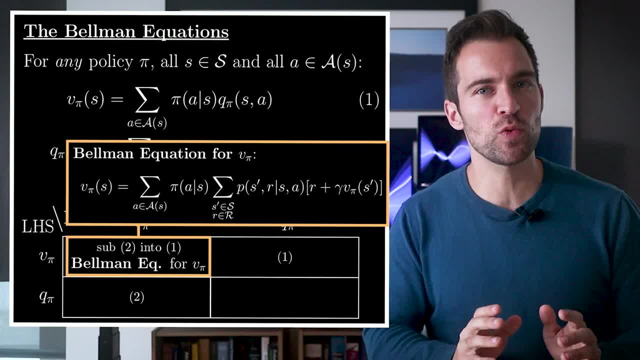 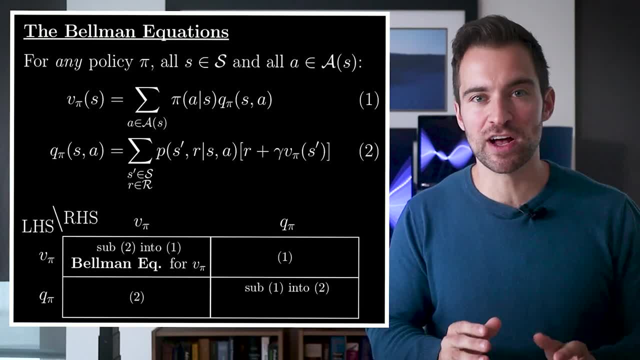 Here it is written out explicitly. This is exactly what we worked through earlier in the video, And if we substitute 1 into 2, we can relate any action value to all action values one step away, giving us the Bellman equation for the action-value function. 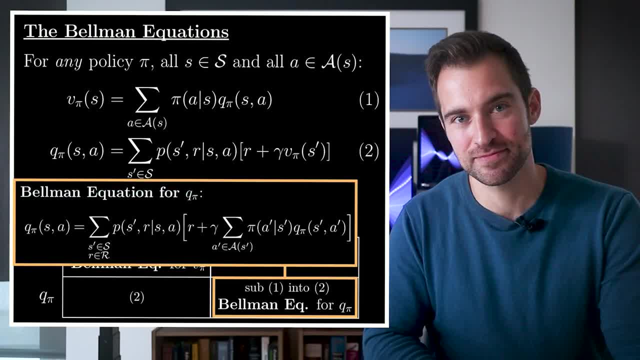 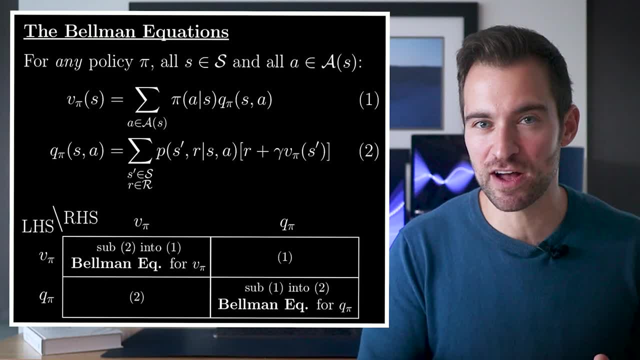 Again, here is what the equation looks like written out explicitly. Now the most important thing to understand is using the MDP distribution. the Bellman equations allow us to calculate state values from one-step-away state values. something similar for state-action pairs. 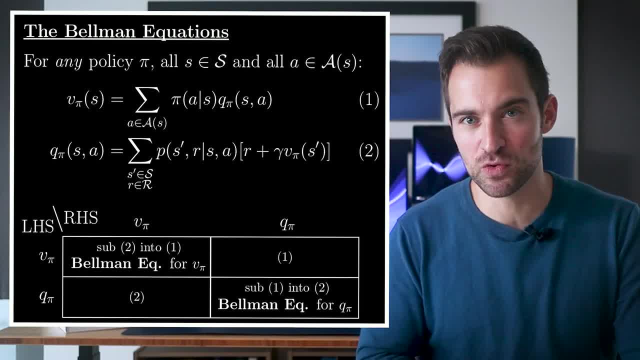 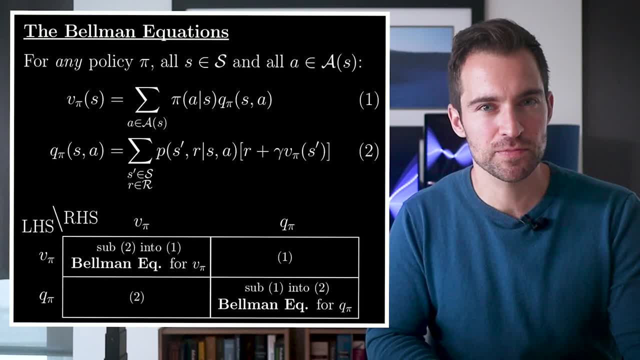 Also, for each unknown value of the function there is a Bellman equation, So finding the solution can be thought of as solving a system of equations. Finally, there's something else that's nice about this view: To refer to the Bellman optimality equations. 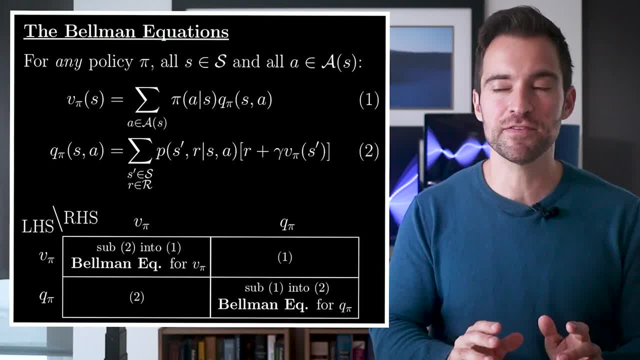 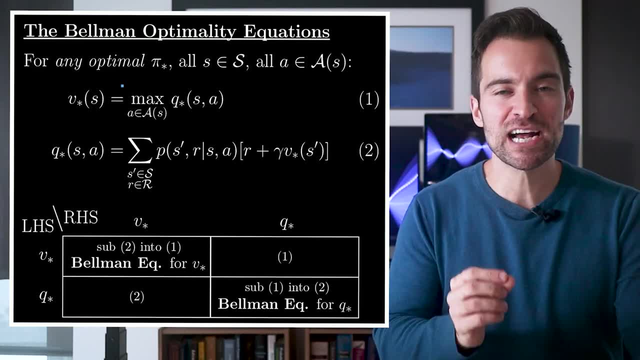 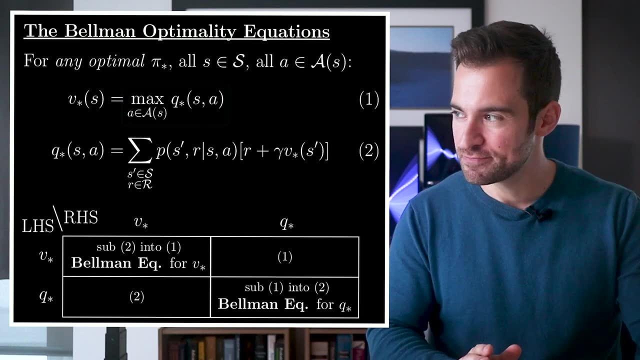 which concern optimal policies in particular. we only need to make a few modifications. There's basically only one tweak to call out: The state value must be the maximum over optimal action values, like we discussed earlier. Structurally, everything else is exactly the same. 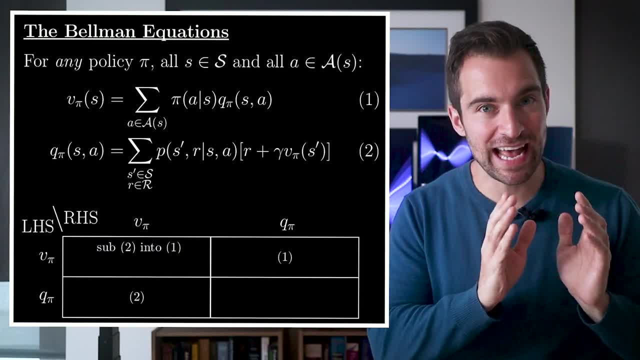 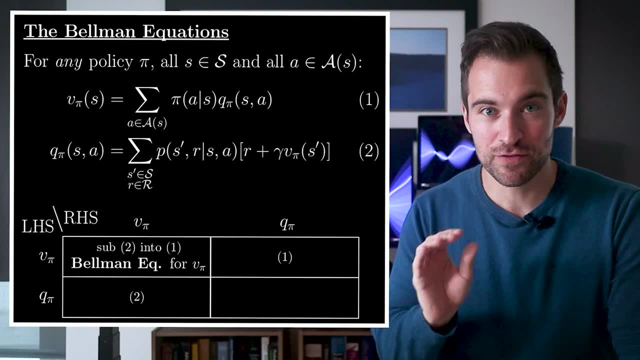 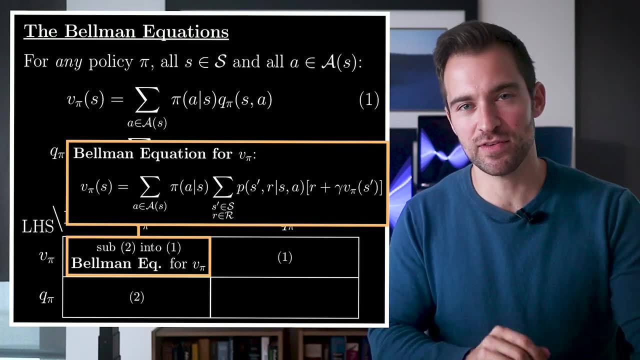 If we substitute two into one, we can relate any state value to all state values one step away. This gives us the Bellman equation for the state-value function. Here it is written out explicitly. This is exactly what we worked through earlier in the video. 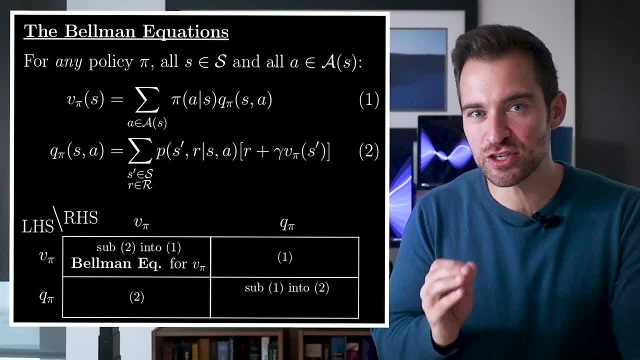 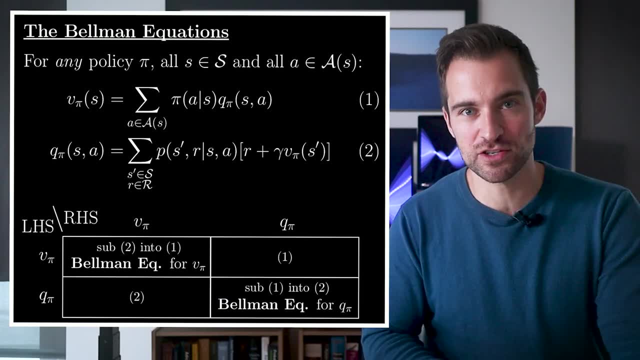 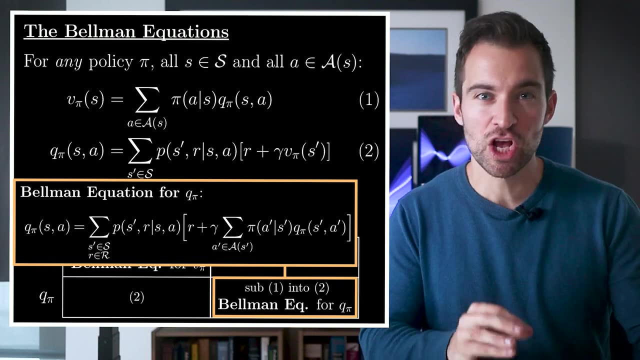 And if we substitute one into two, we can relate any action value to all action values one step away, giving us the Bellman equation for the action value function. Again, here is what the equation looks like written out explicitly. Now, the most important thing to understand is: 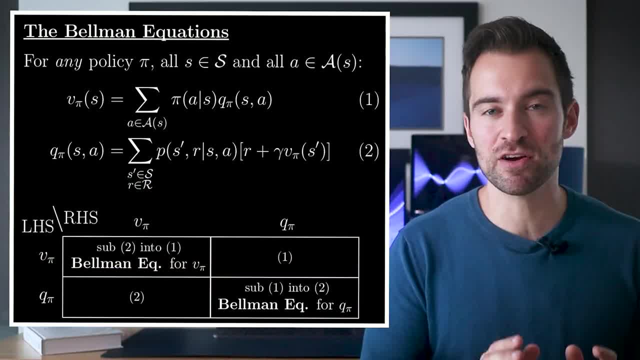 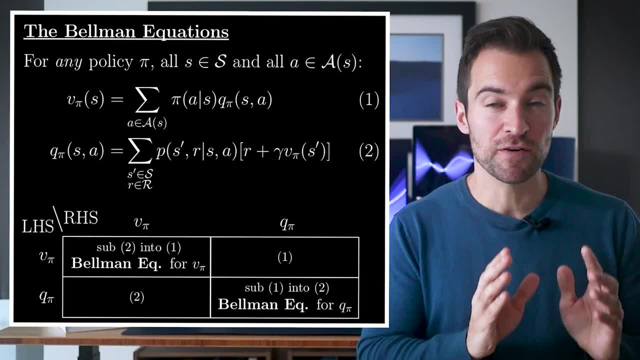 using the MDP distribution. the Bellman equations allow us to calculate state values from one step away state values and to do something similar for state action pairs. Also, for each unknown value of the function there is a Bellman equation, So finding the solution can be thought of. 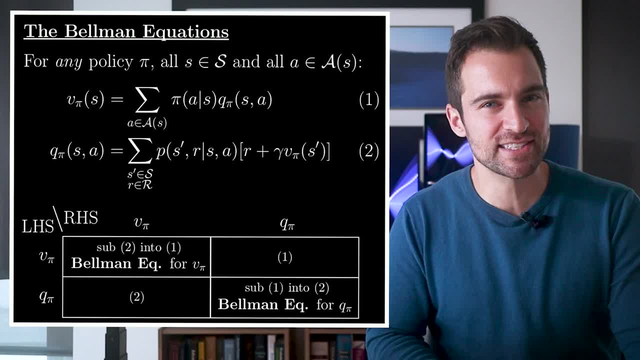 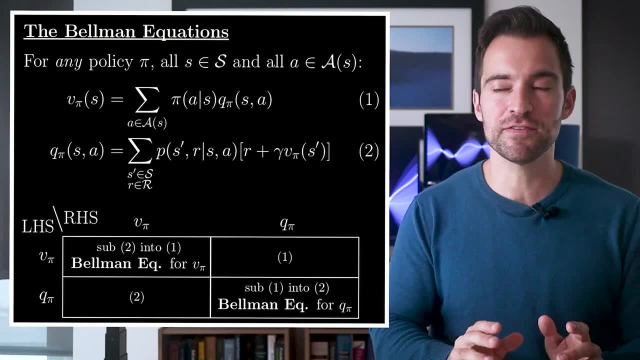 as solving a system of equations. Finally, there's something else that's nice about this view. To refer to the Bellman optimality equations, which concern optimal policies in particular, we only need to make a few modifications. There's basically only one tweak to call out. 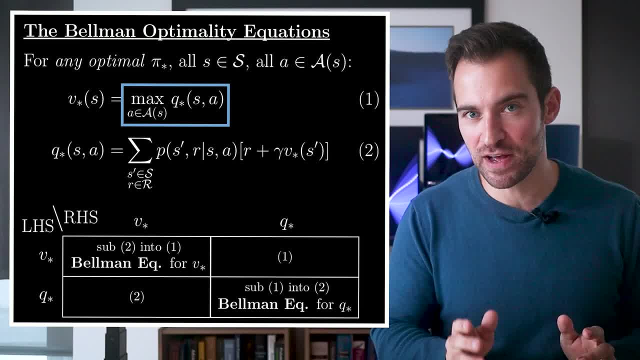 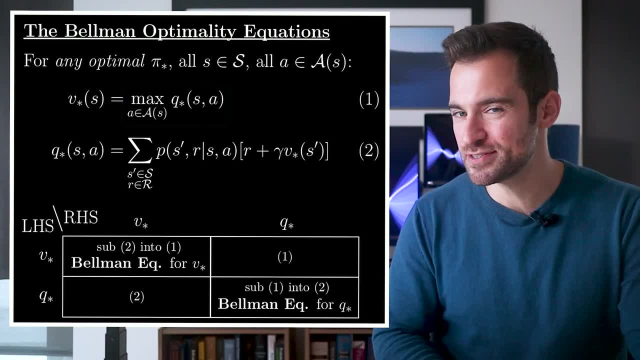 The state value must be the maximum over optimal action values, like we discussed earlier. Structurally, everything else is exactly the same. Take a second to absorb this. Okay, now let's step way back and remember: our original goal is to find an optimal policy. 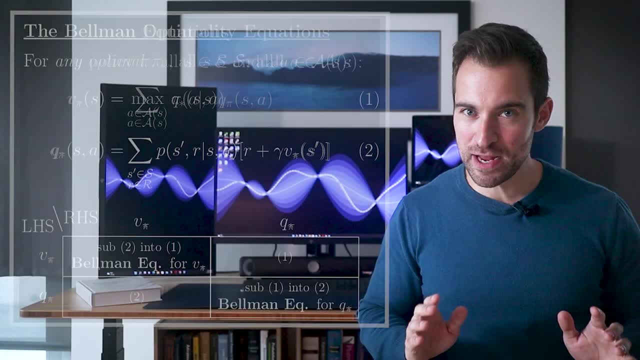 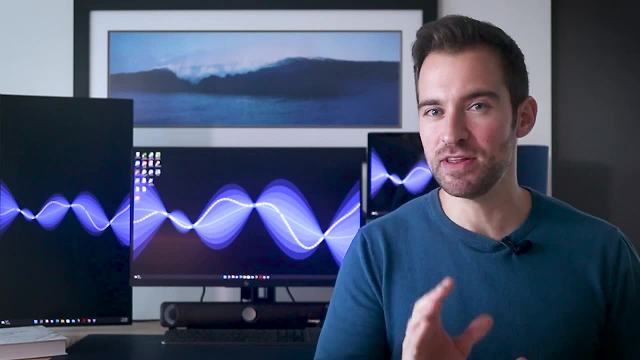 Take a second to absorb this. Okay, now let's step way back and remember: our original goal is to find an optimal policy for a given MDP. As we'll see, the Bellman equations will be the backbone of our algorithms to do this. 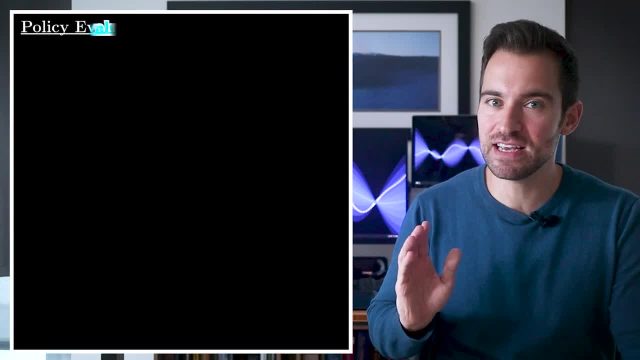 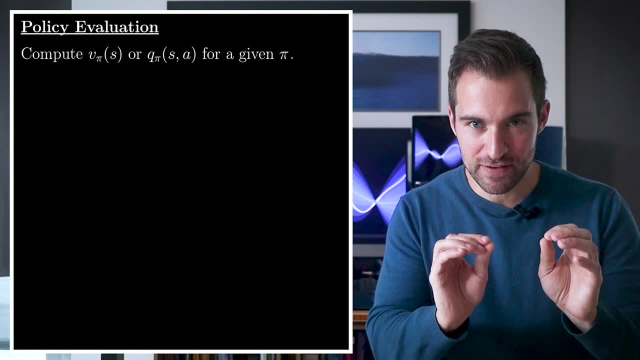 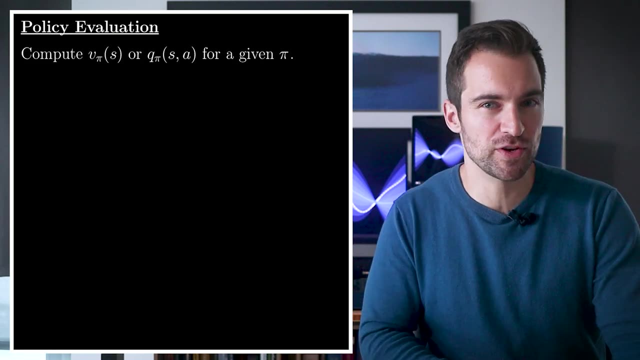 In particular, we'll see that a major subroutine is policy evaluation. This refers to computing the state-value function or action-value function for a given fixed policy, pi For all states, or state-action pairs under some MDP. Now there are several ways we could approach this. 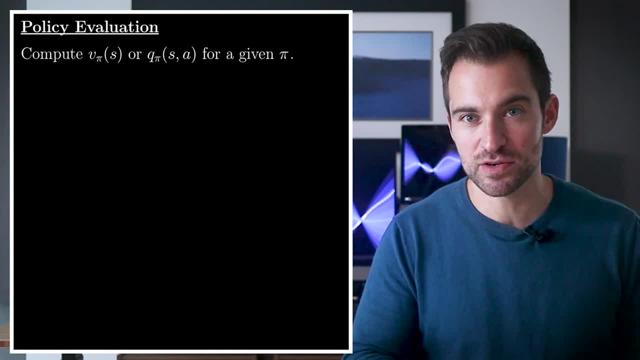 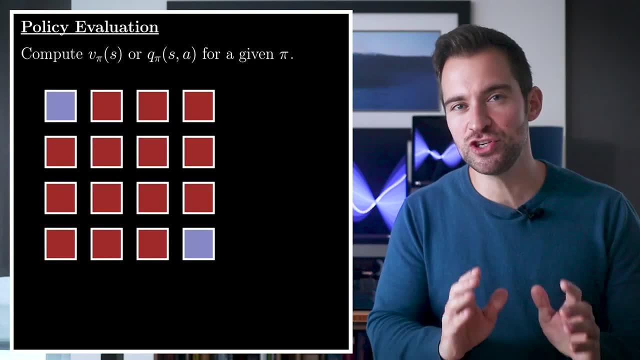 In our case, we'll consider a very simple iterative solution, which we'll explore with example 4.1 from Sutton and Bardo. Here's the setup: We have 16 states, of which two are terminal. In each state, the agent can move up, down, left or right. 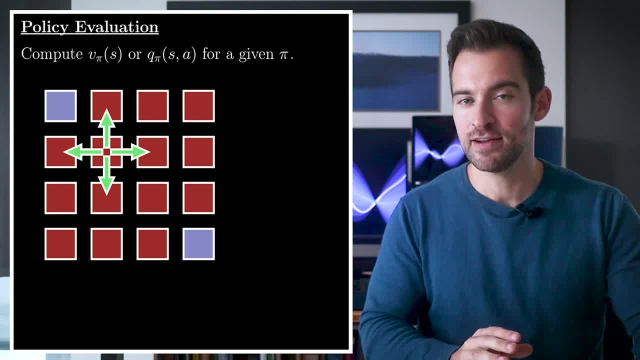 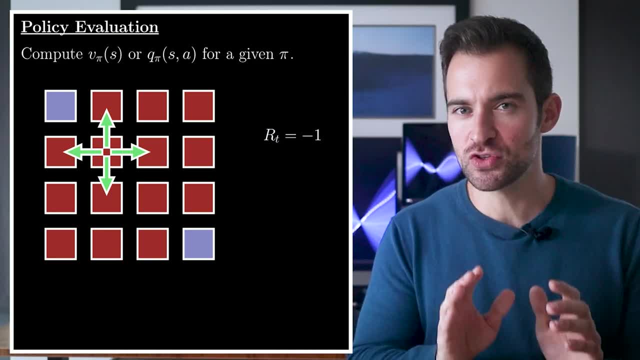 and that will deterministically move it to whichever neighboring state, unless that state is off the grid, in which case nothing happens. Every move will incur a reward of minus one and there's no discounting. So the goal is to reach a terminal state as quickly as possible. 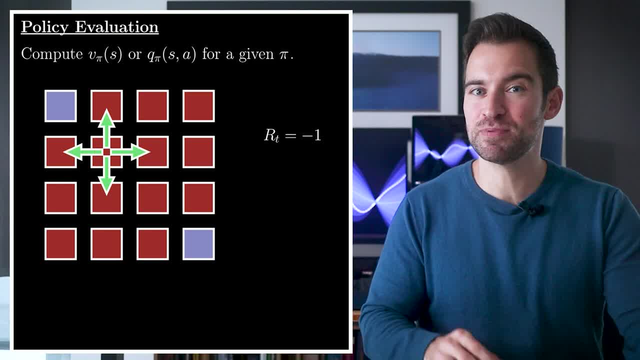 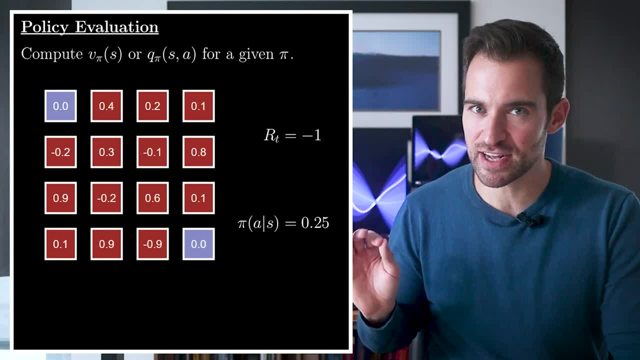 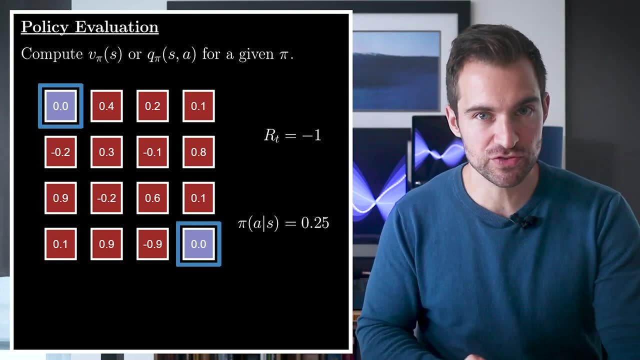 And here's the question: Given a policy which simply samples actions with equal probability, what is its value function? Well, the approach starts by randomly initializing the state values, with the exception that the terminal states must have a value of zero, which is always true. 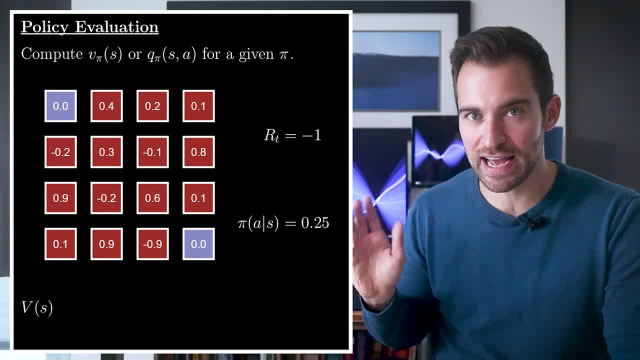 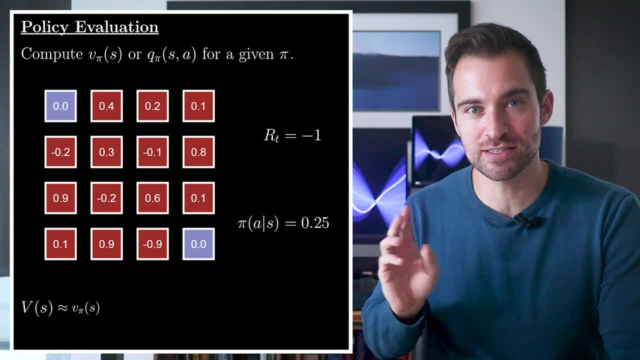 We will refer to each of these values with a capital Vs. It's capital because, especially in our future algorithms, it's a random estimate which approximates the true value. Okay now, clearly these values aren't the solution, And we know that because they don't obey the Bellman equation. 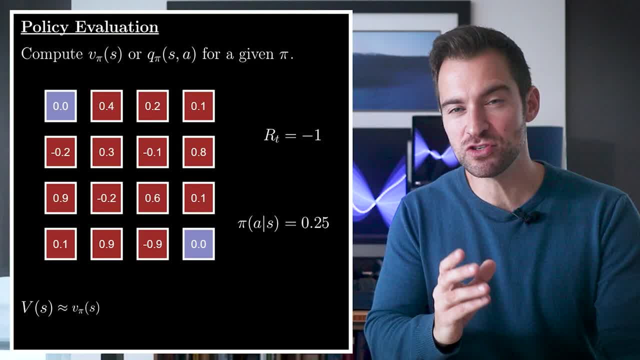 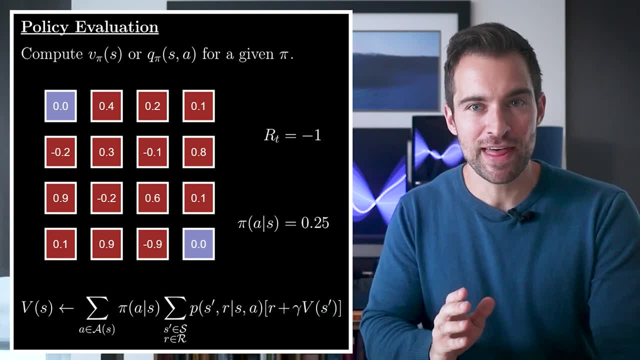 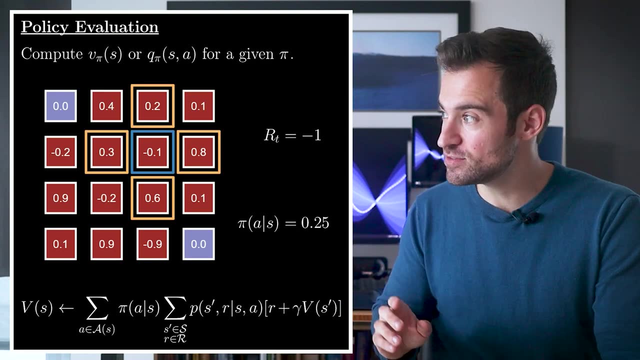 But what's the simplest thing we could do to fix that? How about just reassigning each state value according to the Bellman equation, like this, For example: that means this value will be determined by these values. In fact, one application gives us this. 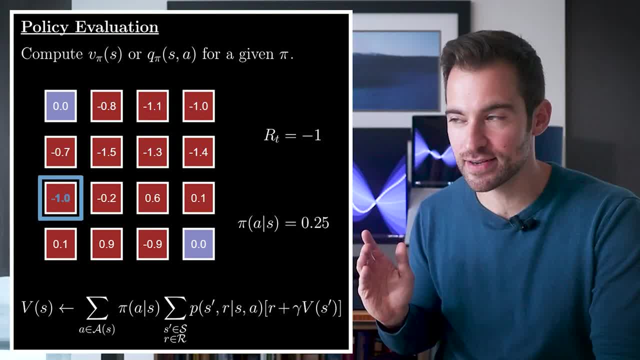 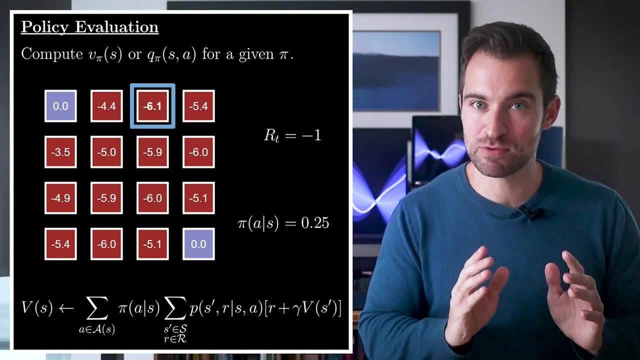 From here, we continue reassigning each state. One pass over all states is called a sweep, And we repeat these sweeps until the values stop changing by more than some small amount And, due to some nice theory, this process always converges to the right answer. 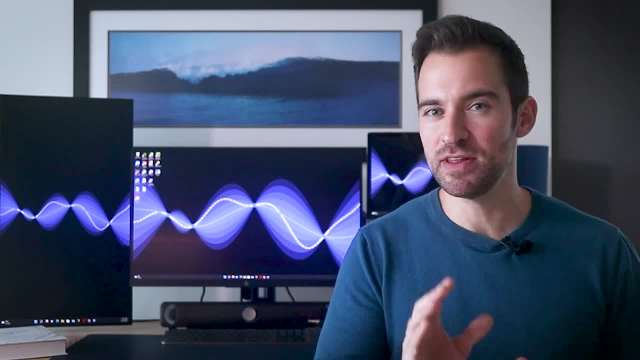 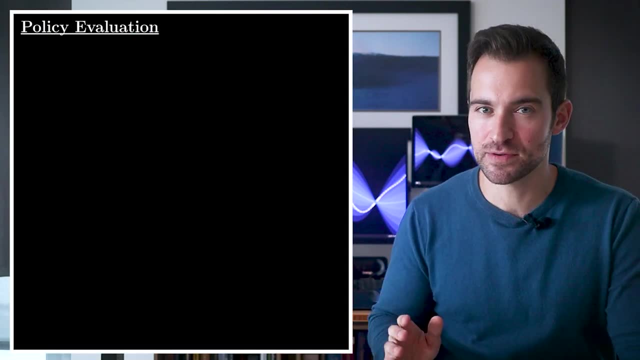 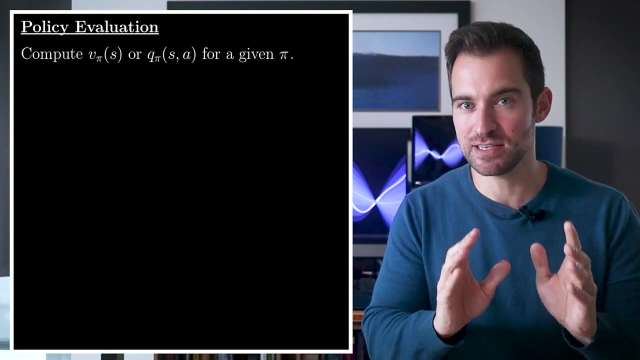 for a given MDP. As we'll see, the Bellman equations will be the backbone of our algorithms to do this. In particular, we'll see that a major subroutine is policy evaluation. This refers to computing the state value function or action value function for a given fixed policy pi. 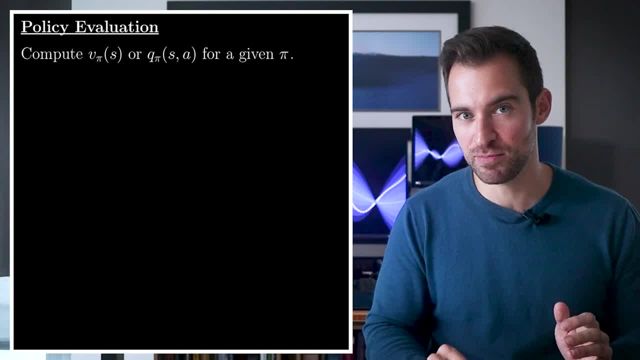 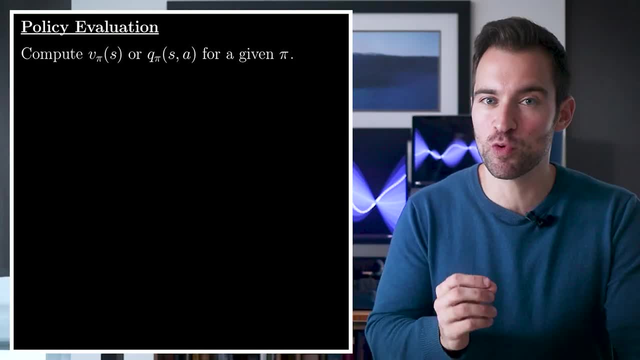 for all states or state action pairs under some MDP. Now there are several ways we could approach this. In our case, we'll consider a very simple iterative solution, which we'll explore with example 4.1 from Sutton and Bardo. 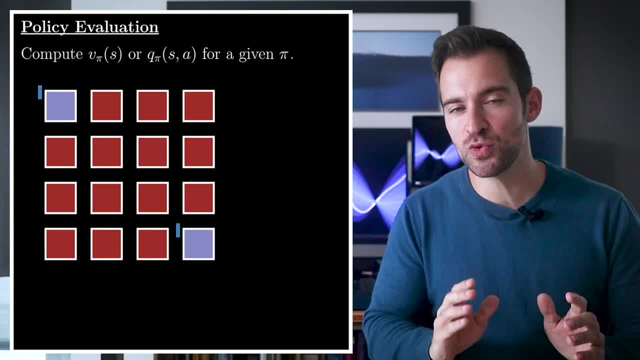 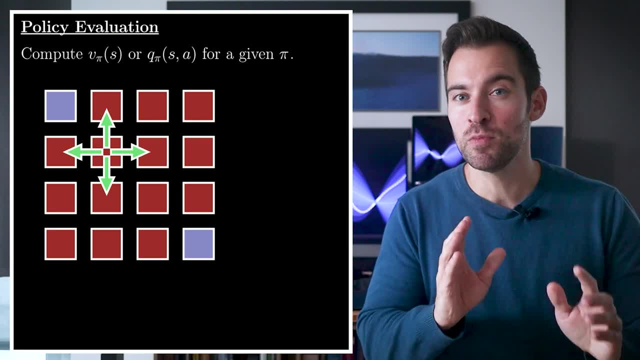 Here's the setup: We have 16 states, of which two are terminal. In each state the agent can move up, down, left or right, and that will deterministically move it to whichever neighboring state, unless that state is off the grid. 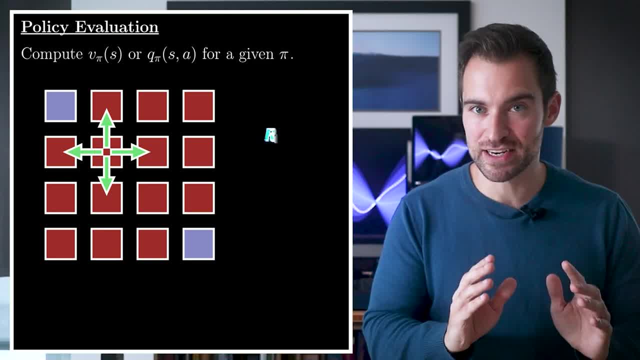 in which case nothing happens. Every move will incur a reward of minus one, and there's no discounting. So the goal is to reach out to the agent and then we'll see what happens. So let's take a look at how to approach a terminal state. 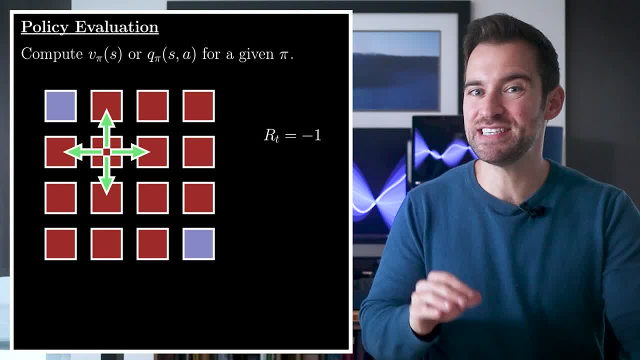 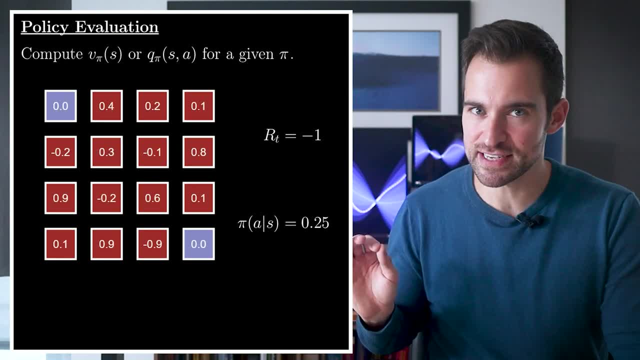 as quickly as possible. And here's the question: Given a policy which simply samples actions with equal probability, what is its value function? Well, the approach starts by randomly initializing the state values, with the exception that the terminal states must have a value of zero. 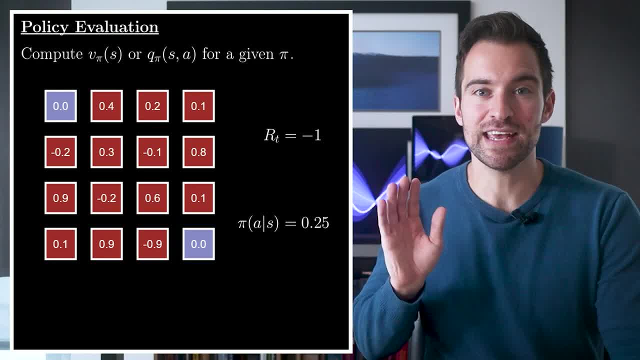 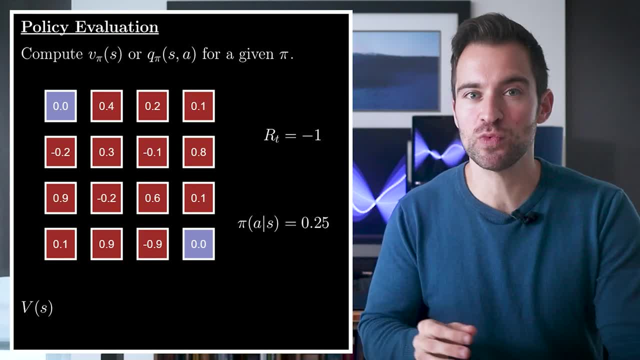 which is always true. We will refer to each of these values with a capital Vs. It's capital because, especially in our future algorithms, it's a random estimate, so it's not always true. OK now, clearly these values aren't the solution. 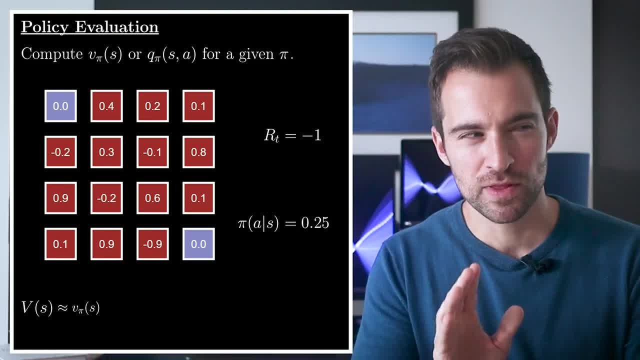 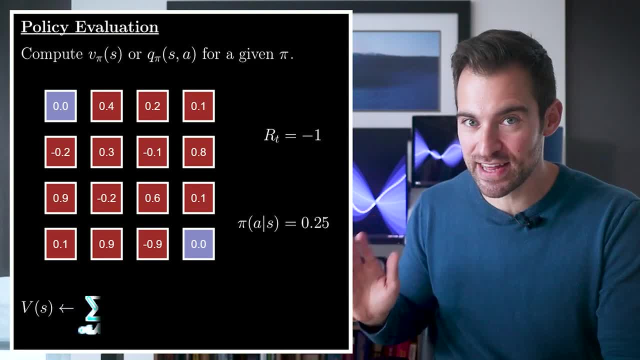 And we know that because they don't obey the Bellman equation. But what's the simplest thing we could do to fix that? How about just reassigning each state value according to the Bellman equation, like this, For example: that means this value will be determined. 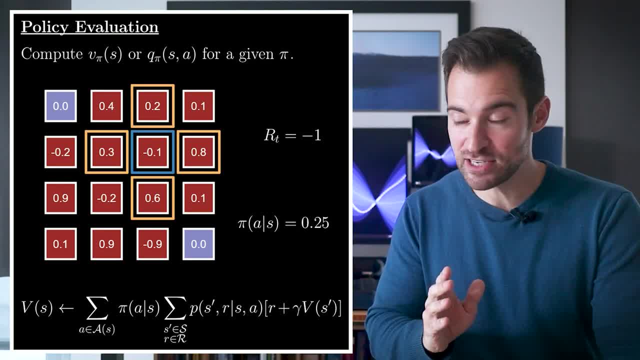 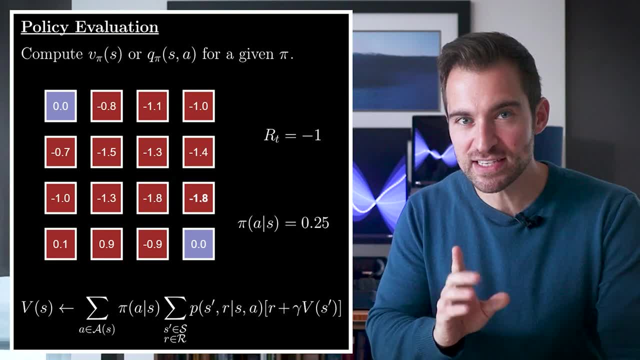 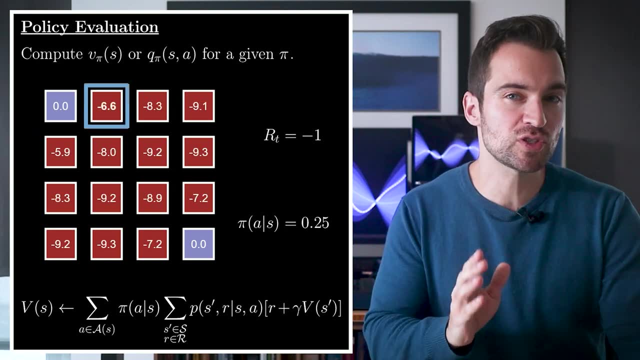 by these values. In fact, one application gives us this. From here, we continue reassigning each state. One pass over all states is called a sweep, And we repeat these sweeps until the values stop changing by more than some small amount. 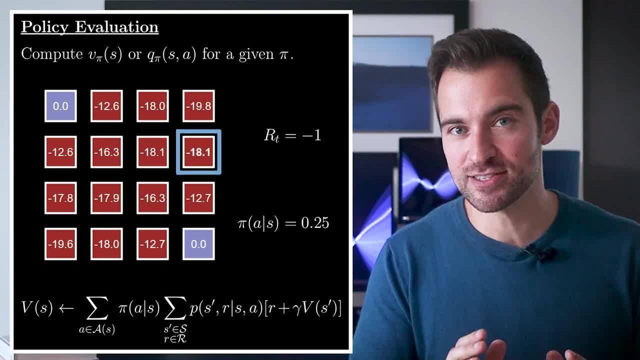 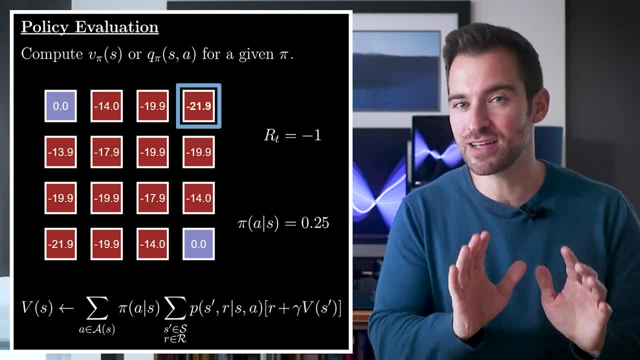 And due to some nice theory, this process always converges to the right answer. My intuition is that each assignment imports some small piece of the known MDP, always making the value estimates a little better. And that's it for policy evaluation. We just turned the Bellman equation into an assignment. 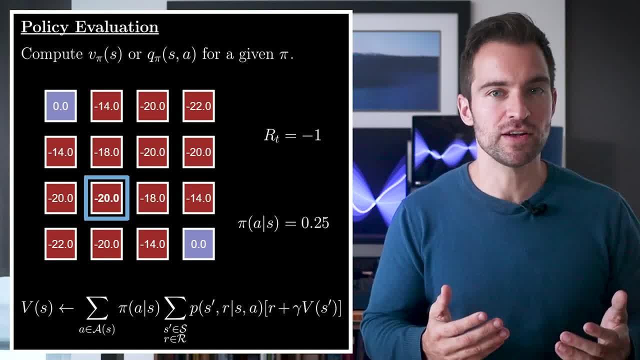 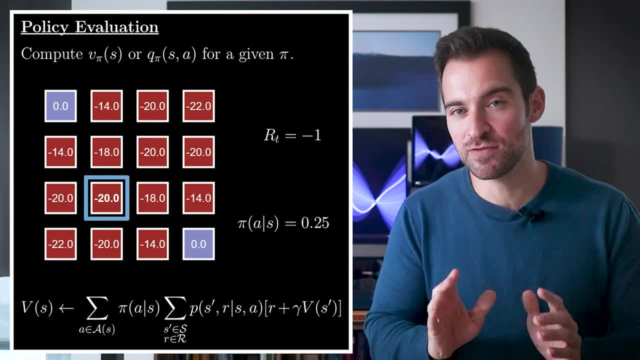 and repeatedly applied it, starting from random values. For action values, the process is virtually identical, except states are replaced with state-action pairs and we use the Bellman equation for the action value function instead. Next we'll cover another major subroutine. 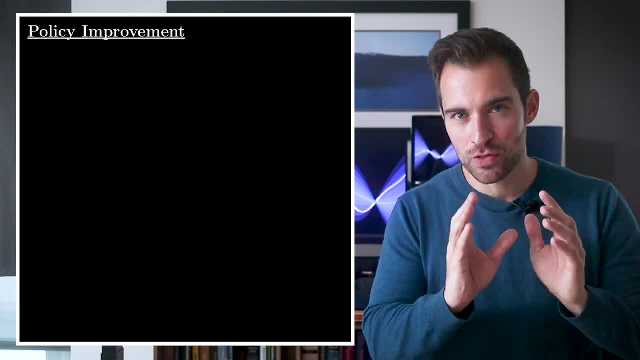 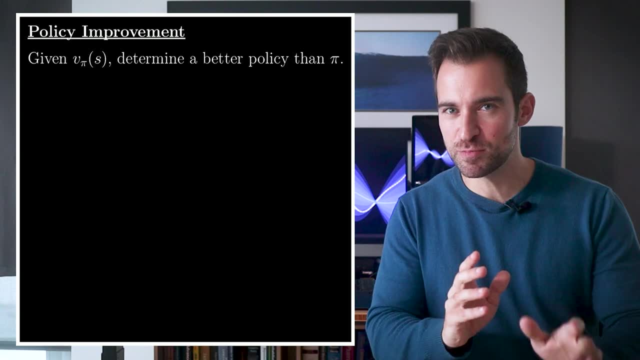 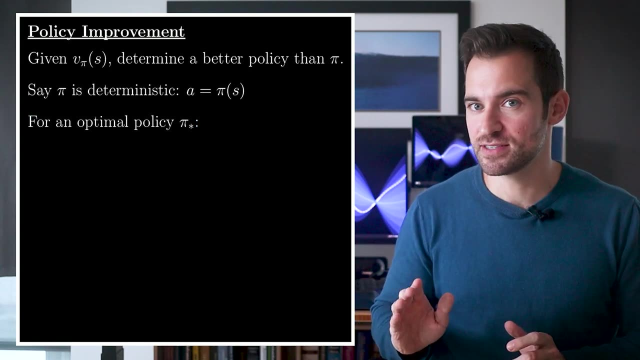 of many RL algorithms: policy improvement. The question here is: given the value function of some policy, pi, how can we determine a better policy? To explain this, let's say for simplicity: the policy is deterministic. Next, let's recall what an optimal policy does. 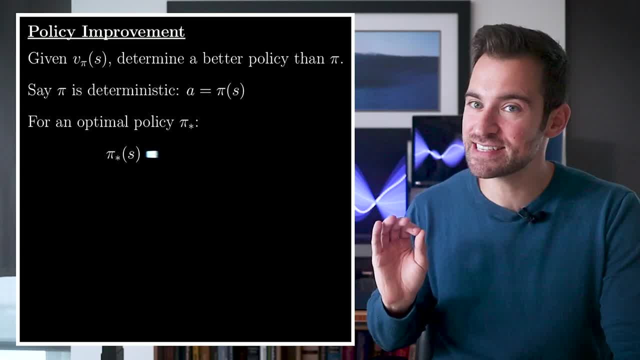 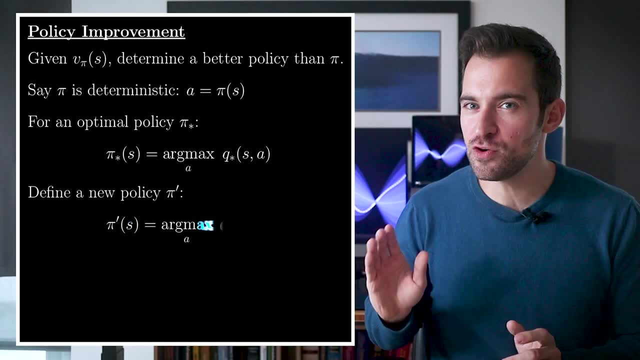 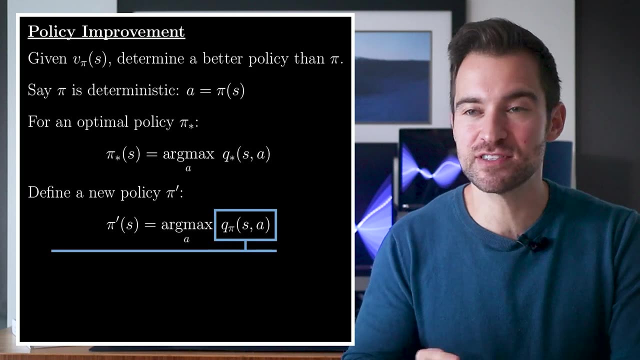 The action selected in each state must achieve the max action value. So does this inspire any ideas? Here's one. We define a new policy which always selects a max action value in every state. As a reminder, we can form the action values like this: 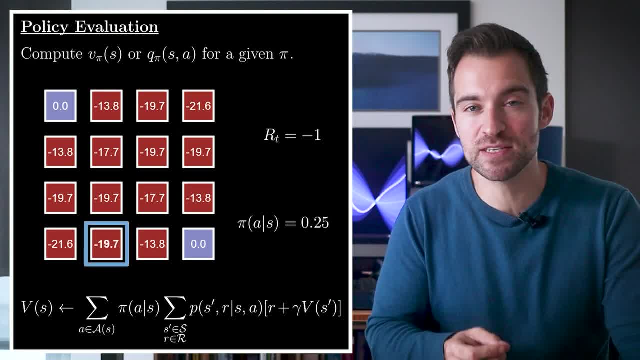 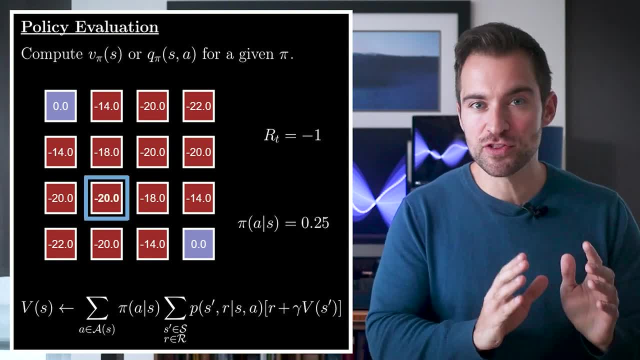 My intuition is that each assignment imports some small piece of the known MDP, always making the value estimates a little better. And that's it for policy evaluation. We just turned the Bellman equation into an assignment and repeatedly applied it, starting from random values. 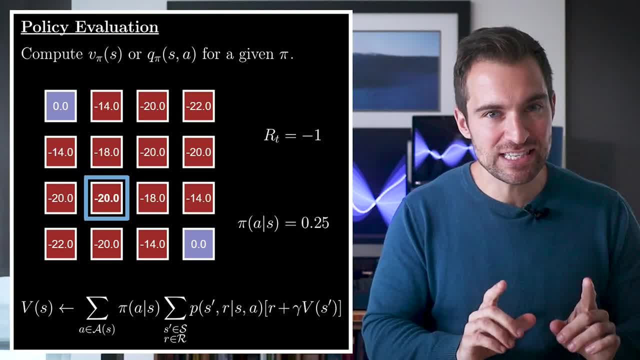 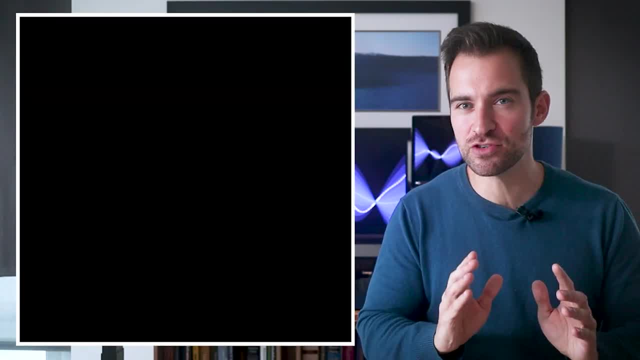 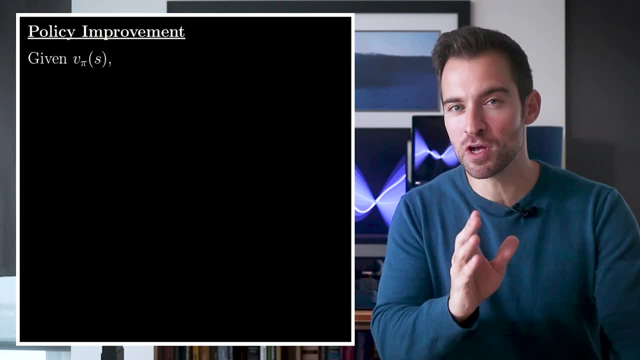 For action values. the process is virtually identical, except states are replaced with state-action pairs And we use the Bellman equation for the action value function instead. Next we'll cover another major subroutine of many RL algorithms: policy improvement. The question here is, given the value function of some policy pi. 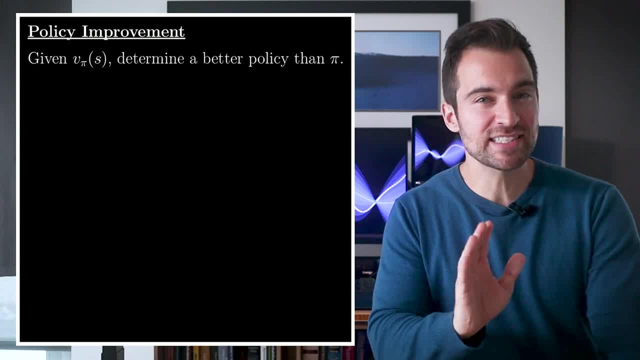 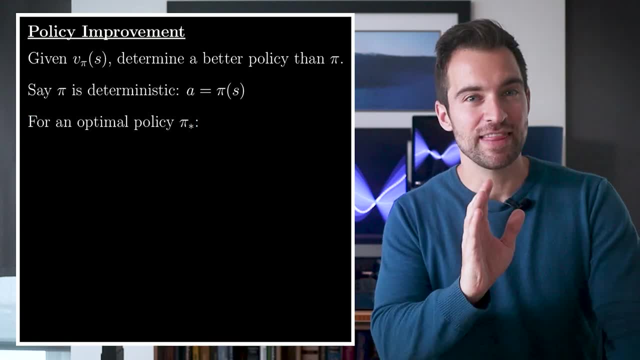 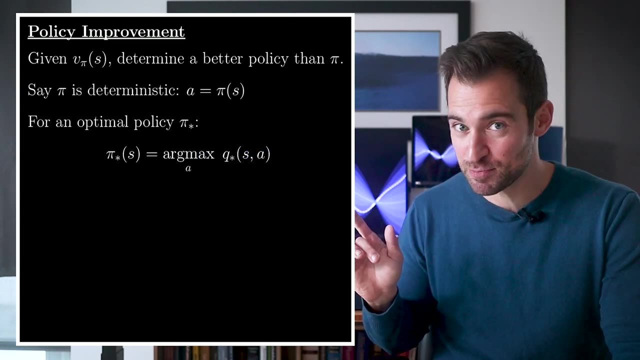 how can we determine a better policy? To explain this, let's say, for simplicity, the policy is deterministic. Next, let's recall what an optimal policy does. The action selected in each state must achieve the max action value. So does this inspire any ideas? 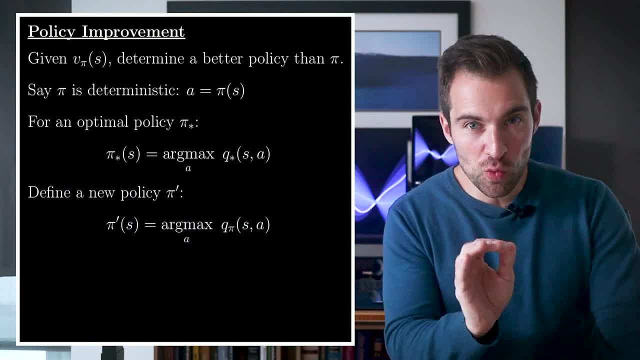 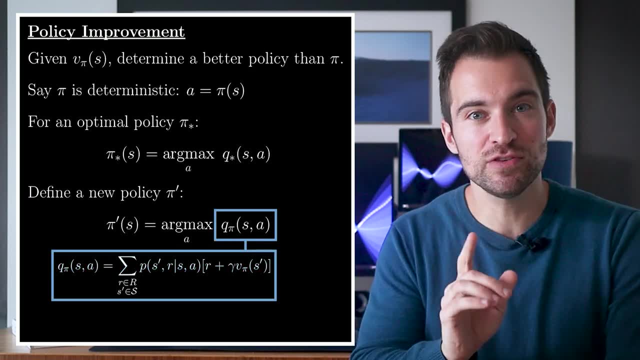 Here's one. We define a new policy which always selects a max action value in every state. As a reminder, we can form the action values like this, using the state values. Also, regarding terminology, we say: the new policy is acting greedily. 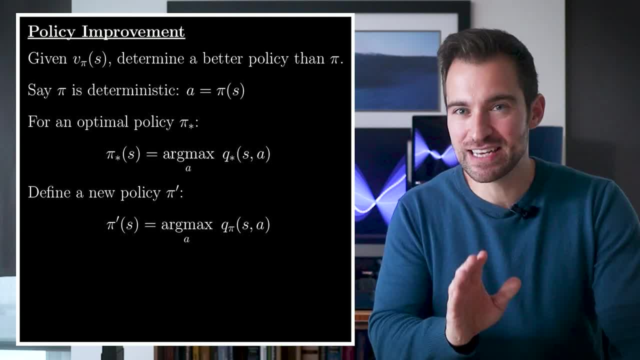 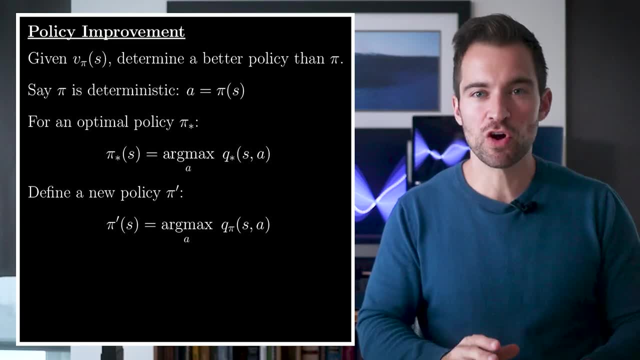 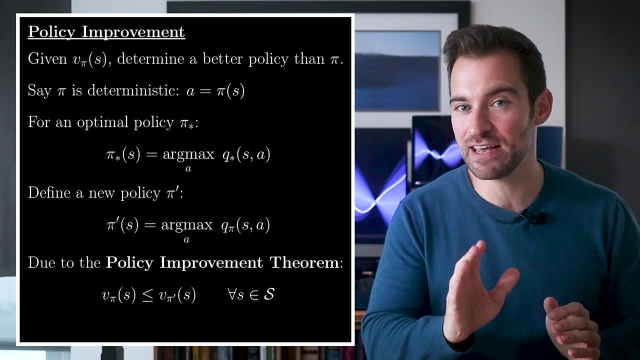 with respect to the value function, since it's akin to a greedy algorithm which uses many local optimizations to travel towards a global optimum. Moving on Because of something called the policy improvement theorem, we are guaranteed that this new policy is at least as good as the policy of the given value function. 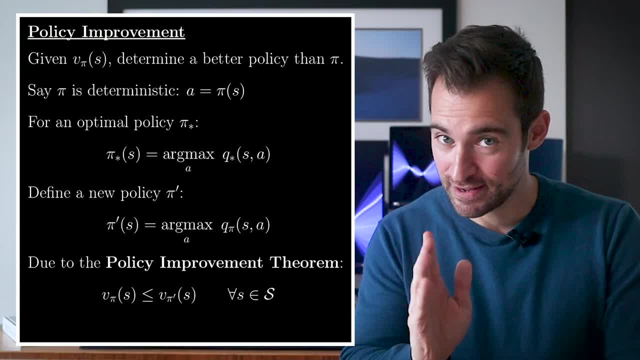 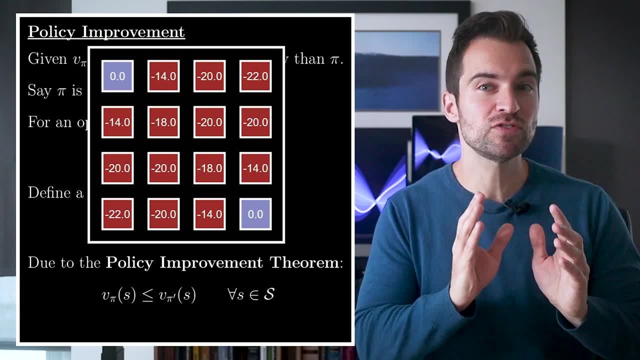 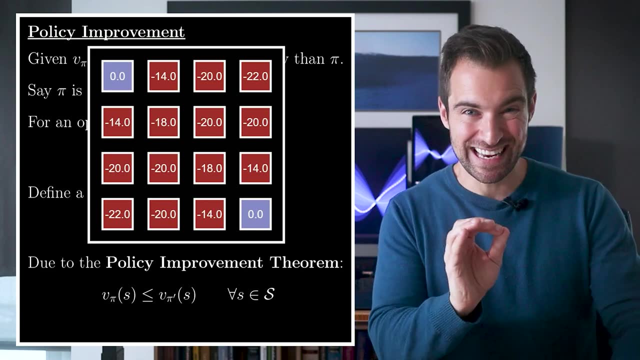 So this always helps And that's great news. As an example, let's revisit the value function from earlier. Remember this: values the policy that gives all actions the same probability. Now applying policy improvement here means our new policy would in each state. 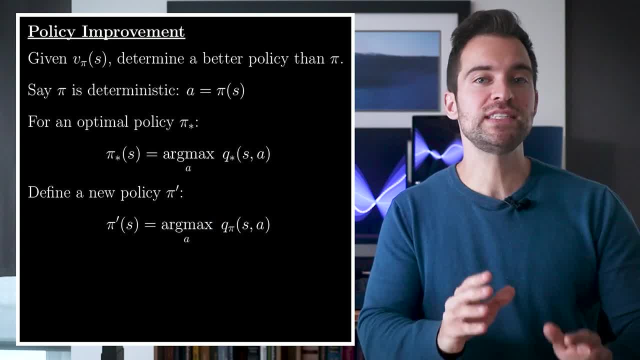 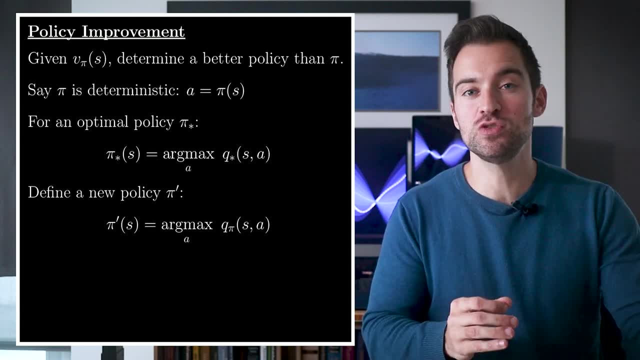 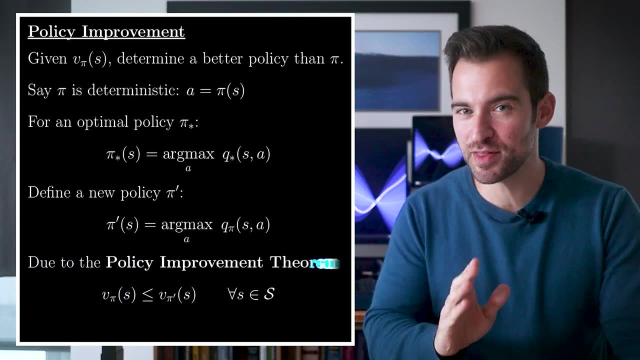 using the state values. Also, regarding terminology, we say the new policy is acting greedily with respect to the value function, since it's akin to a greedy algorithm which uses many local optimizations to travel towards a global optimum, Moving on because of something called the policy improvement. 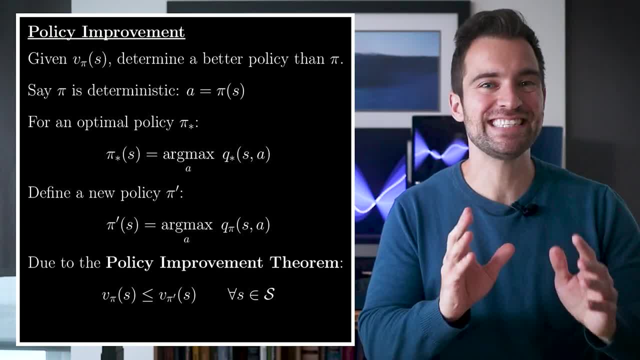 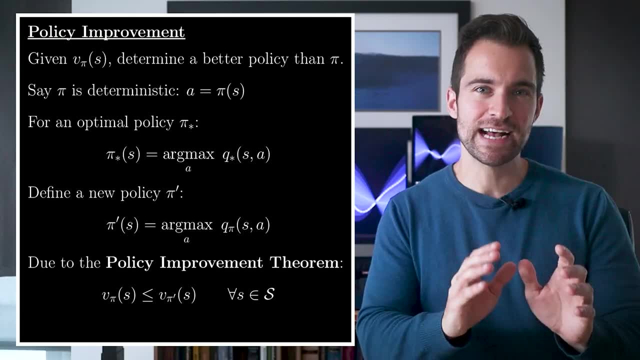 theorem. we are guaranteed that this new policy is as least as good as the policy of the given value function. So this always helps and that's great news. As an example, let's revisit the value function from earlier. Remember this: values the policy that gives all actions. 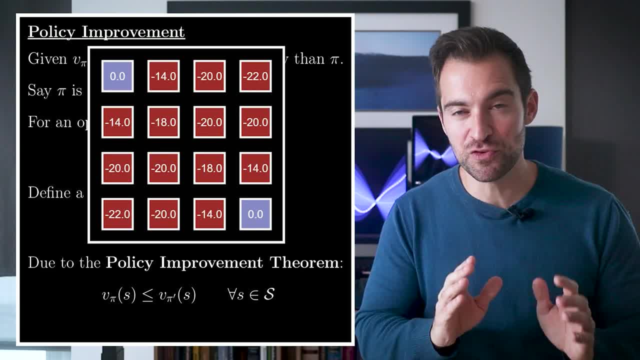 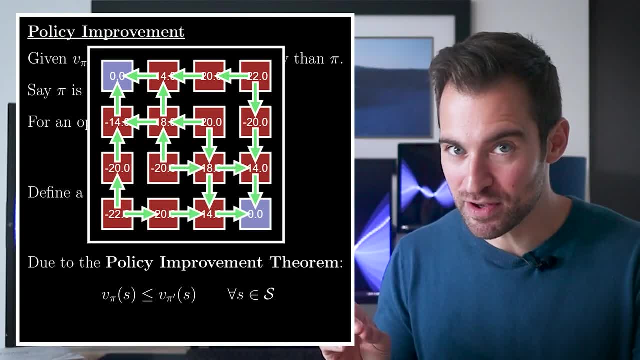 the same probability. Now applying policy improvement here means our new policy would in each state select only the highest action value, And by eyeballing this you can tell this is an optimal policy, Though in general it'll take more than one iteration. 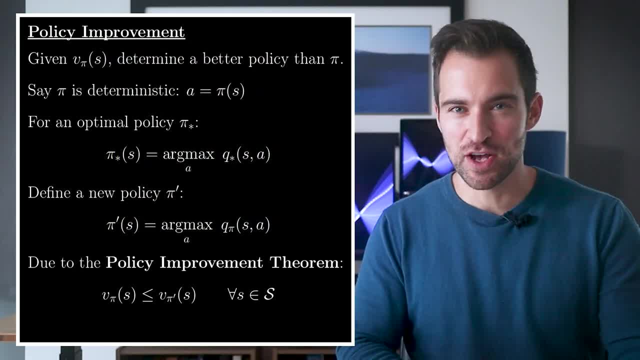 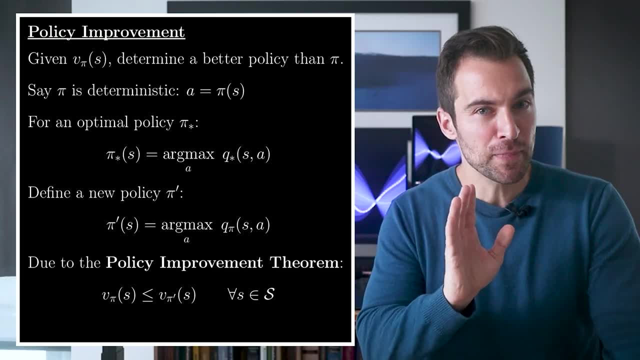 of policy improvement to get to the optimal policy. Now you may ask what if the policy is already greedy with respect to its value function? There would be no improvement to make. Yes, But very interestingly, if you meet that condition where 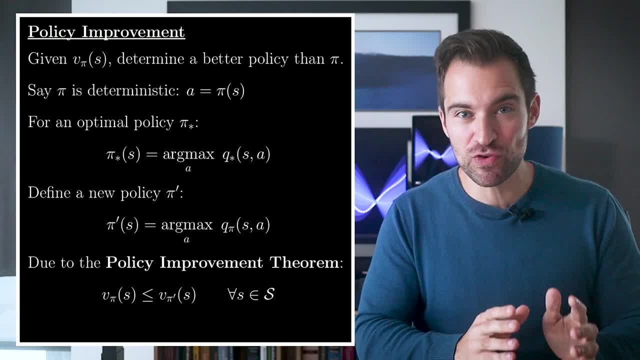 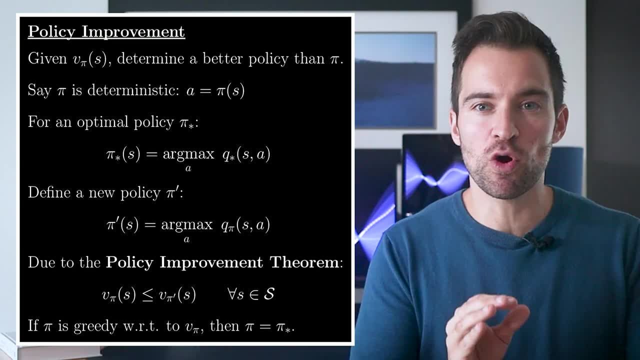 the value function values a policy and that policy is greedy with respect to that value function. you must in fact be at the optimal policy, And that's huge, And that's huge news. It means this tweaking only becomes impossible when there's no more helping to do. 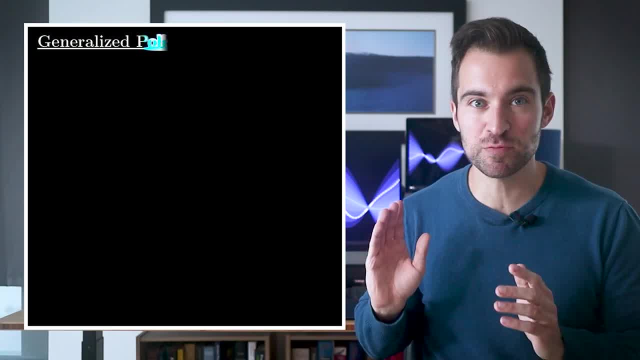 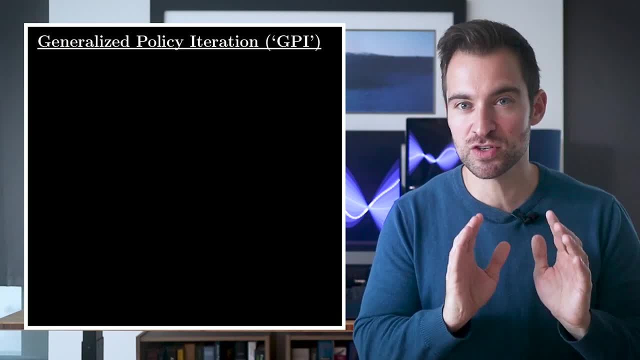 And so this leads us finally to the big picture: generalized policy iteration, or GPI. It refers to an entire class of algorithms, So we'll start with a specific case called, naturally, policy iteration, which will get us the optimal policy and value. 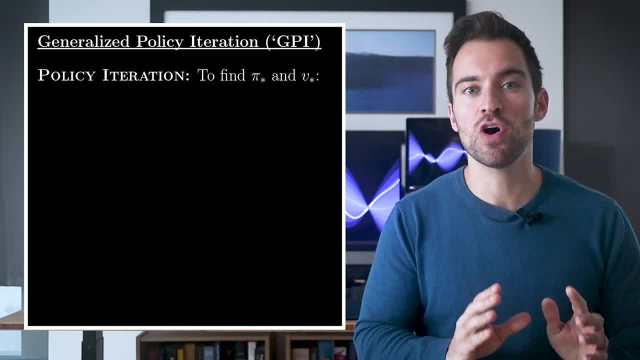 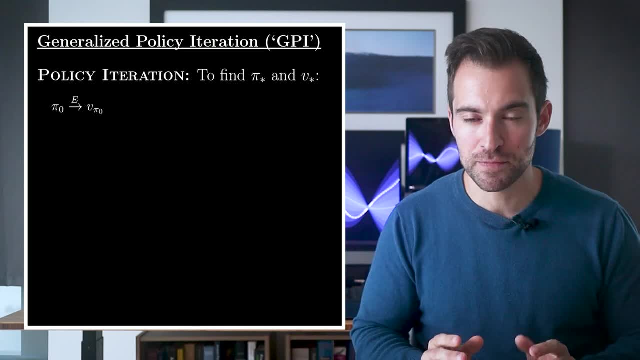 function. It starts with some arbitrarily initialized policy, which we'll call pi 0. We then apply policy evaluation, which means we'll determine its value function. And then we'll apply policy evaluation, which means we'll determine its value function Next, because we know about policy improvement. 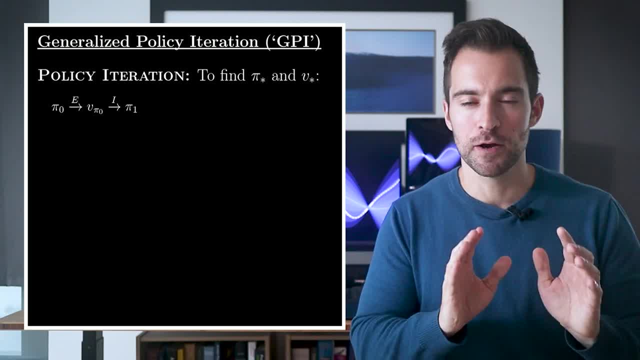 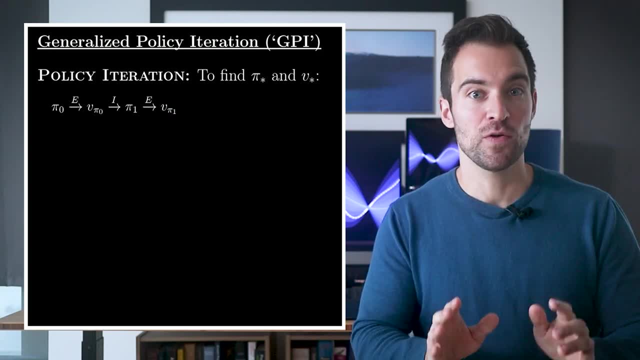 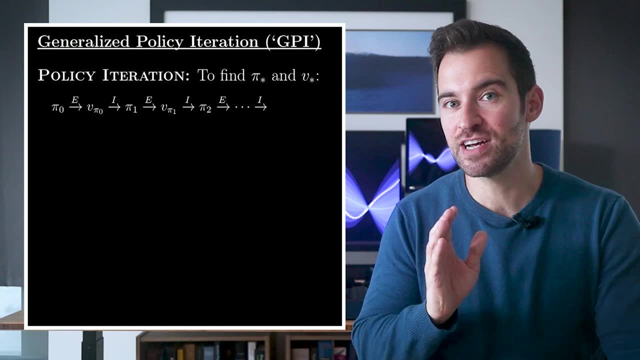 we can create a slightly better policy- pi 1. But now our value function no longer applies. So we apply evaluation again to get a new value function, Then we apply policy improvement to this to yield another better policy, And this process continues until both the policy and the value function stop changing. 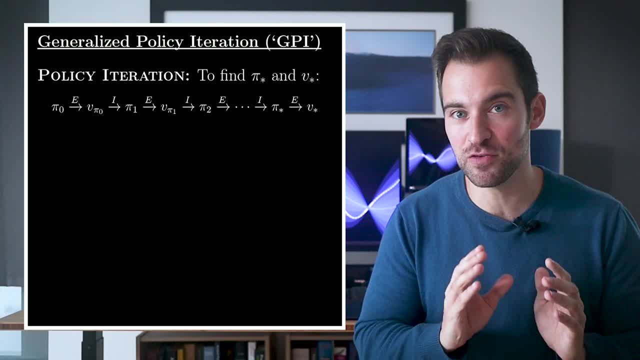 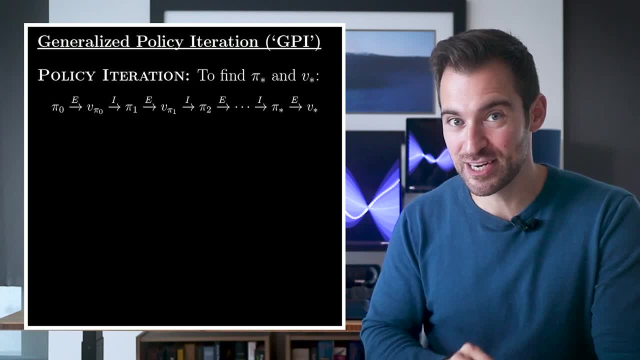 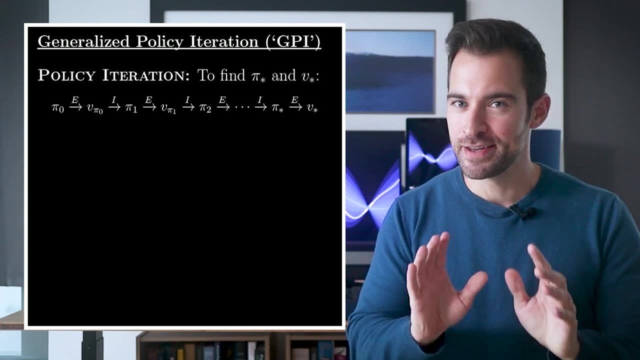 at which point we must have arrived at the optimal policy and value function. Let's appreciate this. It's rare you come across something so simple that does something so useful. Today's a lucky day, OK now. generalized policy iteration refers to something well more general. 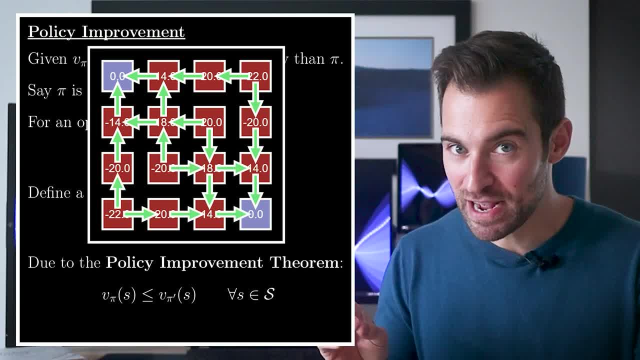 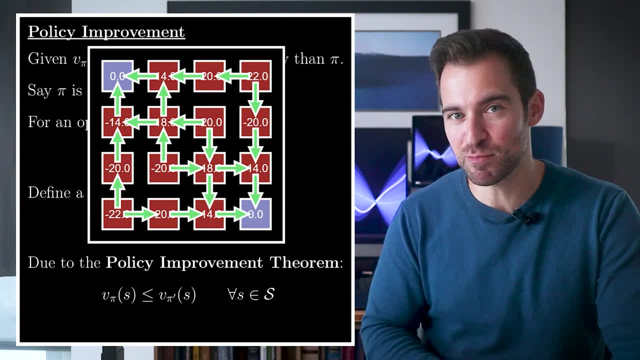 select only the highest action value And by eyeballing this you can tell this is an optimal policy, Though in general it'll take more than one iteration of policy improvement to get to the optimal policy. Now you may ask what if the policy is already greedy with respect to its value function? 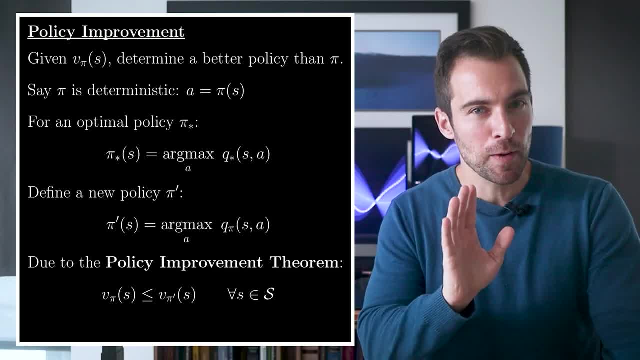 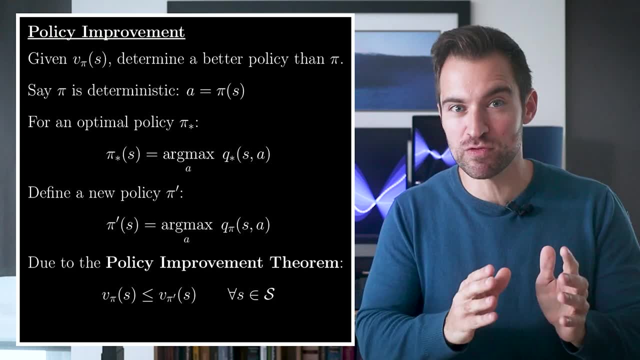 There would be no improvement to make. Yes, But very interestingly, if you meet that condition where the value function values a policy and that policy is greedy with respect to that value function, you must in fact be at the optimal policy. 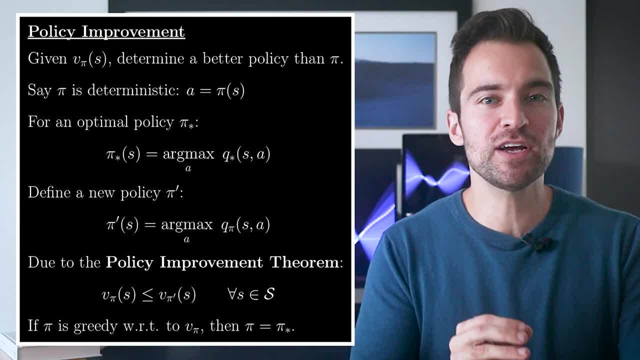 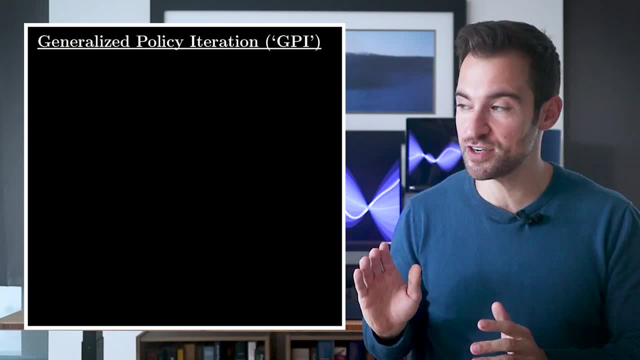 And that's huge news. It means this tweaking only becomes impossible when there's no more helping to do, And so this leads us, finally, to the big picture: Generalized policy iteration, or GPI. It refers to an entire class of algorithms. 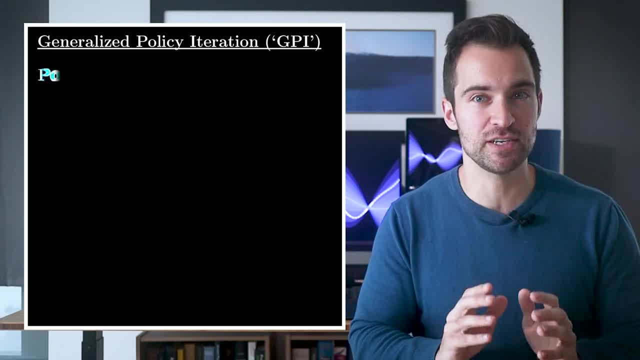 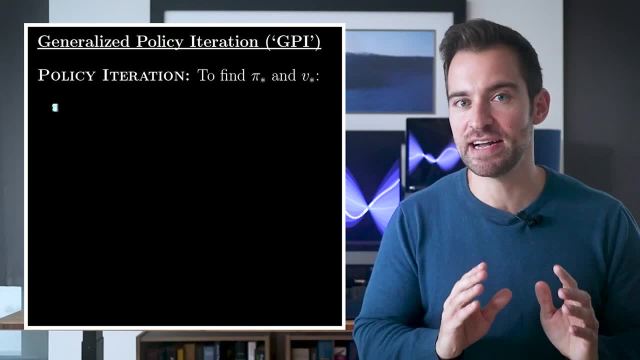 so we'll start with a specific case called naturally policy iteration, which will get us the optimal policy and value function. It starts with some arbitrarily initialized policies, which we'll call pi zero. We then apply policy evaluation, which means we'll determine its value function v, pi zero. 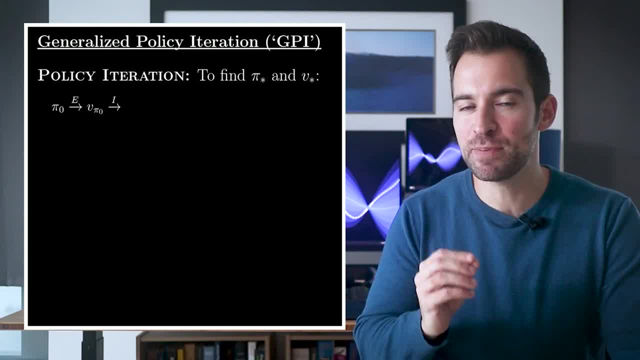 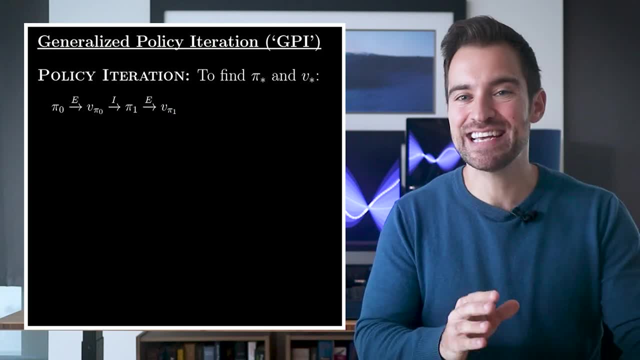 Next, because we know about policy improvement. we can create a slightly better policy- pi one- But now our value function no longer applies. So we apply evaluation again to get a new value function. Then we apply policy improvement to this to yield another better policy. 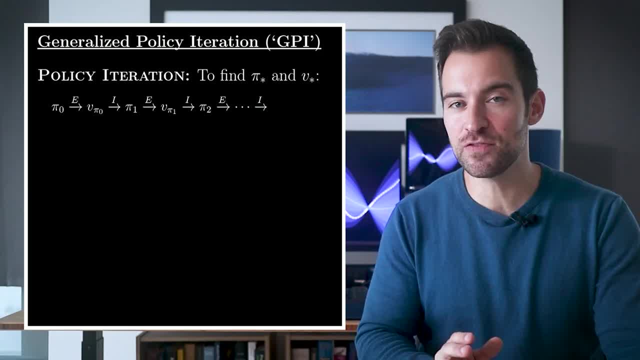 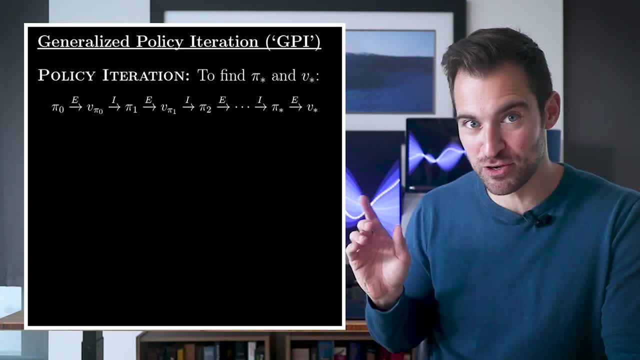 And this process continues until both the policy and the value function stop changing, At which point we must have arrived at the optimal policy and value function. Let's appreciate this. It's rare you come across something so simple that does something so useful. 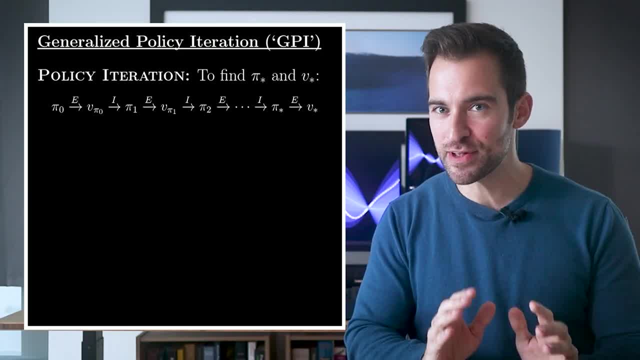 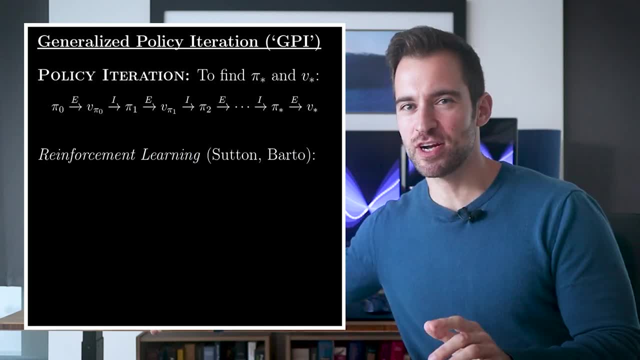 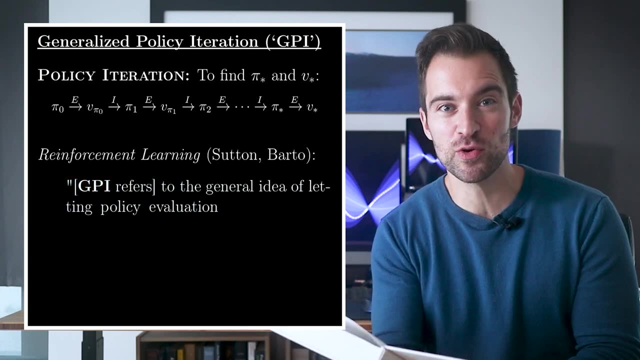 Today's a lucky day. Okay now. generalized policy iteration refers to something well more general. The textbook has a nice description of it, which I'll just read. GPI refers to the general idea of letting policy evaluation and policy improvement processes interact. 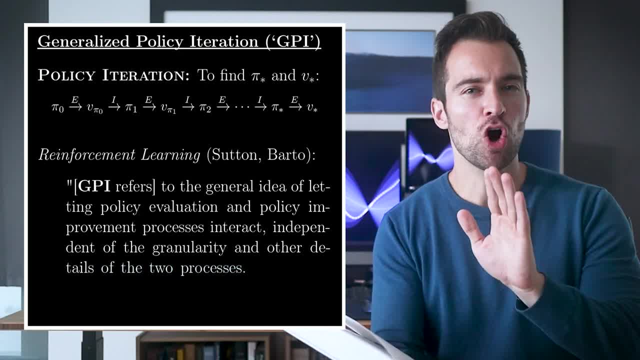 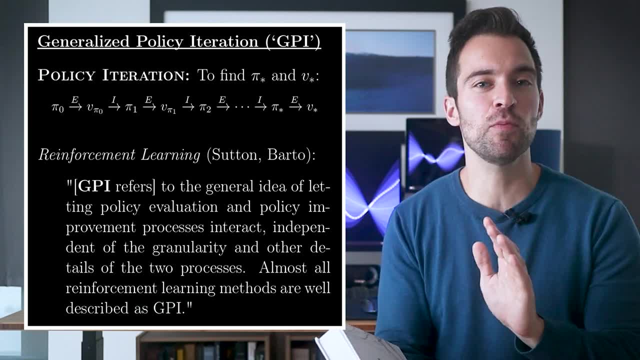 independent of the granularity and the other details of the two processes. Almost all reinforcement learning methods are well described as GPI. I couldn't say it any better than myself. This really captures just how big of a picture GPI really is. To get a sense of the generality, let's imagine adjusting policy iteration. 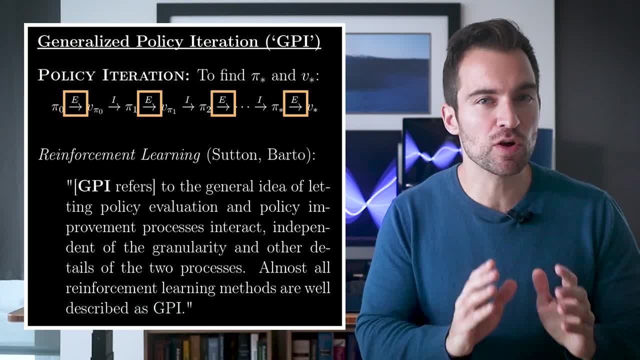 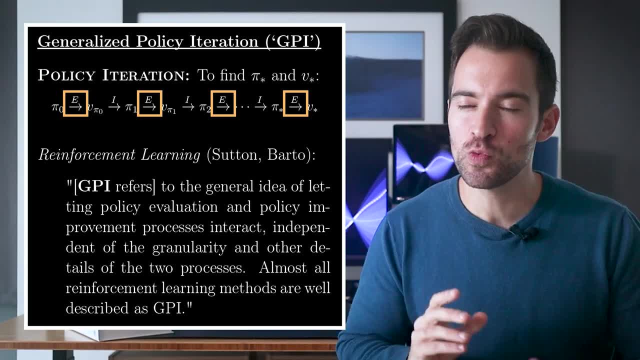 Remember, policy evaluation, as we covered, involves multiple sweeps over the states until the values stop changing. But what if we switch to policy improvement after only one sweep? Would we still converge to the optimum? Yes, and this is in fact called value iteration. 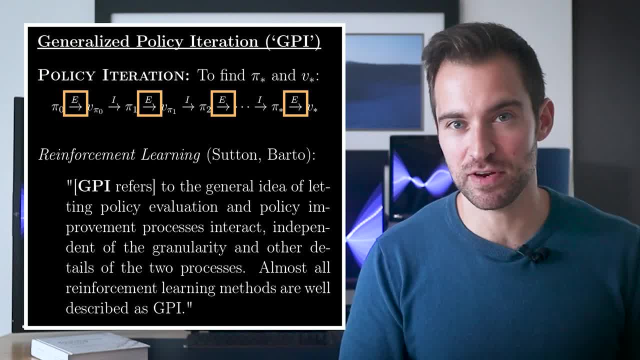 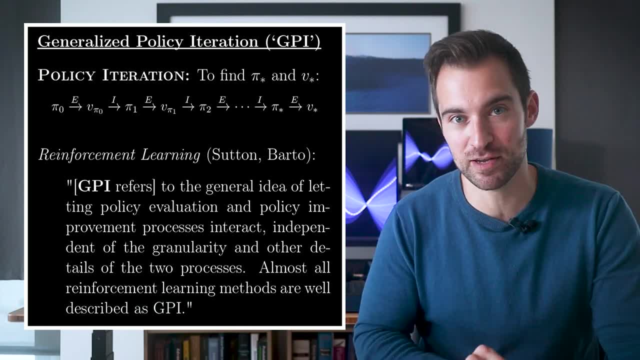 a different algorithm within GPI, which we'll see an example of in a minute. Generally speaking, as long as each process does their job, at least partially, the algorithm will still recover the optimal policy in the limit. As a footnote, the book has this really beautiful way of picturing how these two processes interact. 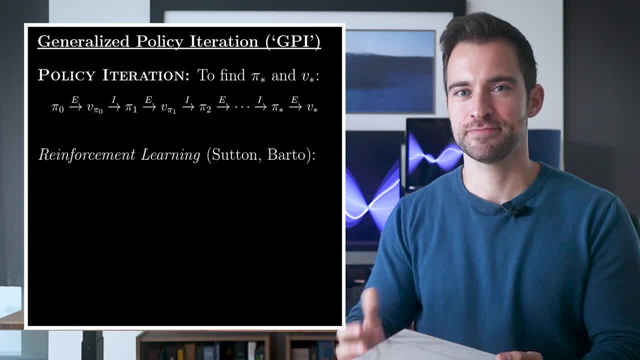 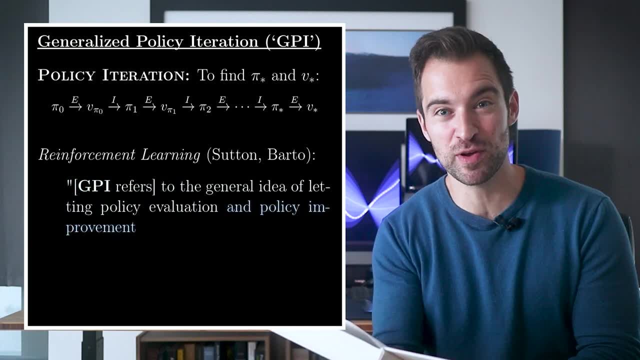 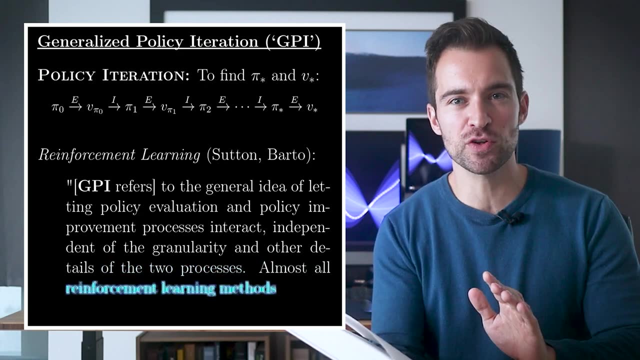 The textbook has a nice description of it, which I'll just read. GPI refers to the general idea of letting policy evaluation and policy improvement processes interact, independent of the granularity and the other details of the two processes. Almost all reinforcement learning methods are well described as GPI. 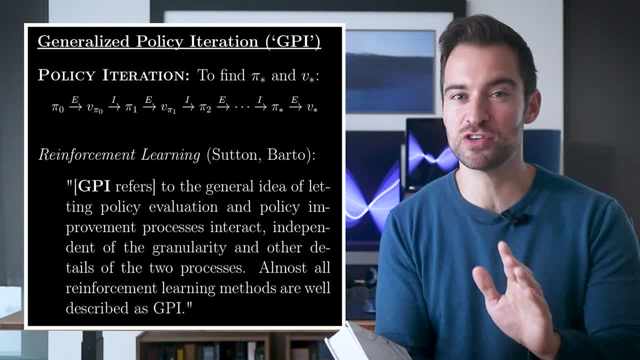 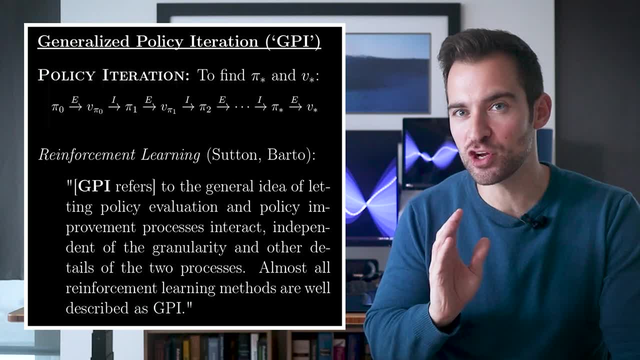 I couldn't say it any better than myself. This really captures just how big of a picture GPI really is. To get a sense of the generality, let's imagine adjusting policy iteration. Remember, policy evaluation, as we covered, involves multiple sweeps over the states. 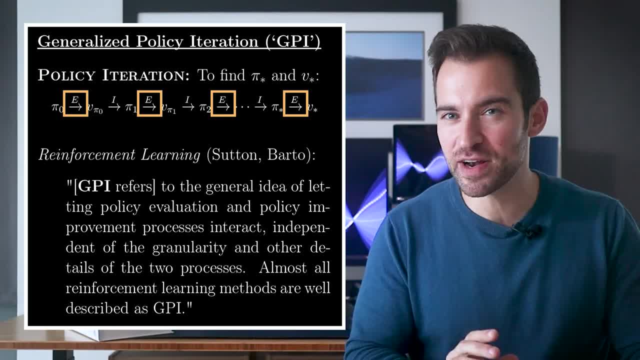 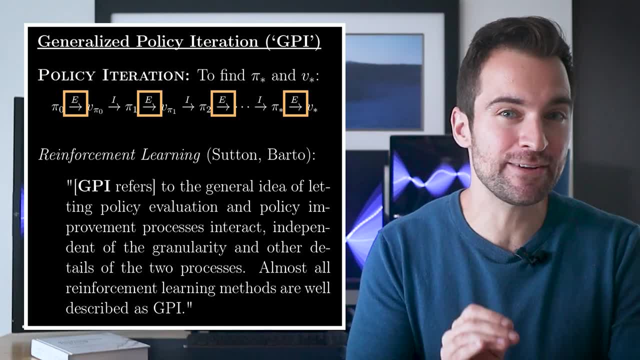 until the values stop changing. But what if we switch to policy improvement after only one sweep? Would we still converge to the optimum? Yes, and this is in fact called value iteration, a different algorithm within GPI, which we'll see in an example. 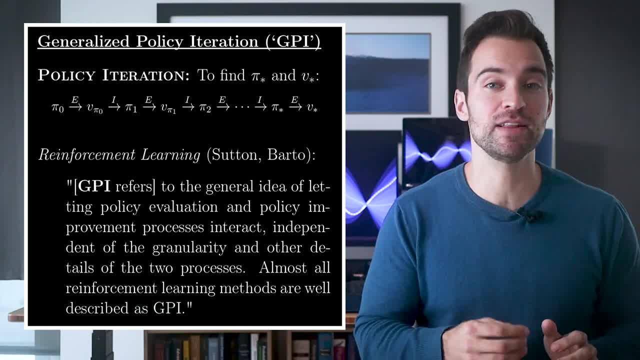 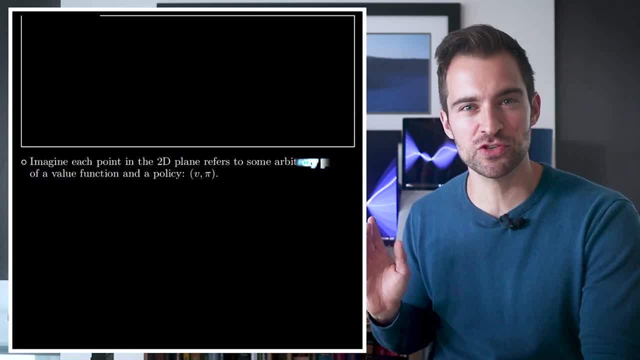 Generally speaking, as long as each process does their job, at least partially, the algorithm will still recover the optimal policy in the limit. As a footnote, the book has this really beautiful way of picturing how these two processes interact. I was going to walk through it. 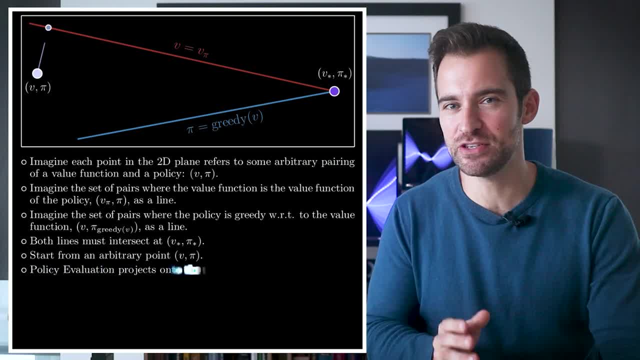 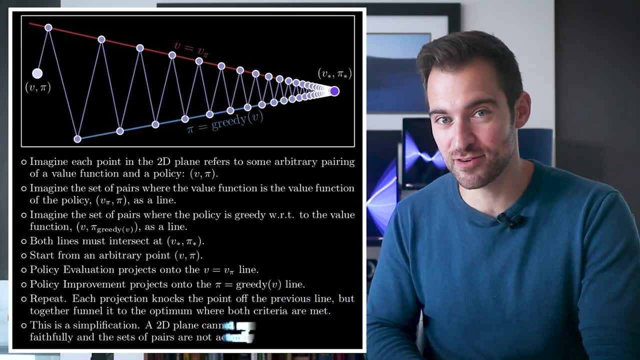 but it's a bit too redundant with what I've already covered and rather heavy to explain. I'm including it here because I just don't have the heart to cut it, So feel free to mute me and pause your way through this if you're interested. 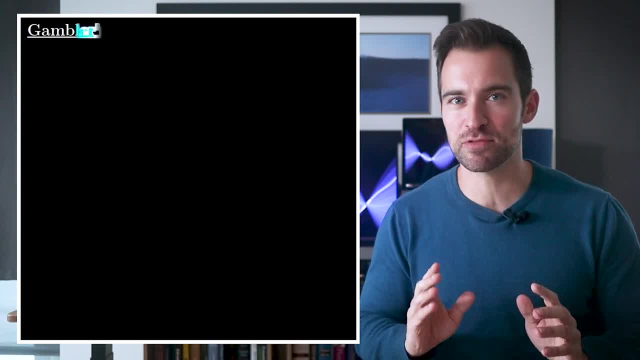 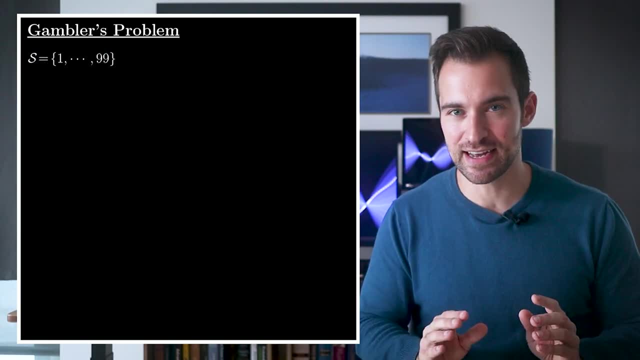 Okay, now let's do the value iteration example. This is the gambler's problem. This is the gambler's problem from the book. Here's the setup: The gambler's state is his capital, which is an integer between 1 and 99.. 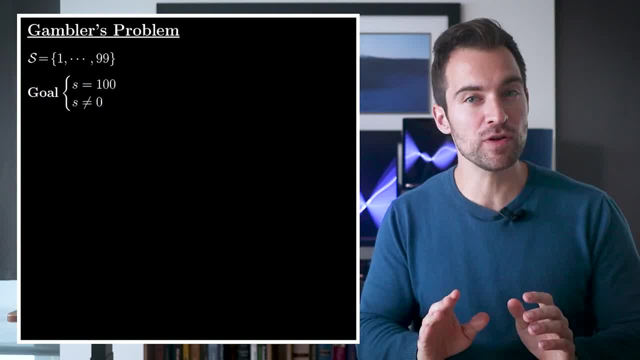 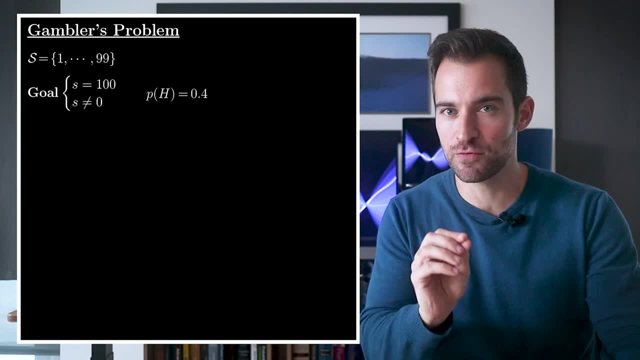 His goal is to reach the terminal state of $100 before the terminal state of $0.. To achieve the goal, he can repeatedly bet on an inbounds coin which has a probability of heads of 40%. Specifically, he can bet an integer up to the amount he has. 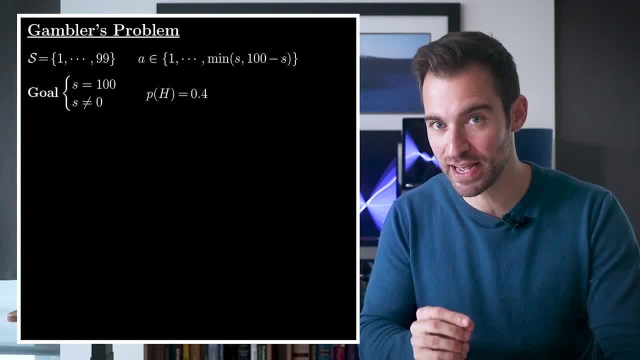 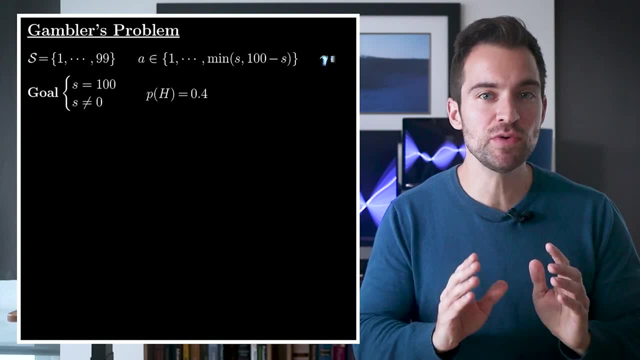 or the difference to $100.. If the coin comes up heads, he gains as much as he bet. Otherwise he loses it. This can be encoded as an MDP by applying no discounting and saying all rewards are 0, except there. 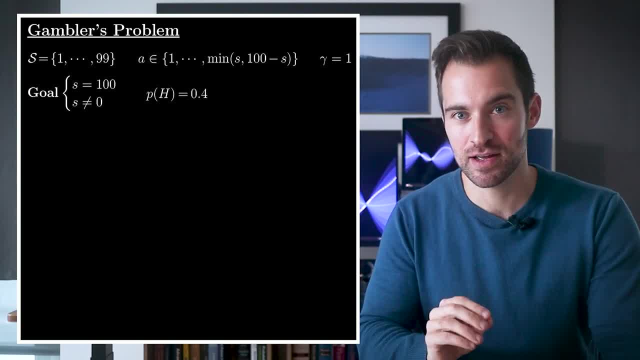 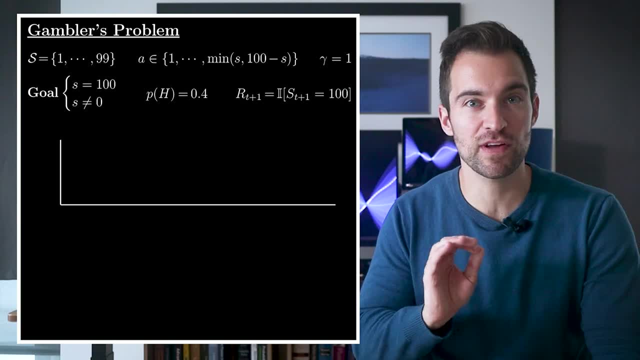 is a reward of 1 when transitioning to the state of $100.. This can all be expressed with an indicator function like this: To visualize the solution, we'll start with a plot of our value function, where we have the state across the horizontal axis. 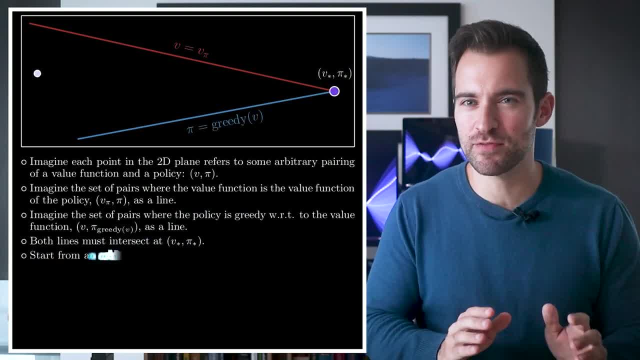 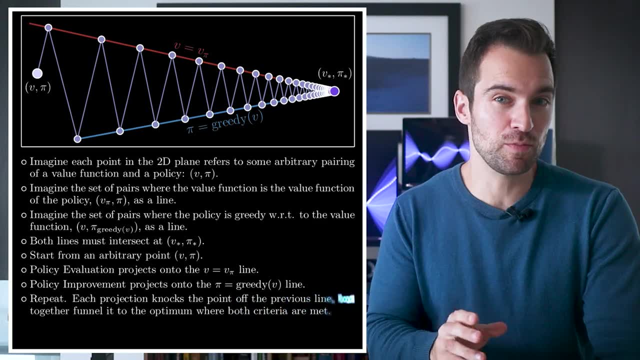 I was going to walk through it, but it's a bit too redundant with what I've already covered and rather heavy to explain. I'm including it here because I just don't have the heart to cut it, So feel free to mute me and pause your way through this if you're interested. 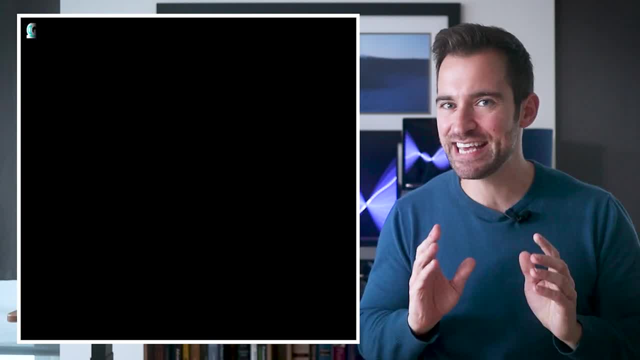 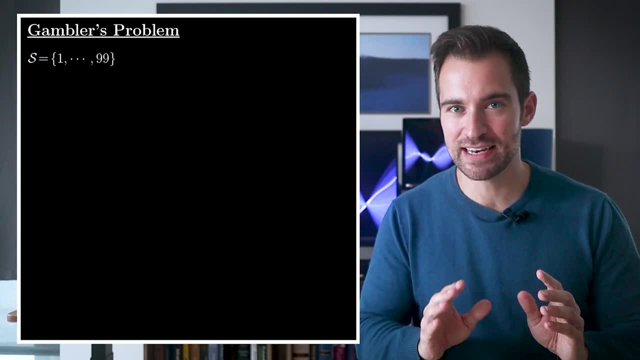 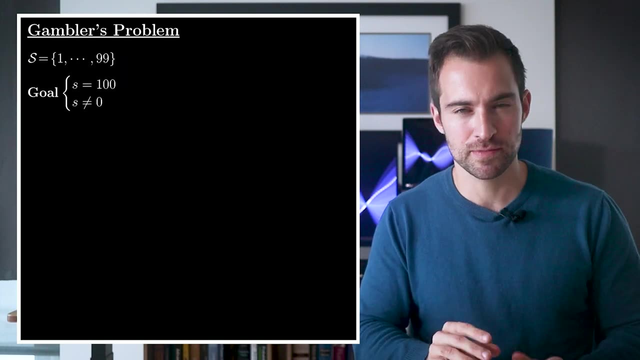 Okay, now let's do the value iteration example. This is the gambler's problem from the book. Here's the setup: The gambler's state is his capital, which is an integer between 1 and 99.. His goal is to reach the terminal state of $100 before the terminal state of $0.. 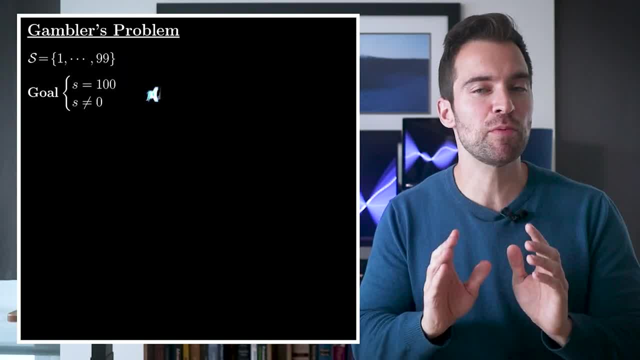 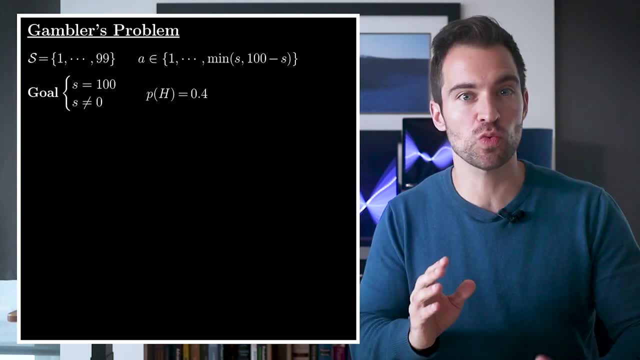 To achieve the goal, he can repeatedly bet on an inbounds coin which has a probability of heads of 40%. Specifically, he can bet an integer up to the amount he has or the difference to $100.. If the coin comes up heads, he gains as much as he bet. 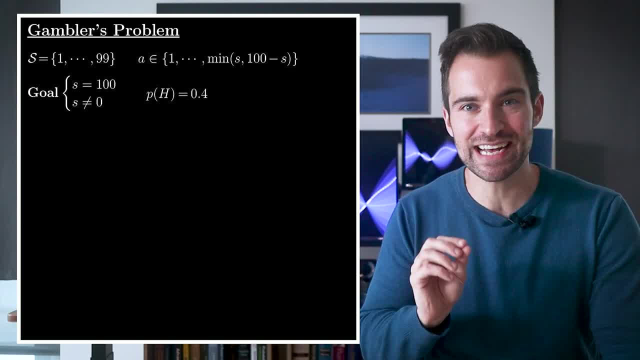 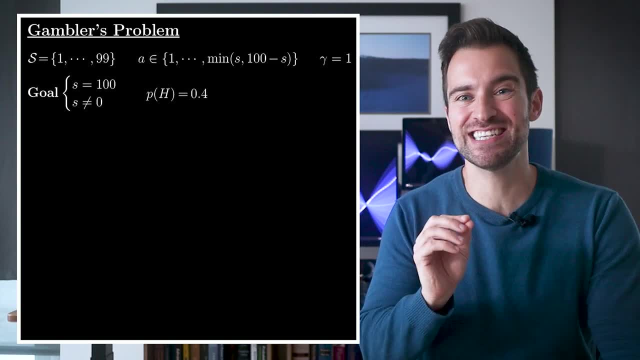 Otherwise he loses it. This can be encoded as an MDP by applying no discounting and saying all rewards are 0, except there is a reward of 1 when transitioning to the state of $100.. This can all be expressed with an indicator function like this: 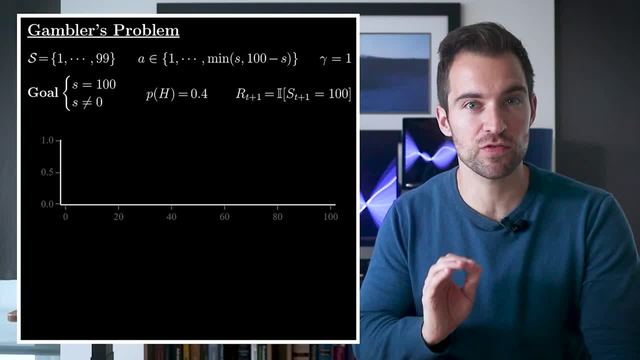 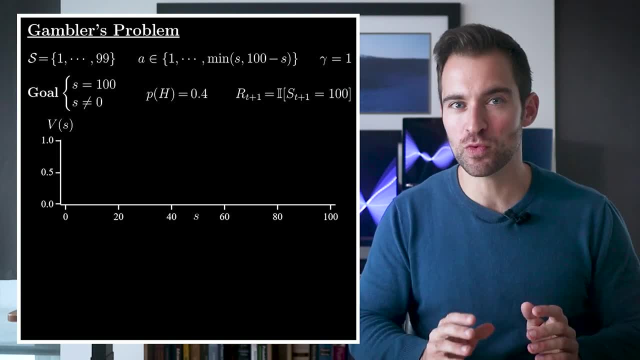 To visualize the solution, we'll start with a plot of our value function where we have the state across the board, the horizontal axis, and the value along the vertical axis. Second, we'll have a similar plot, except the vertical axis gives us the policy's bet amount in each state. 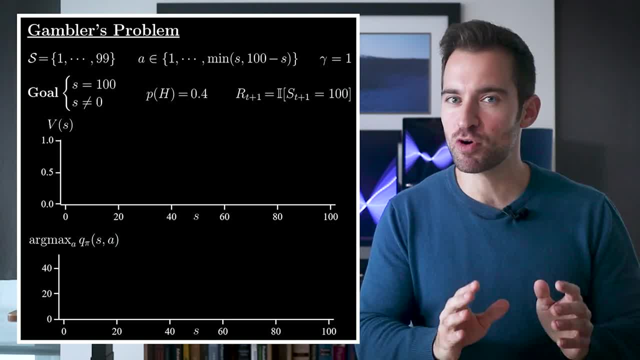 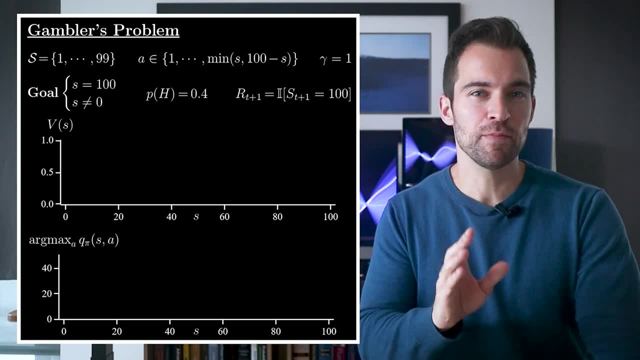 which, in this case, is deterministic. Since this problem will give us quite a bit of ties among highest action values, we'll break those ties by always selecting the smallest bet. Okay, we start by initializing the value function to 0.. Doesn't have to be that, but it works. 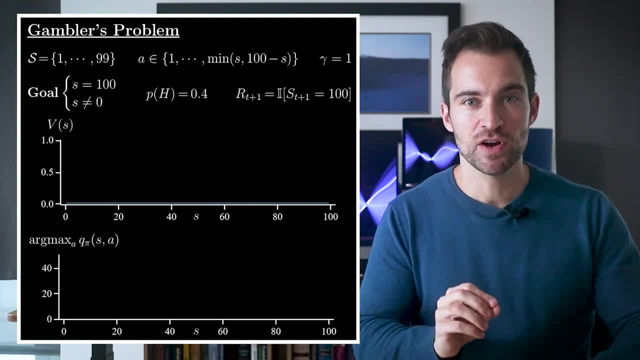 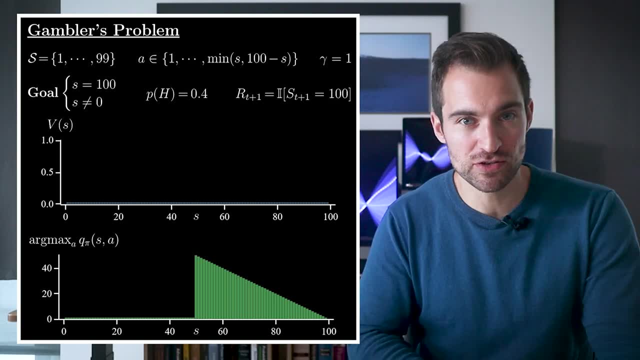 From here we do our first iteration of policy improvement, which gives us these bets. This policy says once over 50, bet whatever it takes to get to 100.. Now we ask: what value does this policy imply for each state? 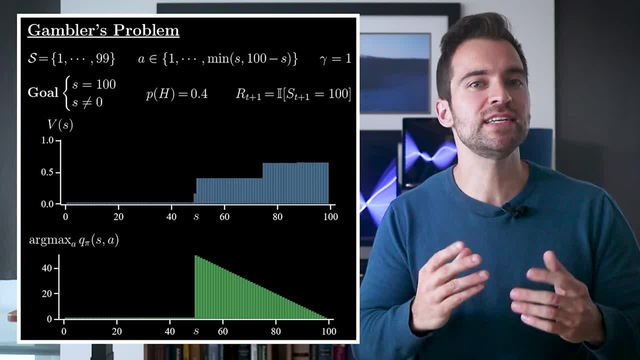 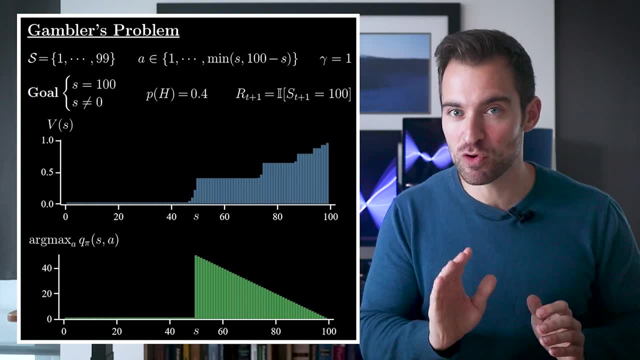 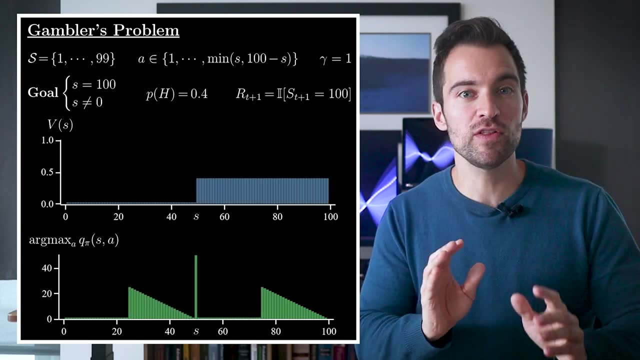 Well, if we're doing policy iteration, we would continually sweep over the states until the value function stopped changing. But, as we mentioned, that's not required In value iteration. we only do one sweep Before making the policy greedy with respect to this value function. 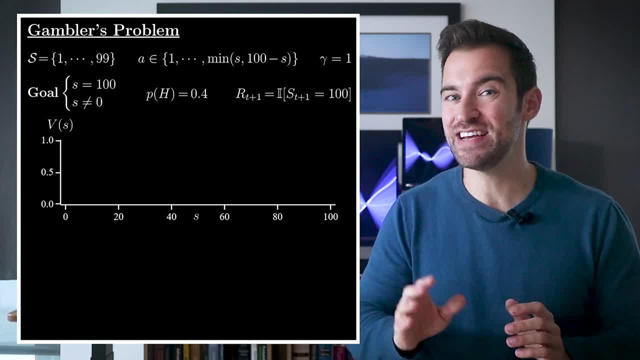 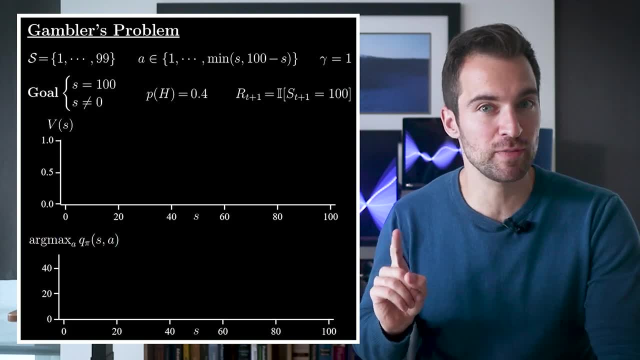 and the value along the vertical axis. Second, we'll have a similar plot, except the vertical axis gives us the policy value And the vertical axis gives us the policy's bet amount in each state, which, in this case, is deterministic. Since this problem will give us quite a bit of ties, 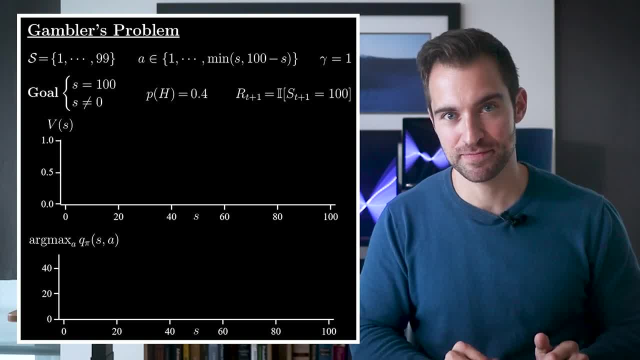 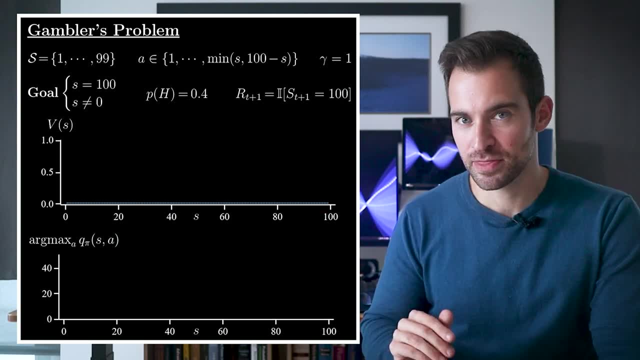 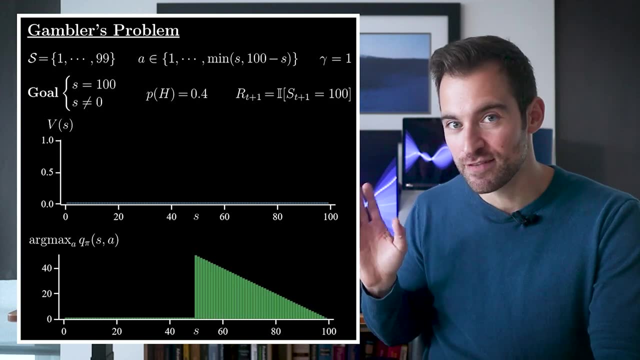 among highest action values. we'll break those ties by always selecting the smallest bet. OK, we start by initializing the value function to 0. Doesn't have to be that, but it works. From here we do our first iteration of policy improvement, which gives us these bets. 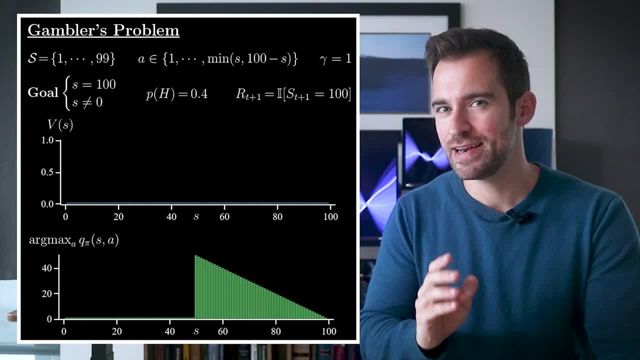 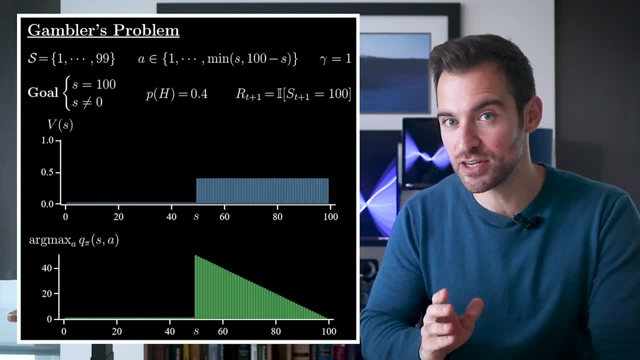 This policy says: once over 50, bet whatever it takes to get to 100.. Now we ask: what value does this policy imply for each state? Well, if we're doing policy iteration, we would continually sweep over the states until the value function stopped changing. 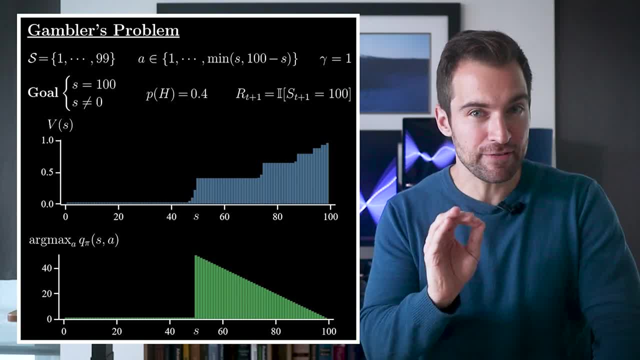 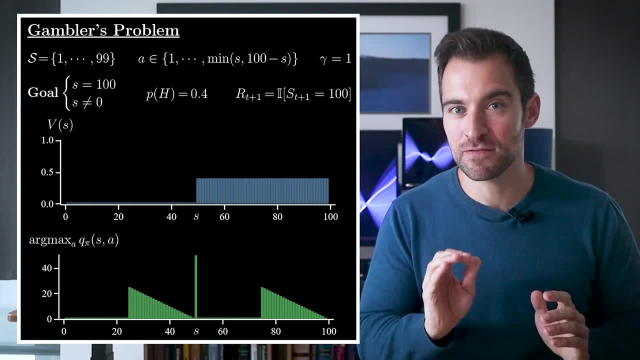 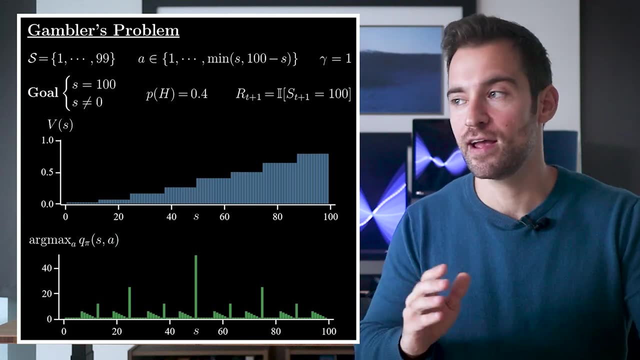 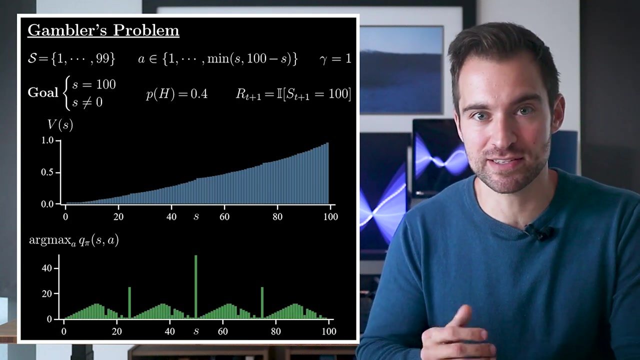 But, as we mentioned, that's not required In value iteration. we only do one sweep before making the policy greedy with respect to this value function, And this process iterates back and forth, and back and forth, and back and forth until the process stops changing and we have the optimal policy. 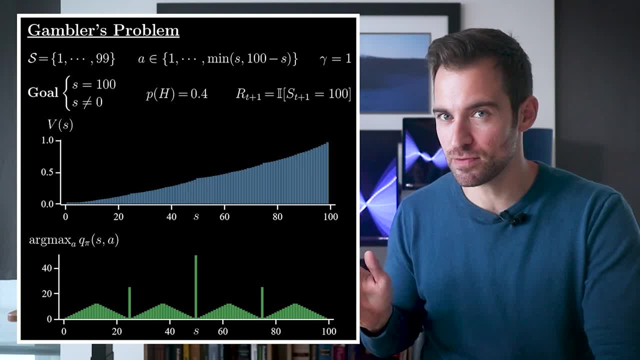 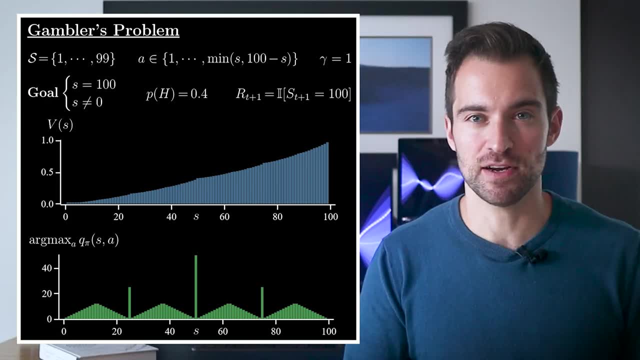 And, as you'll notice, the optimal policy looks interesting and unusual, And that's part of the beauty. I'm sure some clever analysis of this problem would uncover this strategy, But dynamic programming makes that unnecessary. With a simple general algorithm you get whatever optimal strategy the problem demands. 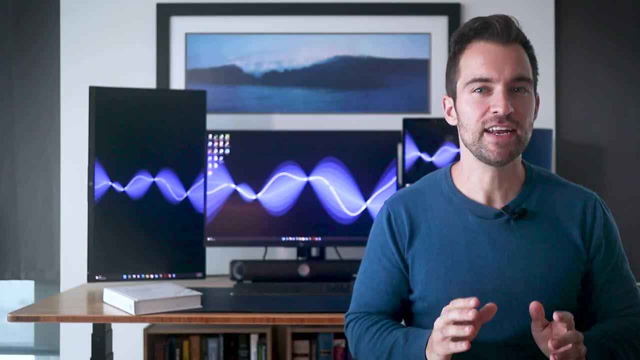 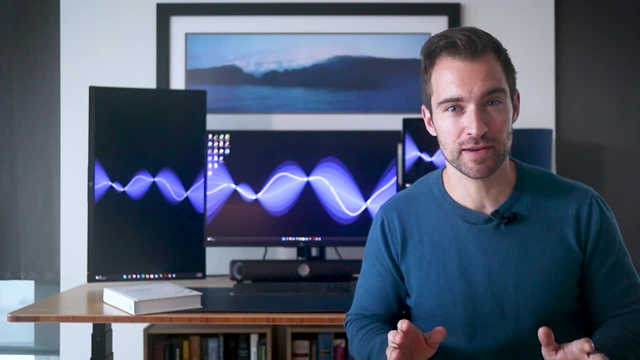 So this is a very powerful tool, but its power is limited. To get here, we required perfect knowledge of the environment, And I didn't go into detail about this. but the state space is also limited. It can't be too big. 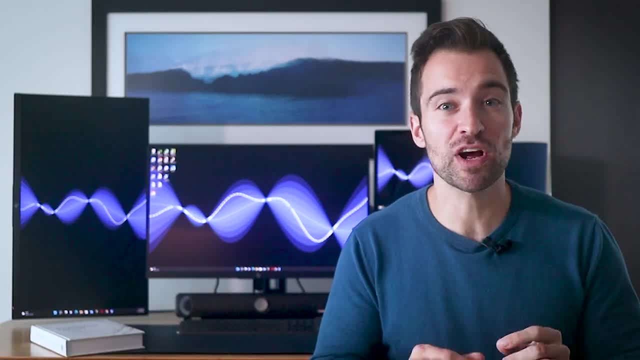 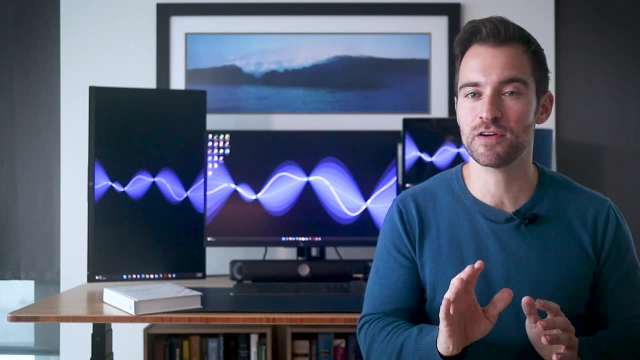 Nonetheless, the theory is foundational to RL As real world problems. strip away these cushy assumptions. we can address those holes directly and still make good progress. To see that, you'll need to watch the next video on Monte Carlo methods for RL. 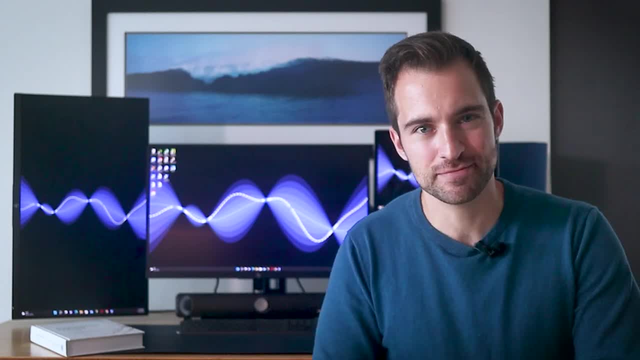 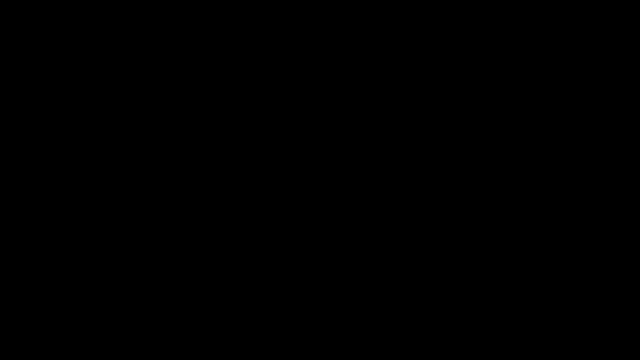 Don't be soft, be tough and keep focusing. See you there. Thanks for watching.